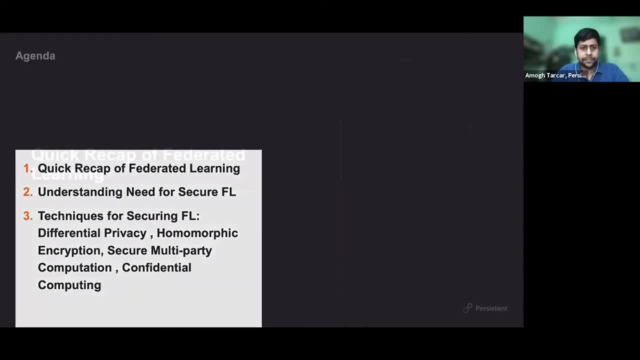 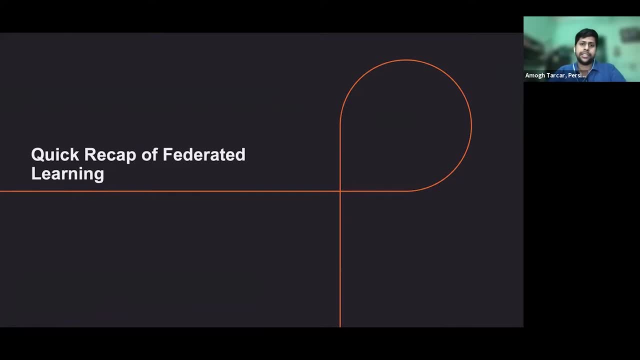 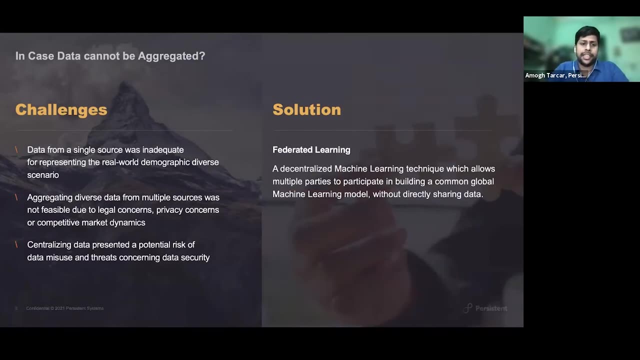 how do we go about securing federated learning? So the last session was about introducing the concept of federated learning and trying to understand its applications. So today let's just quickly try to see why we thought of federated learning. So we are aware of challenges in aggregating data, So there could be multiple. 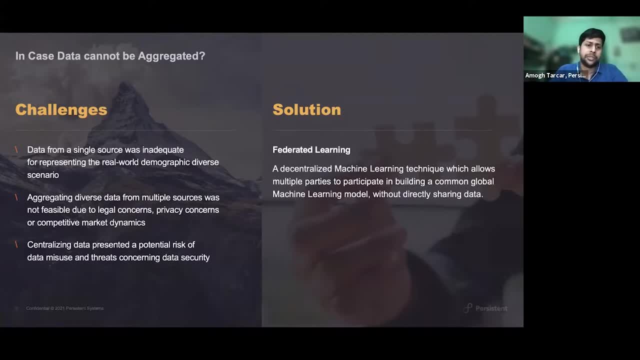 reasons why data cannot be all aggregated in a central server. It could be because of that particular data set up, it could be because of the particular model, or it could be because of the particular data set up Even in a particular model. let's just say, for if you are doing a, 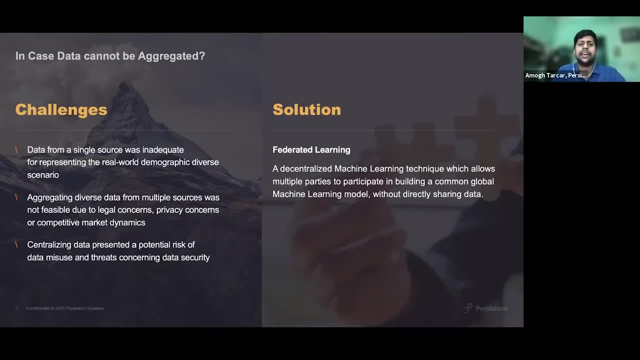 healthcare model and you really want data which has to represent a large group of people And suppose, especially if it's a rare disease, then it's often unlikely that all the data will be accumulated in one hospital, So you need to get data from multiple hospitals, multiple regions, all. 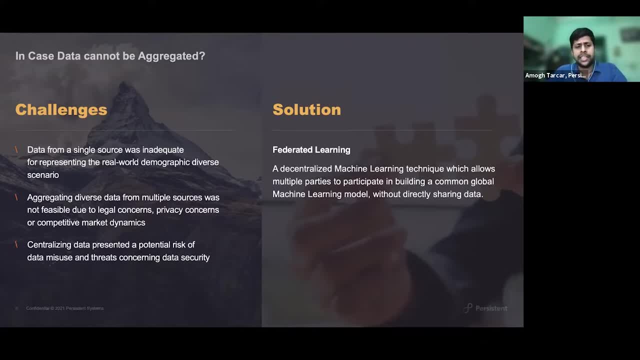 around the world, and that itself is a very difficult challenge. And from the same side, another way of looking at it is that you want realistic data to represent the data set up in a central server, So world, and that is not often present in one location, so you usually have data siloed across. 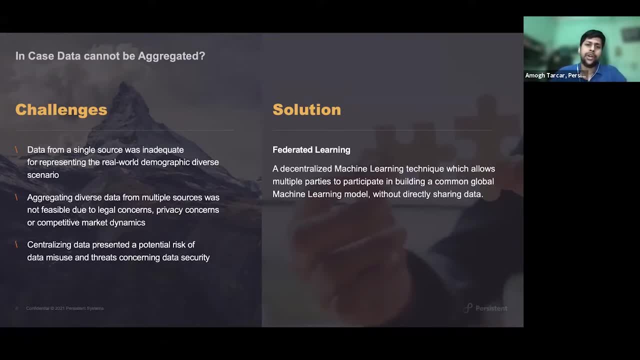 multiple uh either uh in inside the organization, but in various regions, on various organ and sub organizations, or it could be between competitors and so on. second is, when we aggregate so much data, we have to uh kind of make sure that you know we are. we are not uh running afoul of any legal 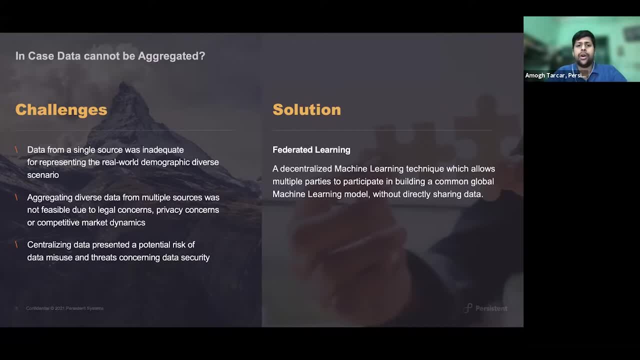 concerns and we have to also consider the privacy of the of the data custodian, and also we need to understand that when we put it all together in a central place, that could be like, because it's all put together in one central place, uh, it becomes a very sort of a target where adversaries 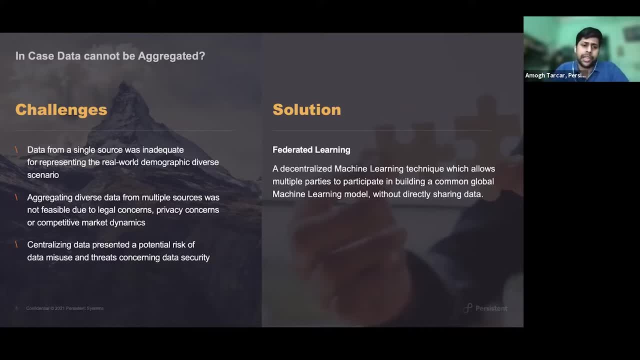 can really attack and try to get- uh, try to get- information out. so that could basically be leading to some sort of misuse of data or, you know, we have to also take care of data security. so a solution around that is basically, you know, instead of aggregating all the data and worrying. 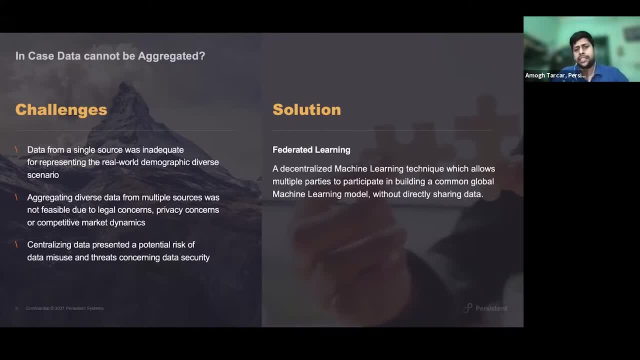 about all these security things? why not keep the data where it originates, at its source, and still do federated learning? so that's basically the concept of federated learning, which is decentralized machine learning which allows you to learn across multiple locations, but you do it in a decentralized. 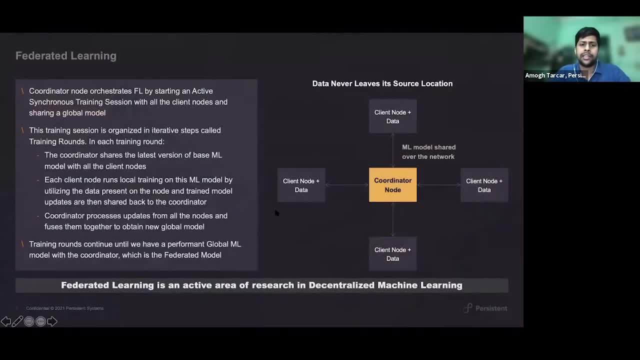 way. so, without sharing the data directly, you can still train machine learning models by actually using uh sort of a star network or other topologies which are there, wherein the model actually travels to the client modes where the data lives, learns there, and then all these updates have to. 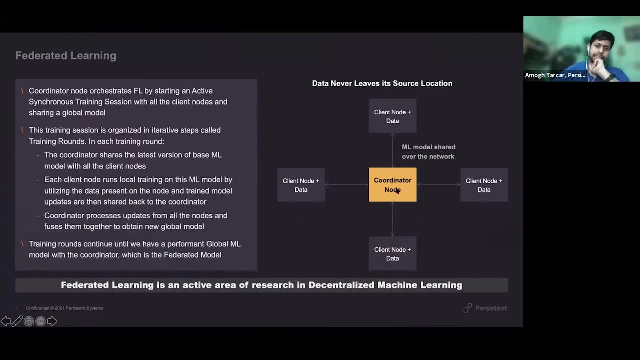 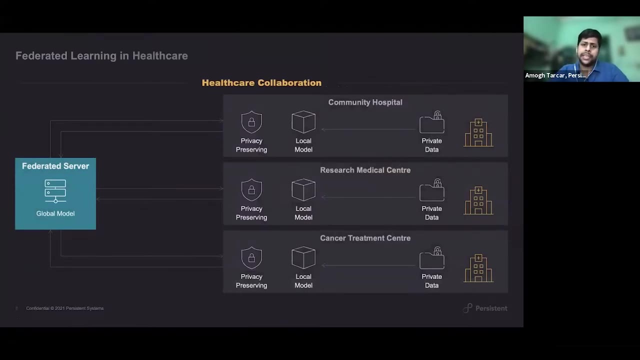 be fused together, uh, to obtain your new, new model, and uh. so in the last session, we actually uh discussed about this at length and we tried to understand how exactly credited learning works. so, uh, this is one diagram which i'll refer to, uh as we as we progress in this session today, wherein 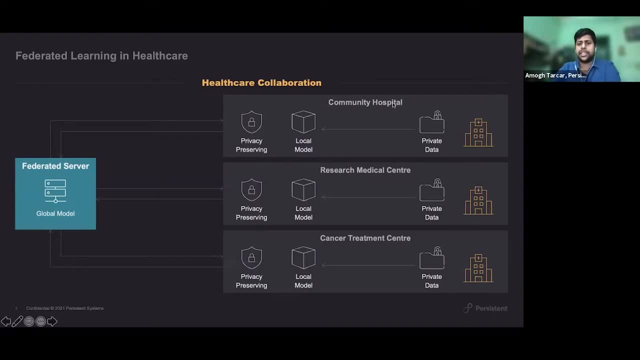 we have this local model across like. so there are three. i suppose there are three data locations, uh, of healthcare models. say, one is a community hospital, another is a research medical center and third is a cancer treatment center, and uh, each of these have some private data on which. 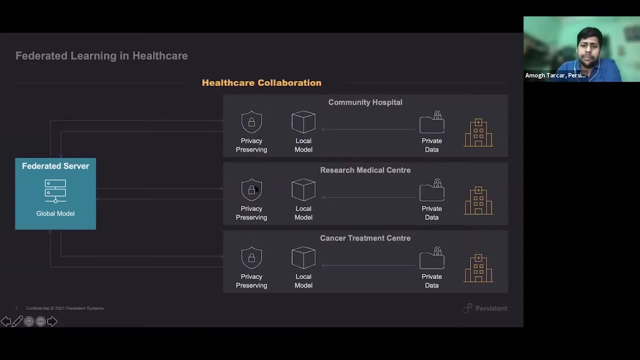 we want to actually learn machine learning, and each of them will receive this edited model, they'll train their own local model and then they'll send it back, and so on. but let's try to understand how privacy preserving and what exactly does this shield? what sort of technologies can be actually employed to make this shield so? uh, so far we as in, i guess. 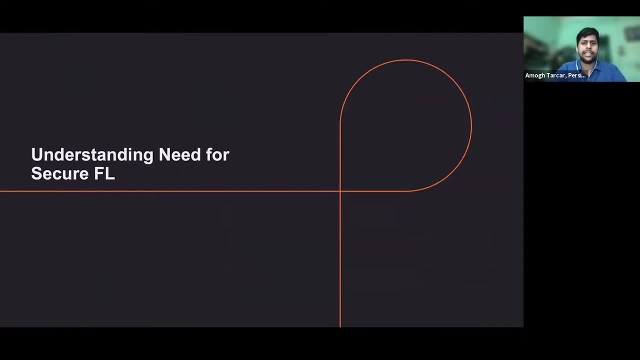 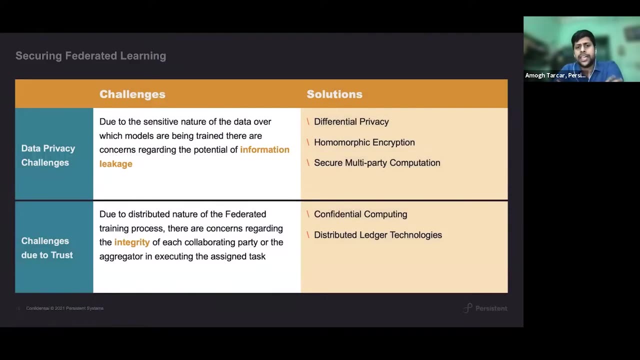 it's just a recap of what we had uh studied last time. uh, we can actually go and try to understand why secure federated learning. so there are, like very, at a very broad level, there are these two challenges which can come up right. first thing is that, uh, we need to think about 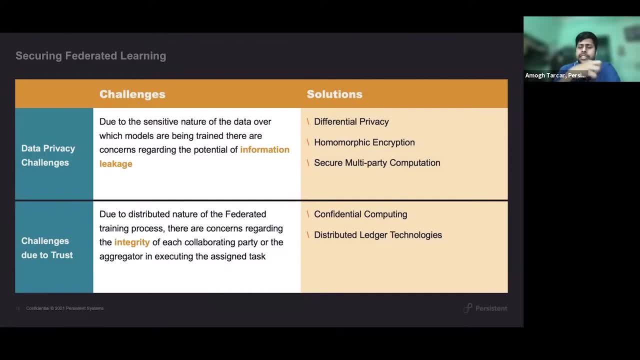 you know, data is not directly getting uh, like it is, it's not moving from its place. so definitely, data is safe. but because we are building models over the sensitive data, we need to be careful about what sort of data can leak from the learned model. so now we are basically abstracting from that data to what exactly can? 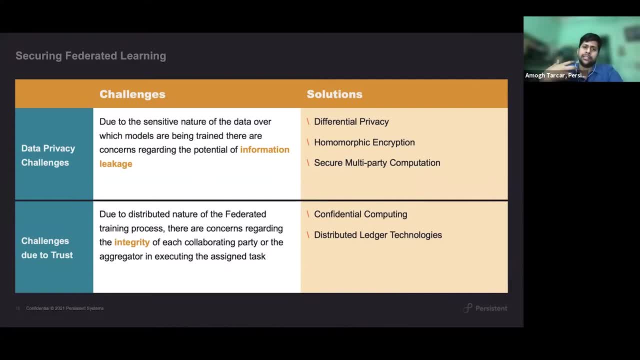 leak by interrogating that learned model. can you, can you? what can you really infer from those weights and the data that we are getting transferred to the segregator? so there are concerns regarding information leakage and this. this is not direct, it's not row by row, but it's still uh. 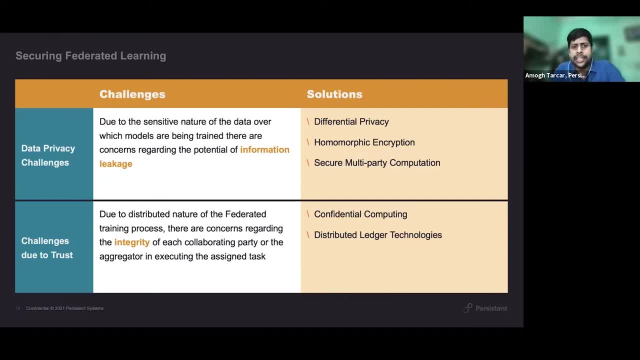 sensitive area because, uh, the data itself on which we are trying to train this is sensitive and upfront solutions around information, you know. you know, to protect information leakages are, uh, things like differential privacy, homomorphic encryptions and multi-party complications, and we'll we'll take a look at that in the next slide. 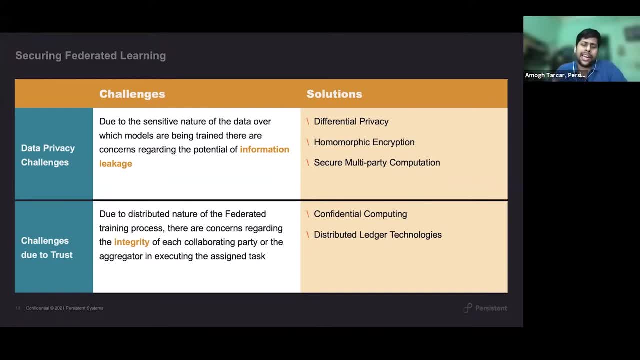 a deep dive on it in this session. but that's one broad category in which you know why you have to really think about securing federated learning, because by default, federated learning is just a learning protocol and it has a very nice virtue that data is not moving from its source location. 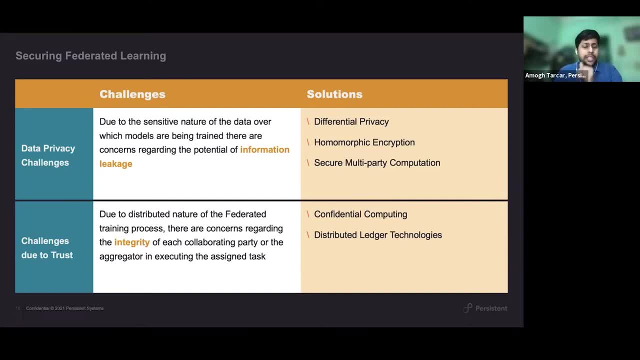 so we get data privacy kind of for sure. but then you're still: what exactly can be learned from this model? that is a very interesting study and we'll take- uh, we'll basically try to understand that more in a very brief way. uh, so the first set of challenge actually arrives from the collaborative nature of 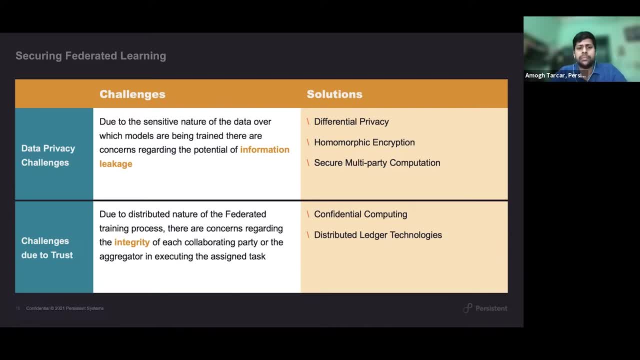 federated learning. so federated learning is not possible with just a single party. as such, you have to have multiple parties. now, in case you, you switch over from a scenario wherein all the parties are really, you know, trusting each other and the aggregator is also very, very trusted. 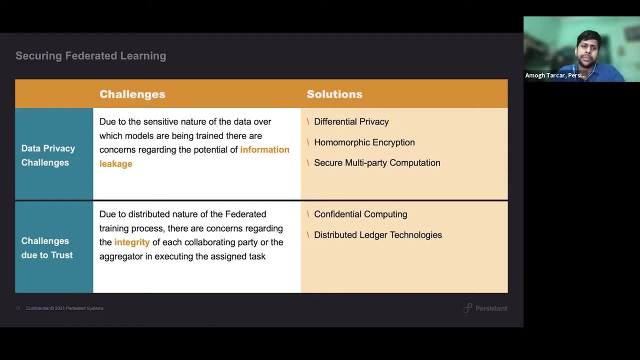 in those scenarios these kind of conditions may not arise. but imagine a scenario wherein to multiple entities which are sort of competitive or could be, basically, you know, working on a subset of data which is kind of, you know, very private to them and it's a collaborative environment, suppose multiple banks are coming together to make some sort of a model. then 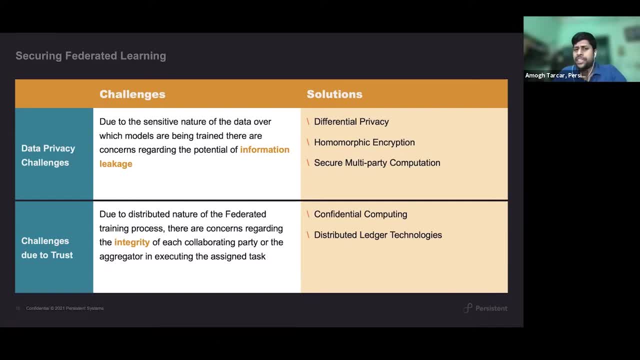 all of them are very concerned about what is the segregator going to do with the model updates which are shared, and that raises concerns about the integrity of each collaborative party as well as the aggregator. so by integrity we mean to say that whatever code which has to run on this particular aggregator of the party, is it running exactly the way it is. 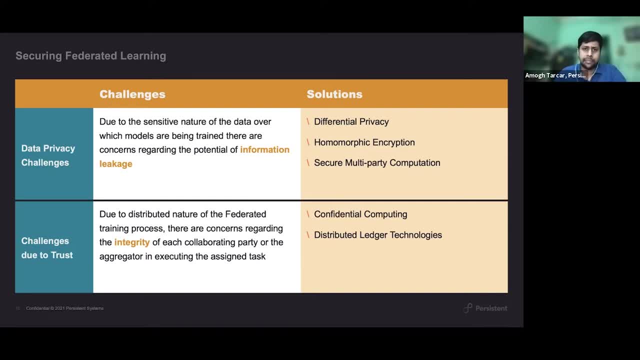 intended to, or it has been altered to, do something else, something malicious, so that basically raises concerns about integrity of you know, and that comes from trust, and suppose there are trust concerns in the setup which we are referring, that's where you know we have to think of solving. 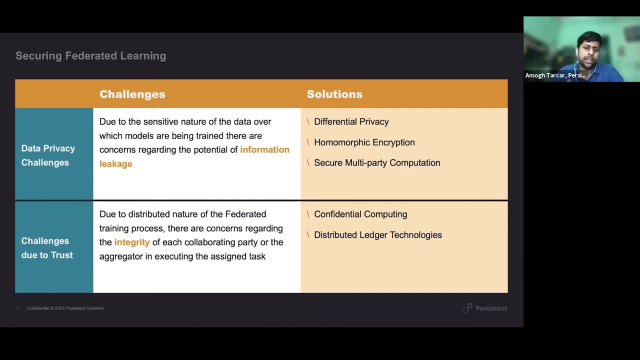 such type of trust issues with technologies which are either distributed ledger technologies like blockchain- blockchain is a it's kind of pitch to solve trust related issues and establish this collaborative trust- and confidential computing, which is a very interesting new paradigm which comes from hardware-backed kind of trust which comes in because you know. 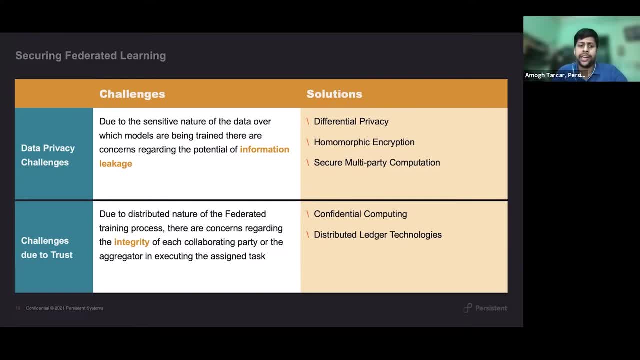 Intel especially has made a special type of hardware trust, which is an existing kind of trust which comes in because you know. intel especially has made a special type of hardware, hardware which can give you guarantees that the code has not been altered and it runs exactly like the way you code it. 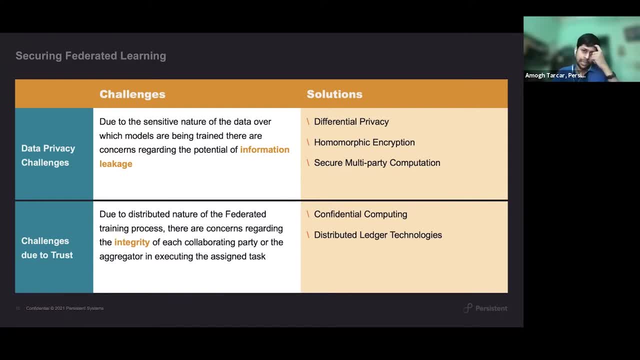 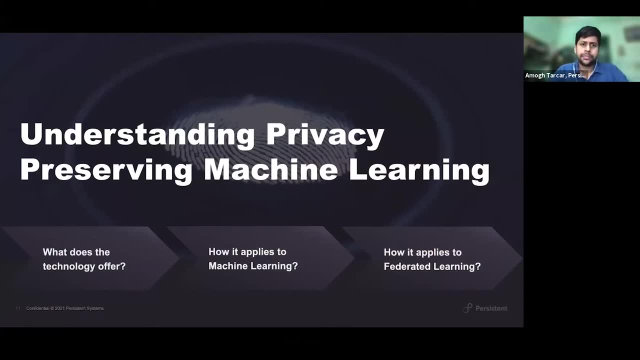 So we'll take a deep dive at confidential computing as well as we go ahead in this session. So as we go ahead, we'll basically try to understand all these various privacy preserving techniques in sort of three steps. First step is: what exactly is this technology? 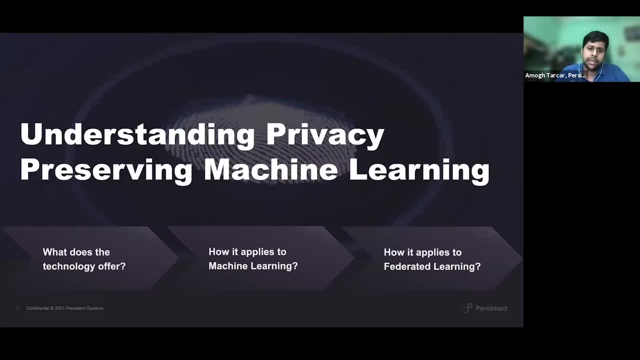 What does this technology offer? Second is how it applies to machine learning in general, like: can you do inference on it? Can you do training on it? Where exactly is it from the point of view of building machine learning? The third thing is how exactly is this particular technology applies to federated learning. 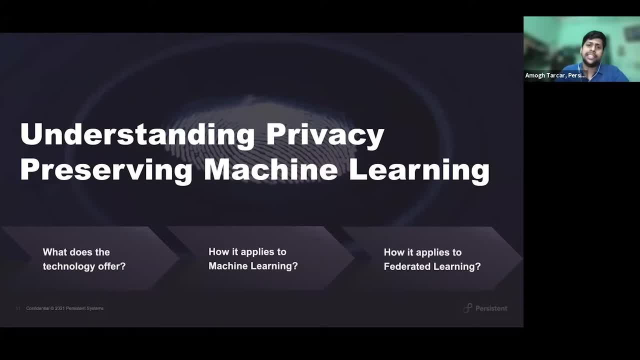 And so the concept is slightly different, because machine learning is much broader and federated learning is kind of a small section of machine learning. So let's take a look, Okay. So let's try to understand from these three broad perspectives What is the technology, how it applies to machine learning and then how it applies. 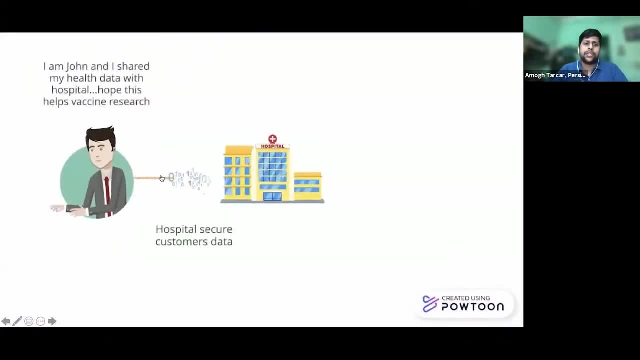 to federated learning. So here I have John, who has shared his healthcare data with the hospital for vaccine research And this hospital basically say it actually tells models by keeping the model, the data safe, but trains the model, And a few months later what happens is that this model is publicly available and some 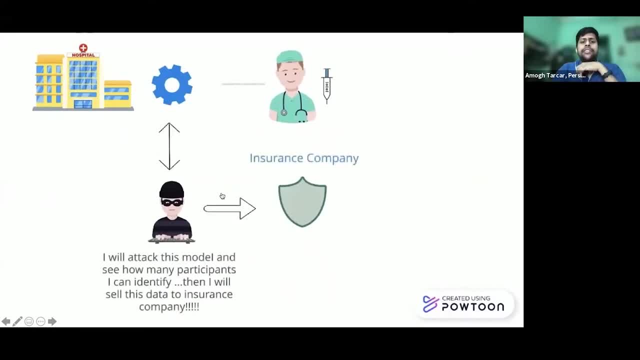 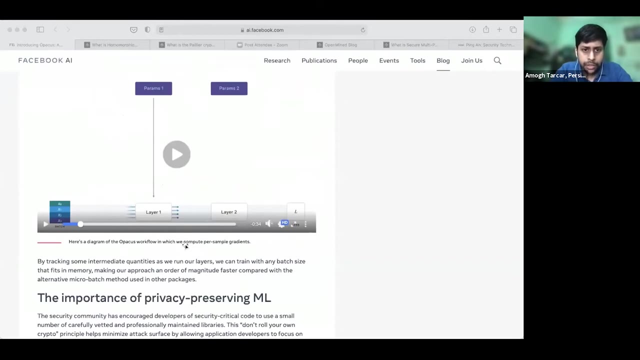 hacker decides to kind of see the model, See if it can identify any participants who have been present in this particular dataset, And we just slow it down a bit so that we can roll a little bit slow. You can still see my presentation that I've just exited from the full screen mode. 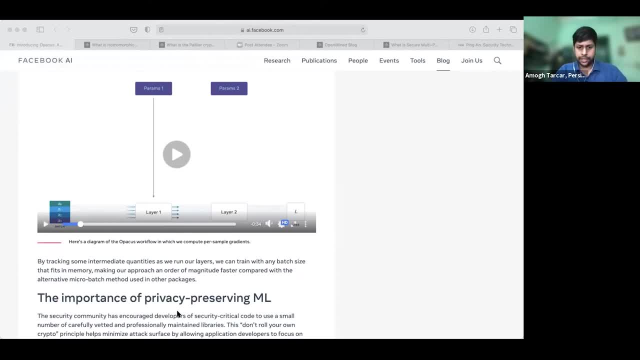 Okay. So yeah, let's just see the session. see the same animation in a slow way. So, first thing is that John has shared healthcare data with the hospital. Okay, So this is the same hospital for vaccine research. Now this hospital basically has secured this data. 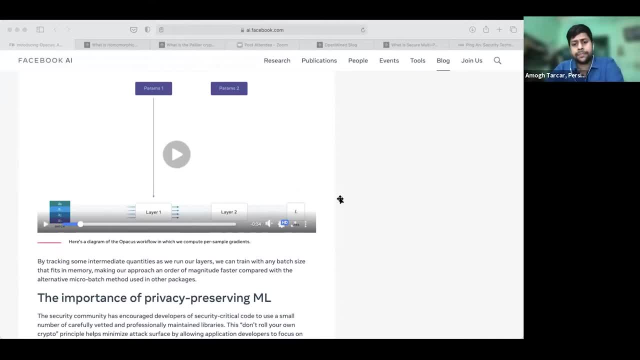 And so the data is going to remain at this same hospital. but the model is trained for vaccine research over this data. So the data doesn't move, but a model is trained on it, say by federated learning or some other technique, And this model basically is available publicly for healthcare researchers to actually use. 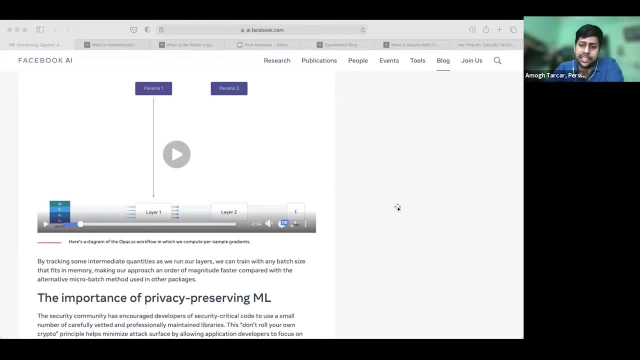 this model and find out if you know for for their vaccine research, They can actually use this model. So that's the current traditional way of trying to build models and then give this model away as a service. So this is completely fine and it's quite common as well, but this is something which 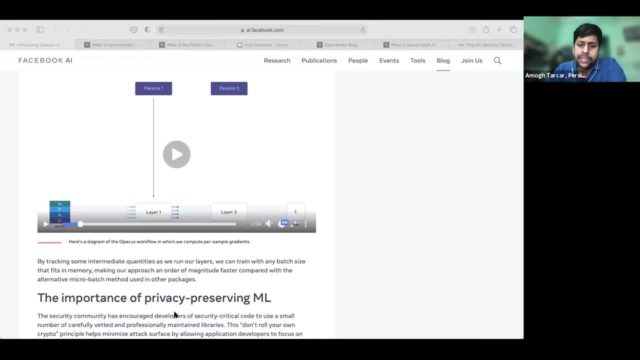 is new wherein, if suppose there's an attacker which which, basically you know, in this case we can assume that the attacker gets some side information about the patients and using that side information, Okay, So the goal of the attacker is to find out if, from whatever data he has, how many of 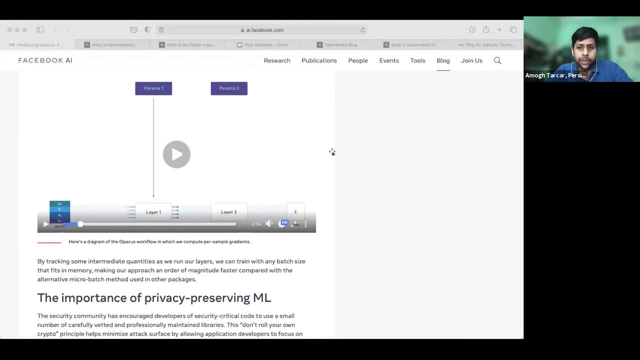 those data points actually present in the model which was trained. So again, to repeat, the model exec is in the weights or the actual, actual data is kept safe at the hospital, but the model basically is out there for public And this particular attacker is attacking that model to find out if certain patients 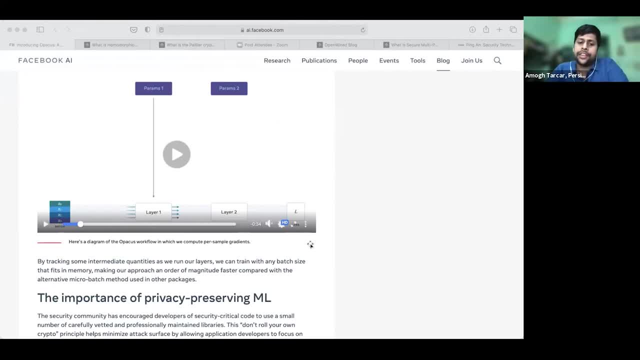 were there in the training dataset. Okay, So if it, if this person adversary is able to identify certain patients, can pass that information to, say, some insurance company who is open to such data and that insurance company can basically, you know, use this information against you. in saying it, it basically: 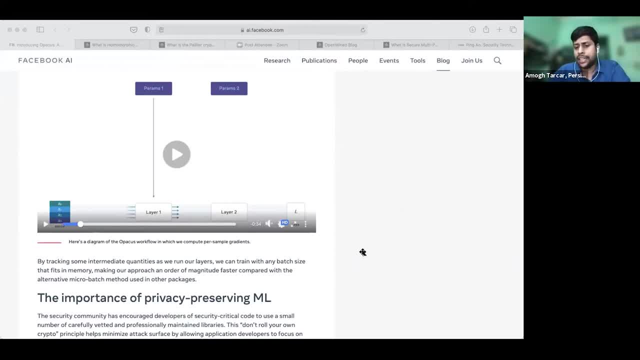 directly increases your premiums or some sort of. you know it does a kind of malicious act and what you get as an end result is that your premiums have increased. Then You are not directly, you know, you are not aware of how exactly your data reached here. 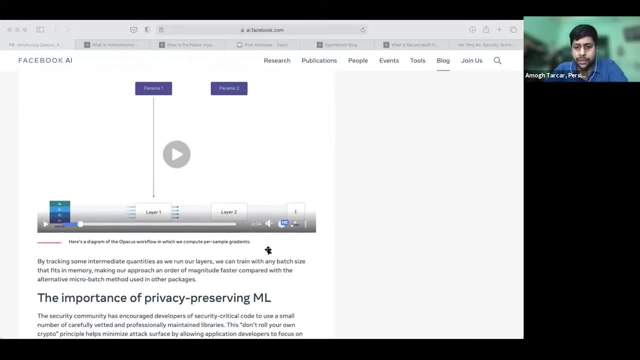 And that's kind of what this insurance company and the attacker, you know the together as such, without your knowledge, and what you get is that they now know that you are having a higher cancer of risk and it may be even possible that you don't know that you know. 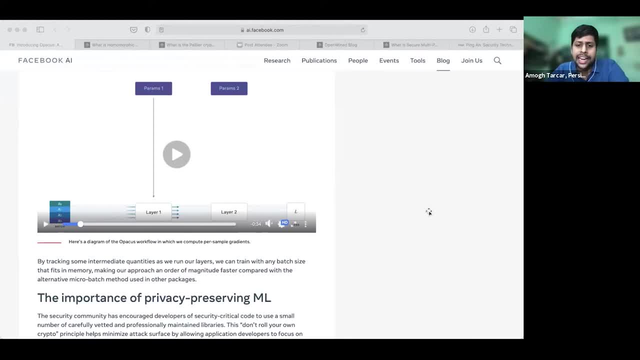 you have that high cancer risk or something that way. So this kind of you know acts are kind of dangerous, Okay, And that's what we, you know, we can take a deeper dive in. So now, if we try to understand what exactly happened here is that: did the hospital leak? 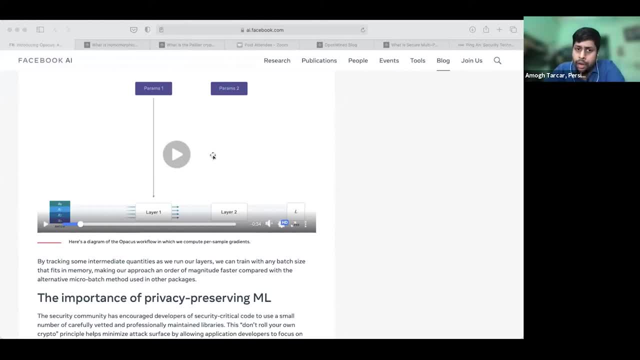 data. No, hospital did not leak data, because hospital kept the data where it's supposed to be: in the hospital and train the model and the model which was there. in case it was over fit, then it basically what. what the model can do is that it can give you, like you know, you might. 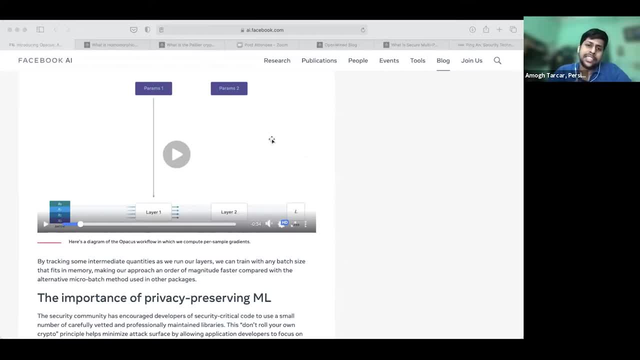 have also noticed it when we train models, that whatever is in the is in the training data gives us a higher confidence score at the output than the others or other data points which are not there in the in the model, And what that happens is that you get a big divide between what is there inside the training 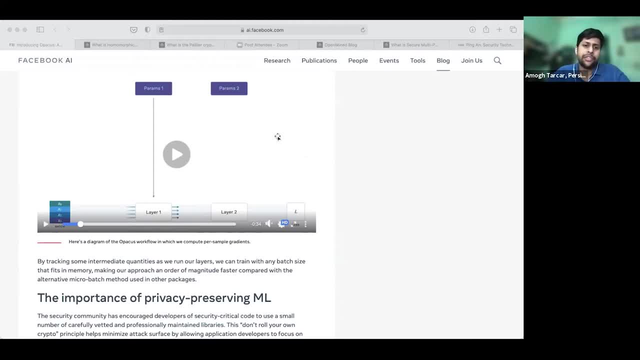 data and what is not inside the training data and those kinds of differences, is what an exploit or attacker can able to find out and use that against you to leak the information such as this. And this attack is called a membership. Okay, This is a conference attack. 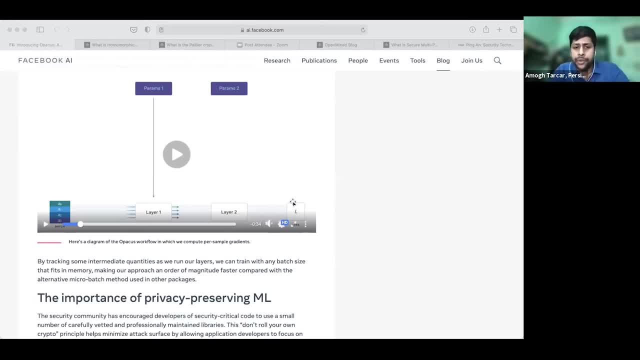 And in this sort of attack, the purpose is to find out if you can find, if you can figure out a pinpoint, a few people who might be present inside the training data set. So that that's the scenario in which, you know, we have to start thinking about saying: 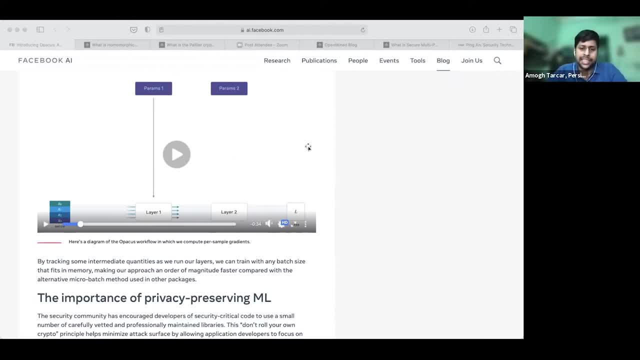 the data is safe- safe, but the model is out there. and what exactly can adversaries get or learn from this sort of, you know, exposed models? And that actually brings us to you know why, Why some sort of security is required when we are performing machine learning in general. 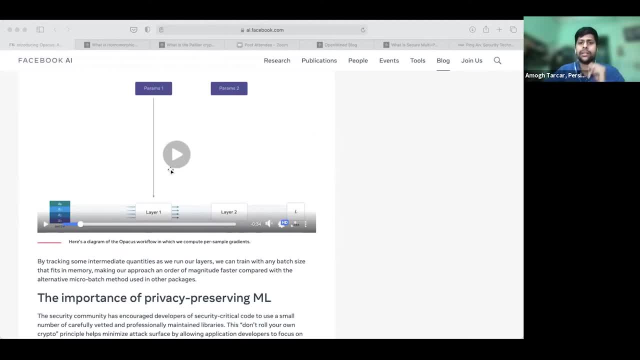 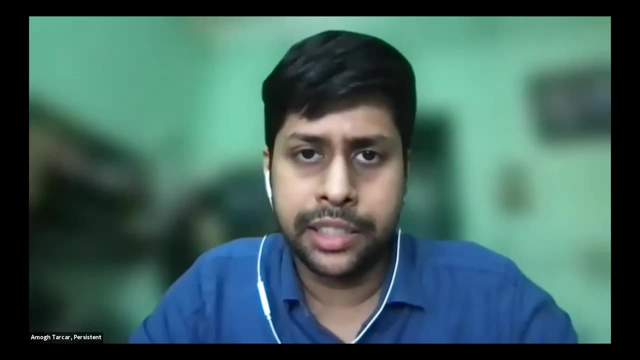 as well as in federated learning. So let me cross check again. So what screen are you seeing right now? Are you seeing the animations or you're seeing the browser? Okay, Then what I will do is I'll stop sharing and I'll share the screen again. 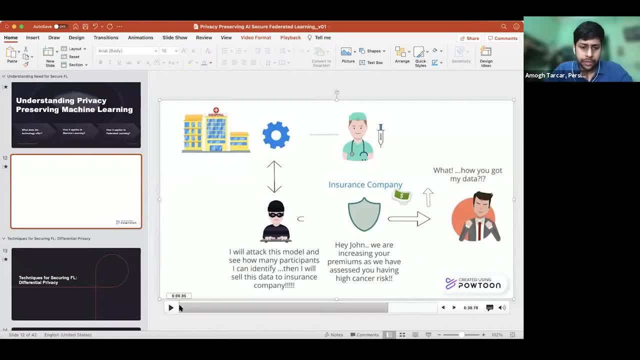 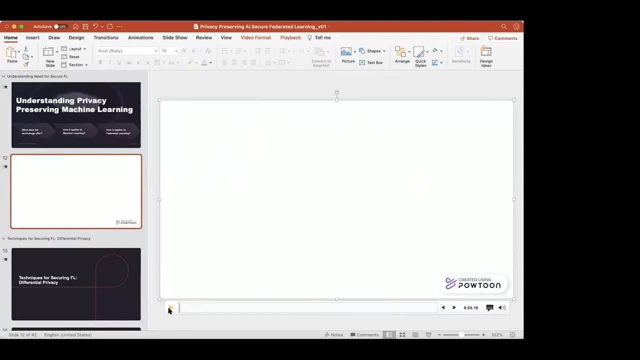 Okay, Now are you seeing the animations? Yeah, Okay, So let me quickly just replay this animation so that we build context again, So we know that the like we can share data with the hospital and hospital has to keep the data safe. and the hospital does that, but trains a model which is then open for. 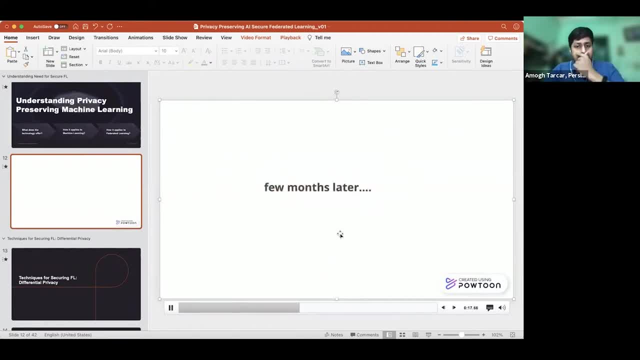 public use, And then this model is basically susceptible to overuse. Okay, And then this model is basically susceptible to attacks. So if an adversary tries to find out and the exploit basically is: you want to find out, can you leak any information about whose data was present in the in the training dataset? 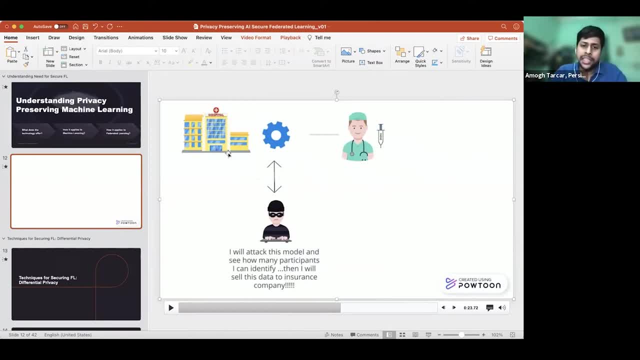 So you don't want to, isn't like the task is not to leak that patient's data directly, but you just want to find out if that patient was present in the training dataset. So, and if you do that, basically you come to know that. 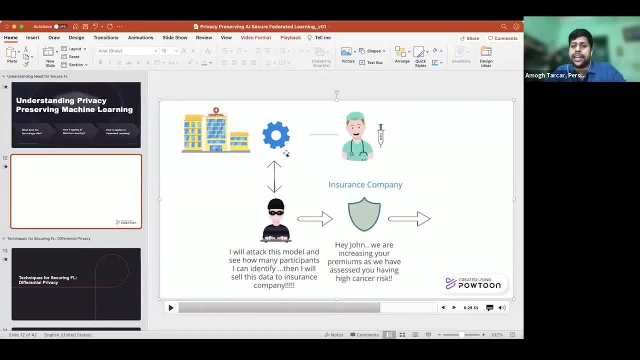 Okay, The patient was there in this particular study. So you sell that data to insurance companies. say, who is kind of, you know, going with sort of a nefarious inclination over here, and they try to, you know, find out if they increase. 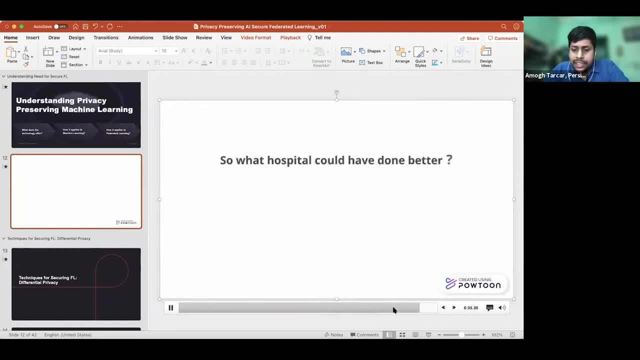 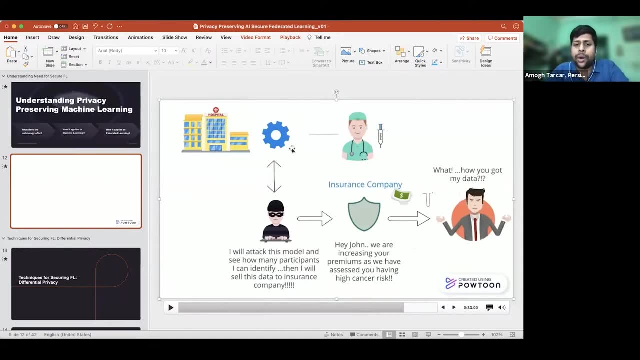 your premiums And basically, in this whole setup, what actually happened was that that model was attacked. It's not, you know, that model did not leak. the data rose directly, like the actual data was leaked, But what this attacker could get is whether that particular patient's data was present. 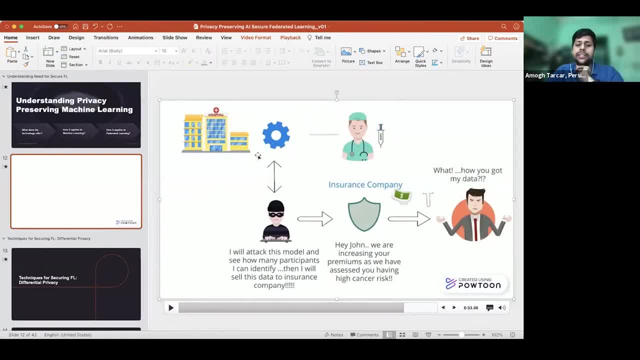 in the training data, set or not, And just with that information they can then, you know, try to run some other, like other adversity attacks and so on, And they basically, you know, can, can use it for their own personal gains. 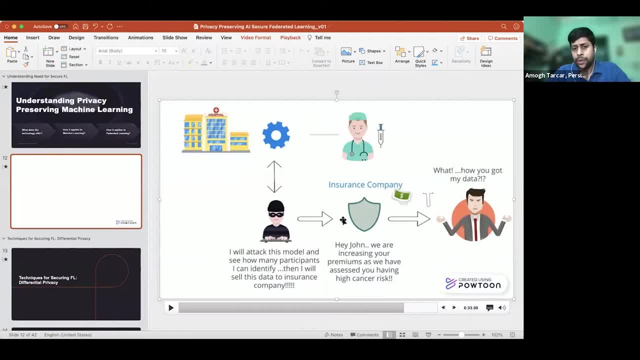 And that's the scenario which which we can get into. then we train in federated learning. So suppose this model is made available for public, What exactly? what can we do? Okay, What kind of things can this particular model leak and how can we protect against it? 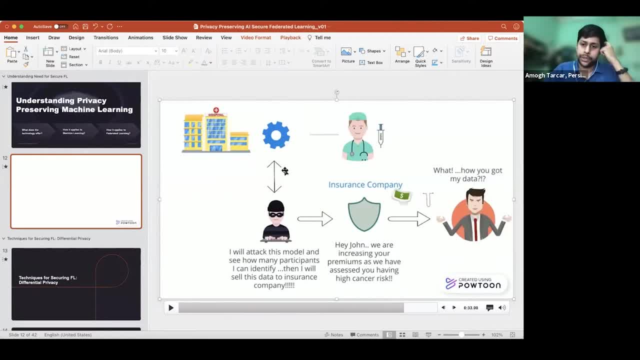 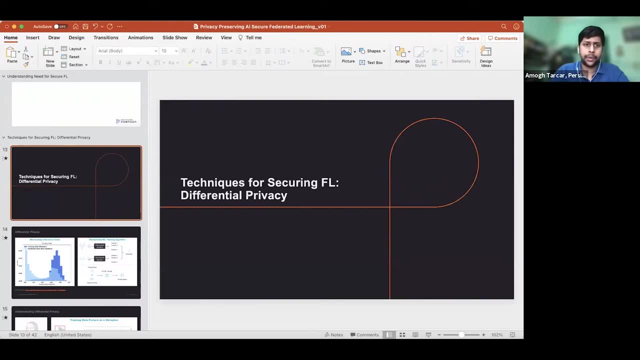 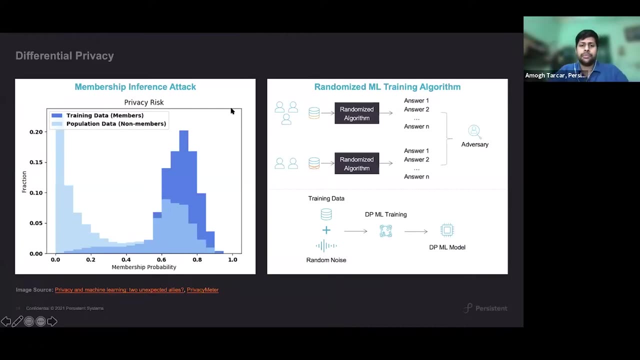 So any questions on this scenario, which, which we kind of observed instead of see how can we prevent this sort of thing, may go back to full screen. So yeah, So, from from a you know, visual point of view, this is what sort of you know happened. 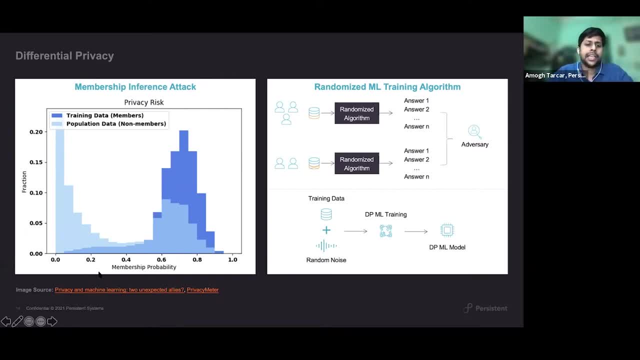 in the membership inference attack. So we have something called as this membership probability, which is basically the probability of whether this particular data point was present in the training data set or not, And this is something which we observe usually in very overfit kind of models. 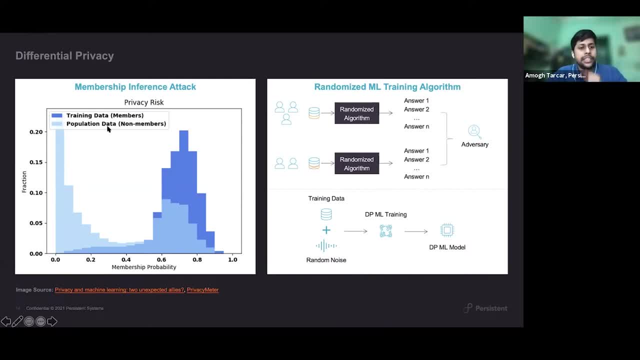 But then see if we can clearly see the training data versus the population data And you can see this clearly divide between, you know, the dark regions and the light regions, And so the light regions are kind of the probability is is low and the dark regions are probabilities. 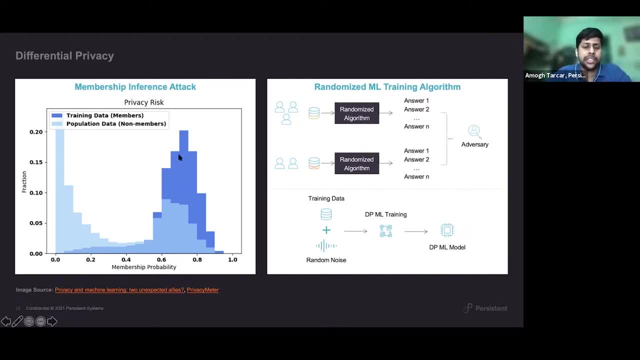 very high. So any data point in in this kind of region, you're more certain that that data point was actually used in the training data And that's something which this particular membership inference attack kind of exploits. and the adversity comes to know whether that particular data point was present in the training. 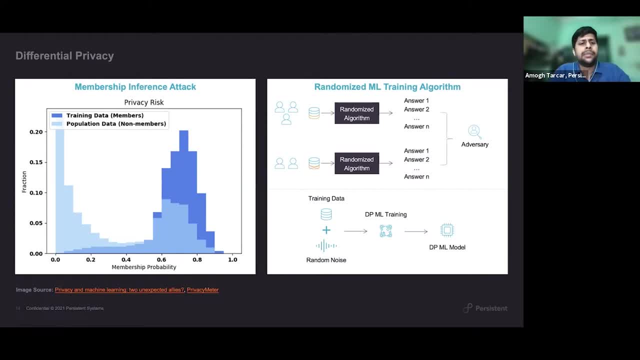 data or not. And you know we ran some experiments on this and basically this what we're observing. right, it's not that very common. It basically happens when you have sort of you know, overfitting happening or there. 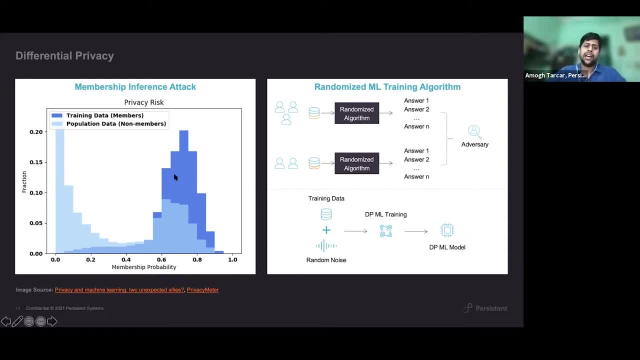 could be multiple other reasons why this could be happening. as such. It could be sometimes that you know your training data is actually a very like. it's not that diverse, It is very closely related. it's kind of you know from a pure machine learning point. 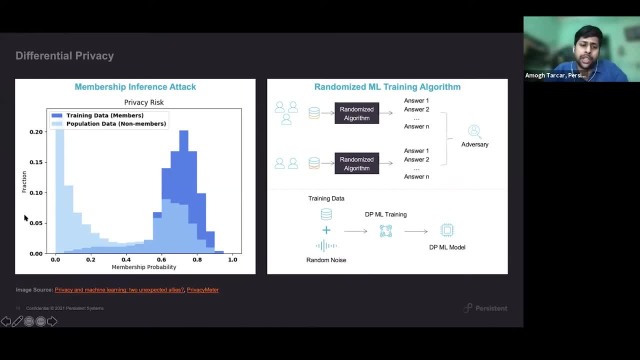 of view. If you try to take a deep dive, You can see why this sort of a divide happens And that basically can be attributed to the type of data you're really running. So oftentimes if you increase the size of the data set, then this, this kind of neutralizes. 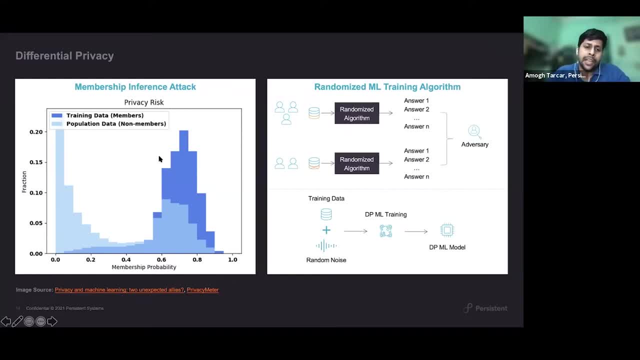 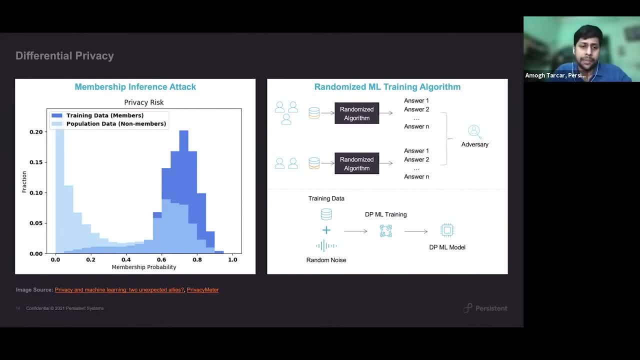 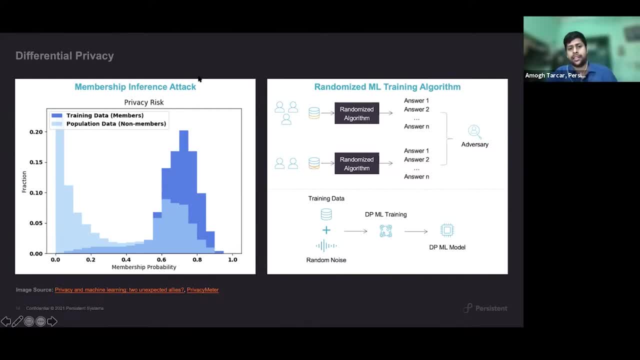 the real world. In fact, this basically attack was shown by researchers from, I think, University of Pennsylvania, wherein they're actually shown that these attacks actually happen and you can leak information about the training data. You can actually try to understand more from this blog post by Nicholas Papernaut, which 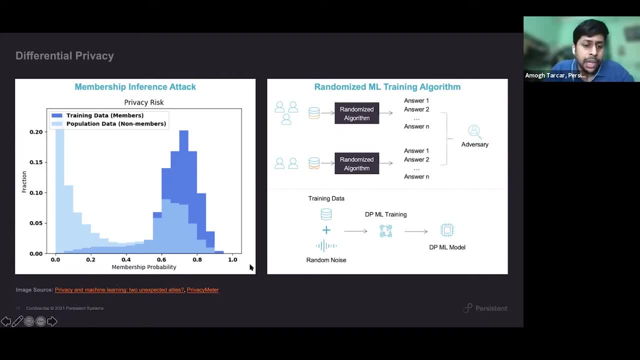 is about, you know, privacy and machine learning being unexpected allies. So they have even went ahead and built tools such as privacy meter to kind of take a deep dive in doing membership inference attacks. So in the research community these attacks are kind of, you know, very prolific and outside. 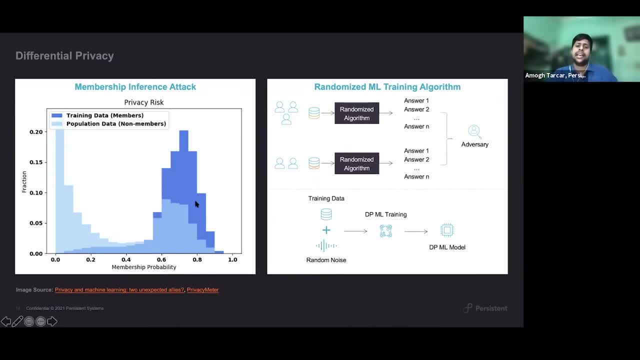 the research community also, there have been multiple cases wherein such attacks have actually happened. Utkarsh, to your question of homomorphic encryption: when we come to homomorphic encryption I'll explain this. It's possible, but you know, we'll have to just understand the nuances of how exactly. 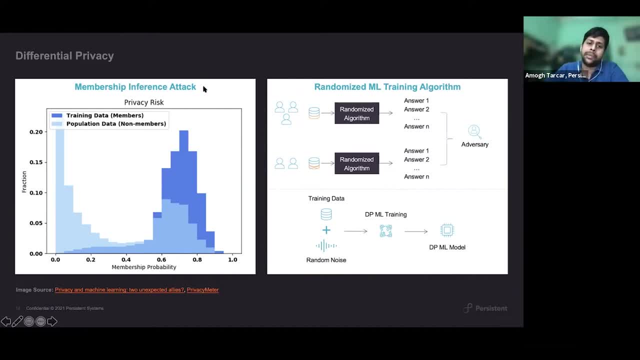 do we apply encryption to see if membership inference attack was possible or not? So before that, like you know, let's try to understand the first technology over here, which is differential privacy. Can differential privacy help in reducing such attacks? And the answer is yes, it can, but we need to understand what is differential privacy. 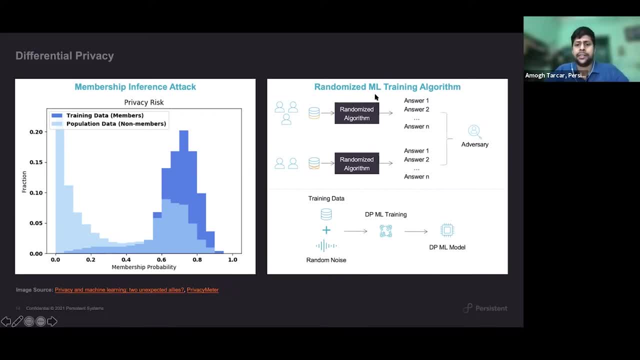 And the high level understanding is that the probability of trying to find an answer should not change in case a particular patient or a particular data point is actually removed from the data set. So essentially, what you're saying is that you know the final answer, the probability. 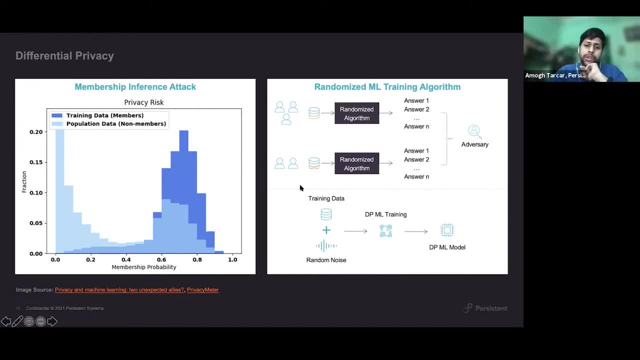 of getting that answer should remain the same, whether your data was used or not used, Okay, In the same data set or in the same training set. And that, basically, is you know, that's the, it's the crux of differential privacy as such. 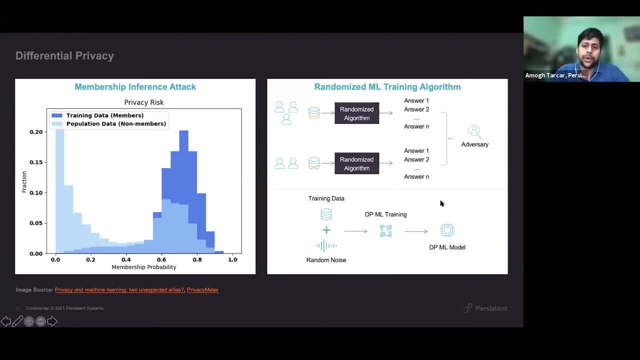 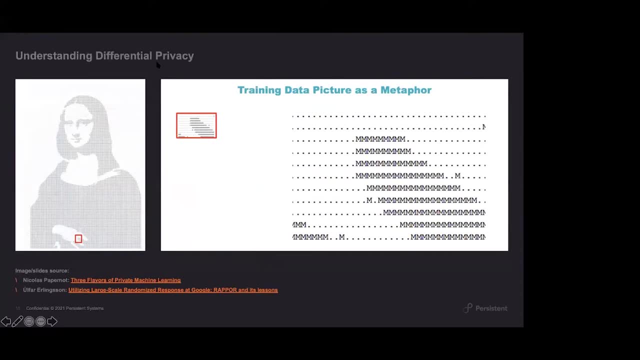 And you achieve that by applying noise to the overall system. Let's just take another example to further get this done. So in this slide we can see, that is this picture of Mona Lisa, and I've picked the slides from Nicholas Papernot's very recent talk on 3D. 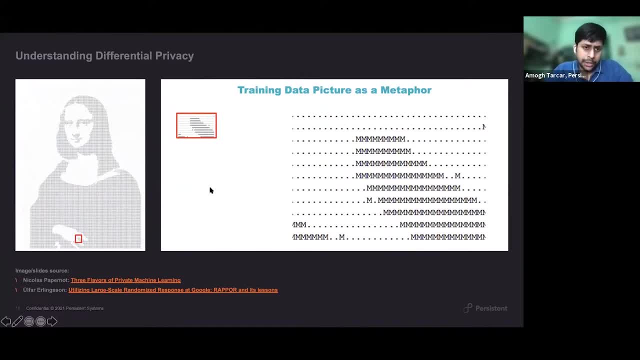 On three flavors of private machine learning. And this particular slide as first, I think, appeared in Ulfar Ellingson's presentation, So credit goes to them for you know making this visually very easy to understand. So first thing is that you know we see this Mona Lisa picture and each of these data points. 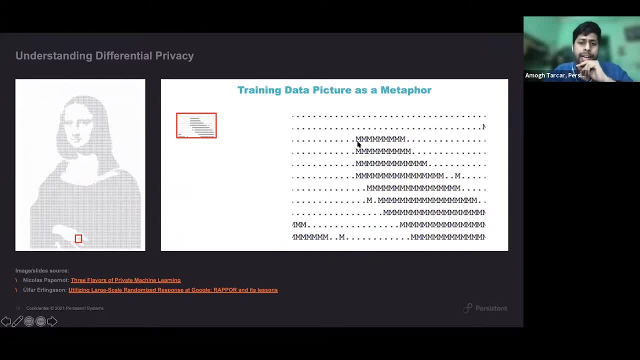 which are making up this picture is actually either a dot or an M, So dot and M could be individual data points which are all put together. Okay, You get your bigger picture of Mona Lisa. Okay, So that's how we can look at. you know, training as a part of this. 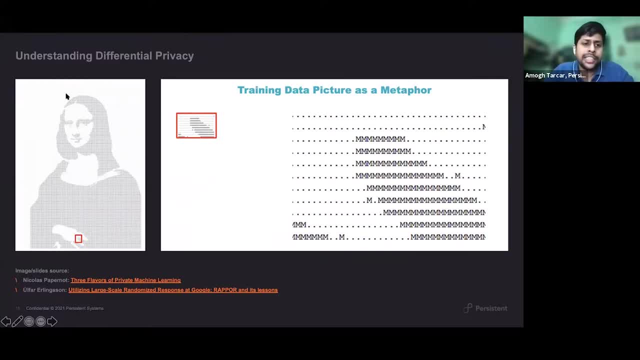 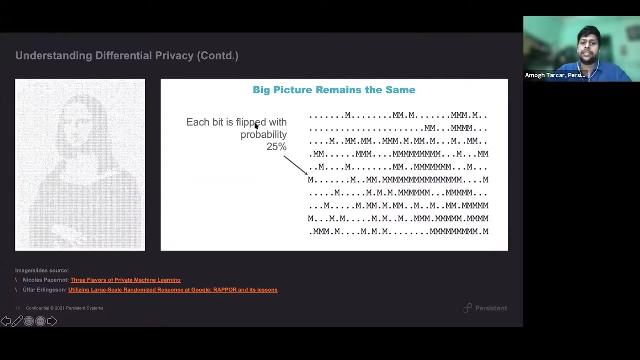 Like each data point is contributing something And the overall is the pattern which is observed, And this pattern is what we are always interested in. So what differential privacy can do for us is that it can add some noise on these data points. Like each data point is flipped by, say, probability of 25%. 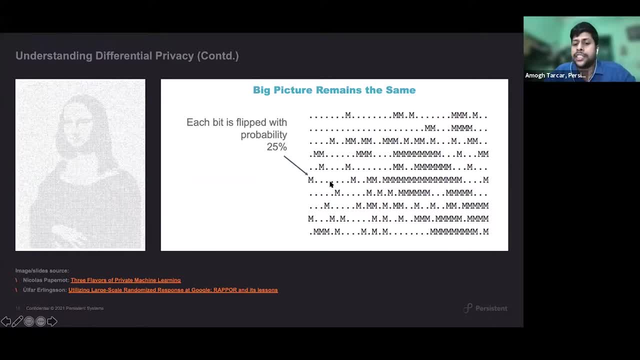 Right, So we basically randomly go in and, instead of using the real dot or a real M, we basically use this technique and we add noise to the system so that we randomly go and actually change some dots to M, And when we do that at the individual level, yes, you're changing the data point. 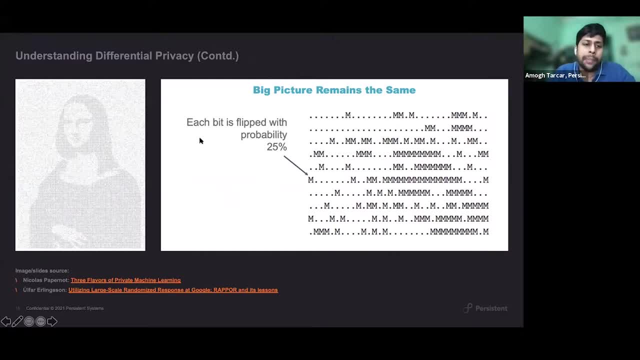 But what happens in the bigger picture of what is the overall pattern you're trying to learn, is that that pattern, as you see over here, it's very noisy, Yes, but it also shows the Mona Lisa picture clearly. So this is the analogy in which differential privacy can really protect your data point. 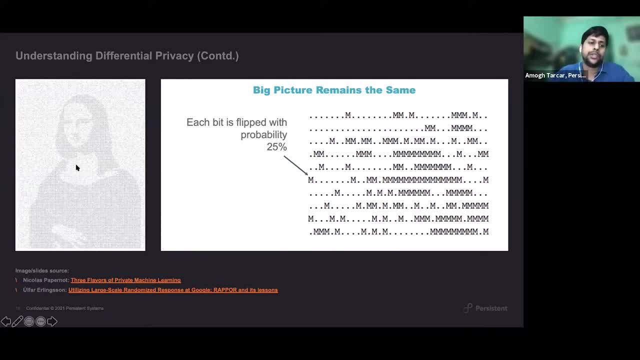 So what happens in this case is that if you pick any data point or you do say machine learning on this kind of data, even if you leak the data, you basically just you know you can never be sure if that dot or that M actually came from that person. 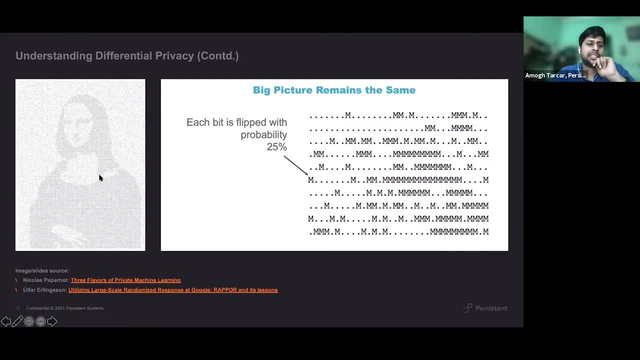 And also because we are adding this noise in a very systematic way, We know how to get rid of this noise as well. So that's something, you know, which we can do at like this is noise basically being added at the data level. 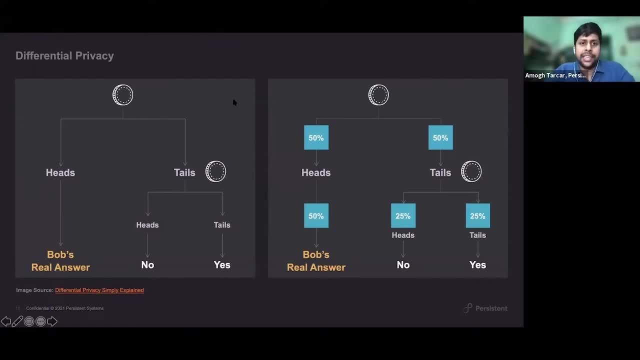 So let's just take another example in a similar way, to try to understand how exactly is differential privacy can be added to a specific data point. So suppose you want to ask some sort of a very sensitive question to a person say: So, you know, like the analogy which we had used of dot and M, let's try to put a question on that. 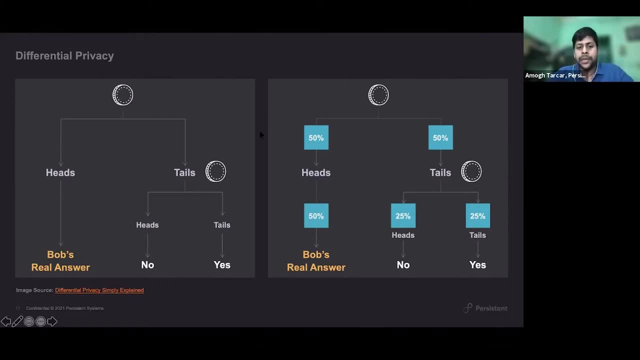 Say we want to basically understand from like. we are trying to run a survey across our own company and we want to know how many people are actually dissatisfied with the company and want to quit. So naturally nobody will be really, you know, very eager to give the real answer in the first go. 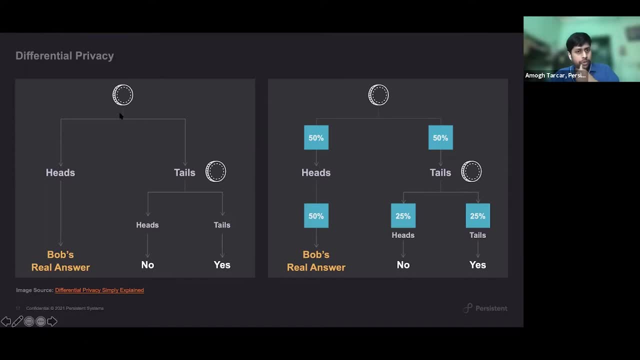 But if in case you can, you know, tell them to flip a coin the first time the coin gets flipped. if it comes heads, You tell the real answer, And if it comes tails, you just have to flip the coin again and just tell what the coin says and not your real answer. 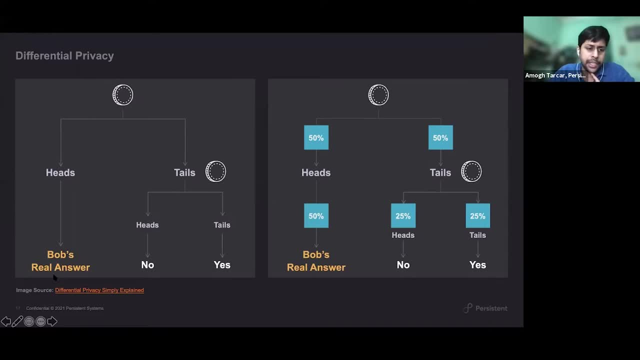 So you just flip the coin and it comes as heads, You tell your real answer that yes, you would like to quit the company or you don't want to quit the company. And if it comes tails, you just flip it again and just tell: if it is heads, you say no, if it is tails, you say yes. 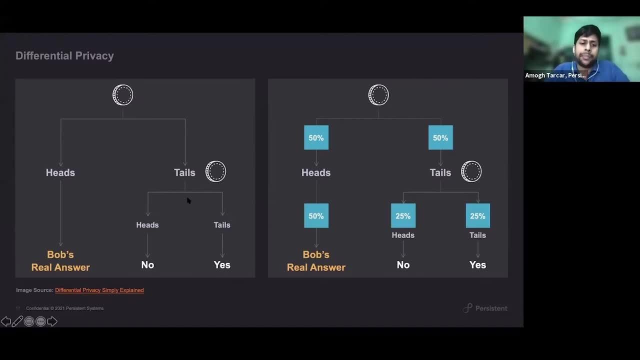 And this is one systematic way in which you know, by flipping these coins at the point when the data is in fact getting collected itself, you can add differential privacy And if you do any further, you know trainings on it or any further action on it. you're kind of you know, sort of plausible deniability. 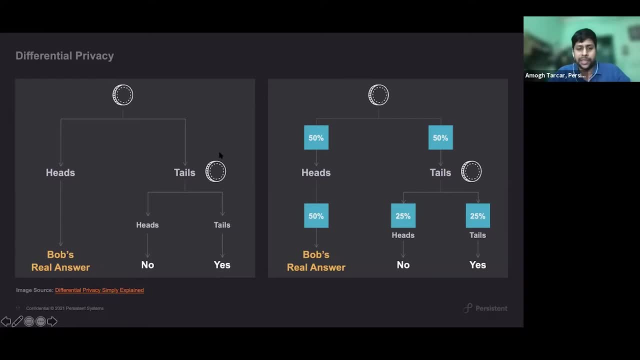 always is with you that you can deny saying no. I said that answer because of the coin came to be tails. So this is the thing we are providing at a user level: some sort of privacy, But at the same time, when the data is- you know the noise which is there- is getting uniformly added across all the data points. 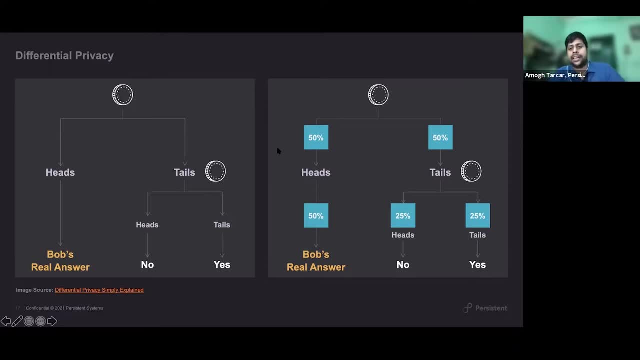 And you can remove that noise because you know how much exactly You can calculate The probability and and from the bigger picture, you can remove that noise and you'll you know you'll get an approximate statistic of what your answer is. 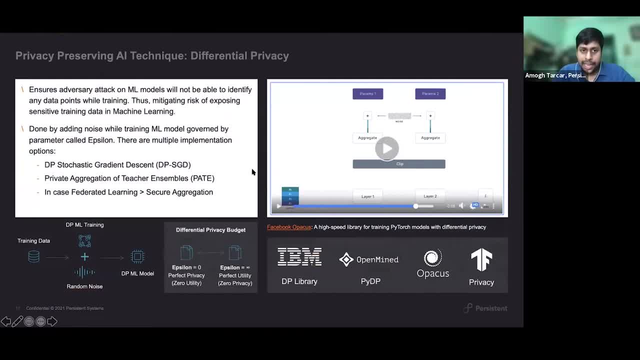 So that's basically differential privacy, which actually adds noise in in the algorithm in between, then basically, you can add noise to the training data, as we saw in the example. But recent examples also use differential privacy, not on the training data but on the actual, you know. 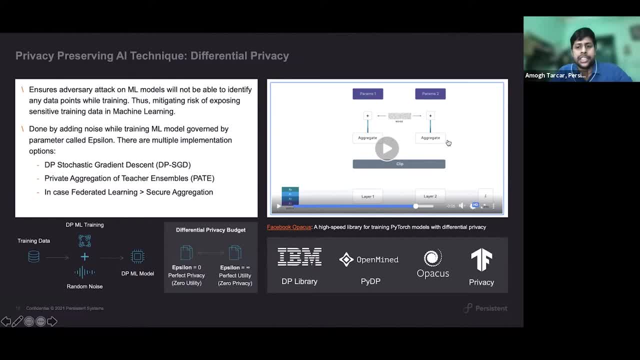 wait updates which happened during training of machine learning and Facebook's Packers library is something which is exactly that. the same kind of you know implementation also in these can be done with TensorFlow privacy as well. So that basically is called differential private stochastic gradient descent. 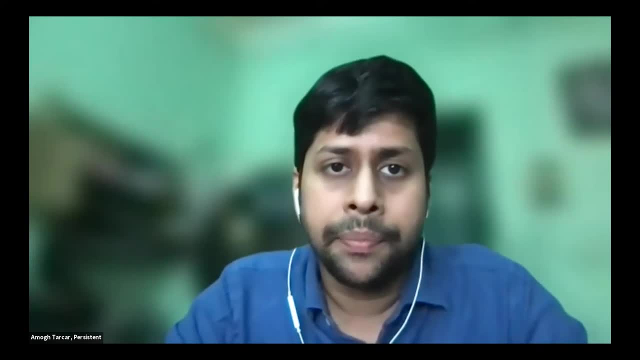 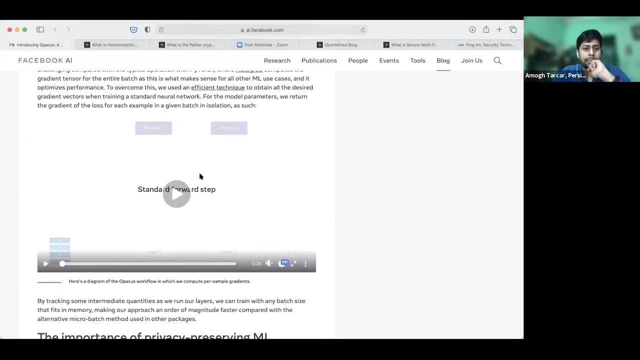 And there is a nice animation which basically shows that. So here it is. basically, you know, this is Differential privacy being applied at the time of training. So let's just see this GIF. It makes it very clear to the normal standard step forward in the neural network is it happens like normal? 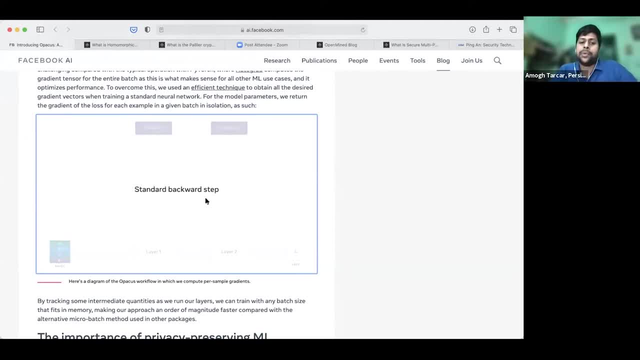 And after that is basically this backward propagation step. So in that case we compute the losses and we are trying to update the parameters directly. But in case you want to apply differential privacy, we can actually not update the parameters Directly, but instead just clip them all together. 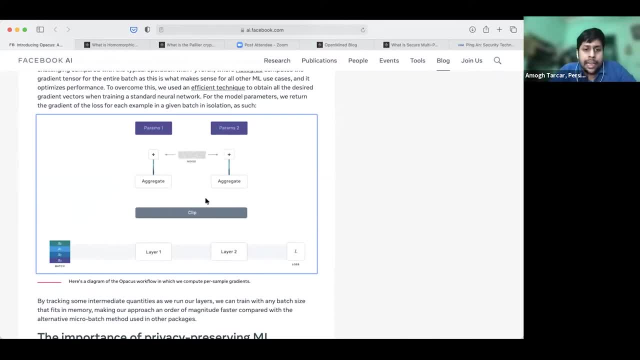 And then aggregate all of them, add some noise And then update it. So what basically this allows us to do is that we are essentially adding. you know, we are basically saying that each of these- in case you know, if our neural network is such that it's trying to even make the weights- are trying to really remember what was the real. 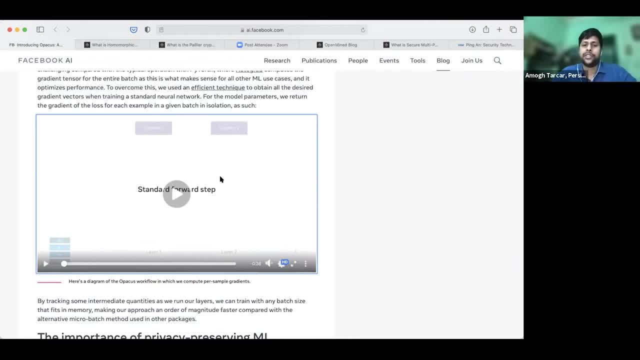 In Input. this technique of a package, kind of you know, helps mitigate that sort of memorization of the data points in the neural network itself. So when you're clipping it and you're adding that noise, you're making sure that you're not letting this particular model memorize the data, and that can have really good benefits. 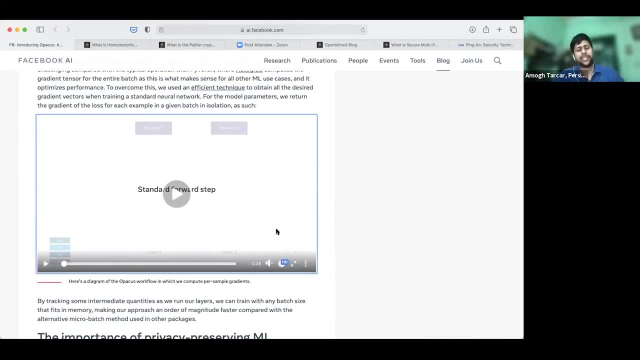 So it has benefits for like better general, general generalizability of this particular model, as well as you get this privacy guarantee. So it has benefits for like better general, general generalizability of this particular model, as well as you get this privacy guarantees. 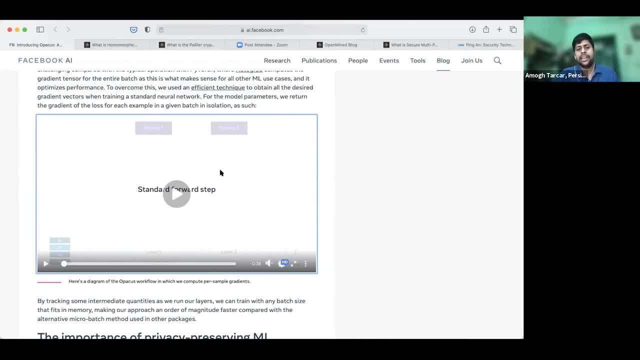 That however much this particular model is out there and somebody really tries to attack it for doing, say, membership inference attack or some sort of you know model inversion attack, They will not be really able to get hold of the data point. but and this particular model, 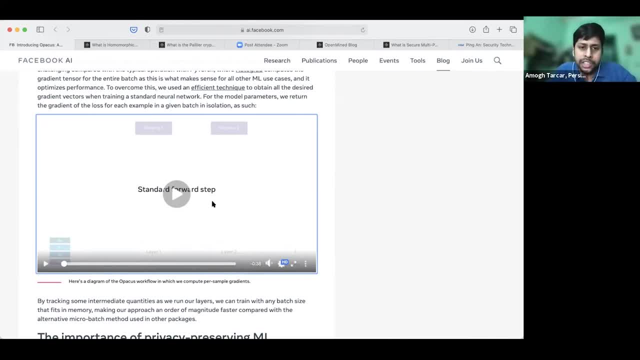 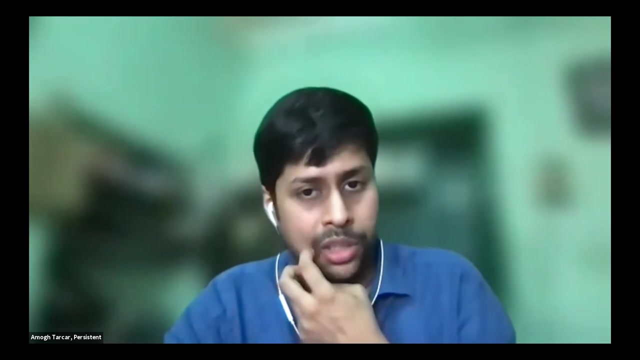 So on one side, you're actually helping generalize the model. on the other side, you're essentially mitigating such type of attacks. So differential privacy can help us get all of this. But yeah, as as Dr Sharman mentioned in the chat just now, yes, the noise comes with a negative, which is it has a direct impact on privacy, on the accuracy of the model or the performance of the model. 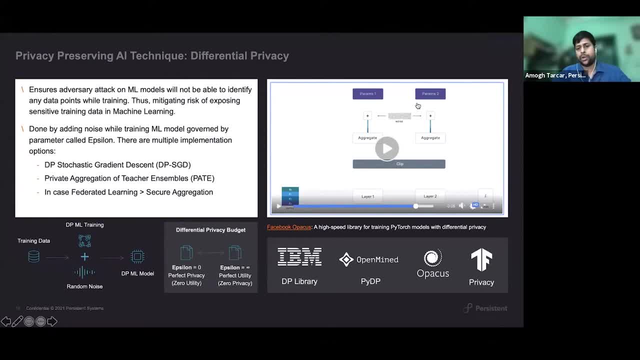 So, coming back to my slides, you basically have, like, this noise is sort of controlled by a value called epsilon, And this epsilon can go from zero to infinity. with the smaller the number of epsilon you get better and better privacy, The higher the value of epsilon. 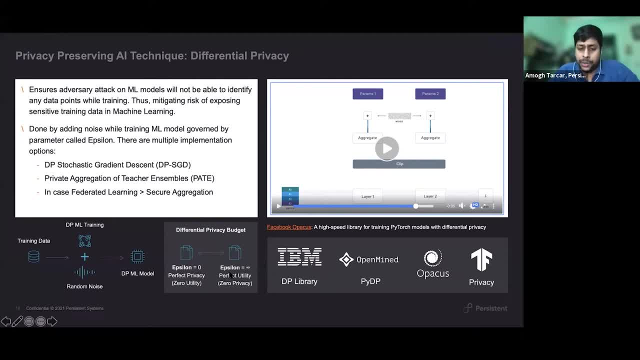 You, basically, are going more closer towards you know, not adding noise at all, and that gives you the perfect utility. So you it's it's like a very difficult balance between perfect privacy and perfect utility, and you want to be somewhere in between here. 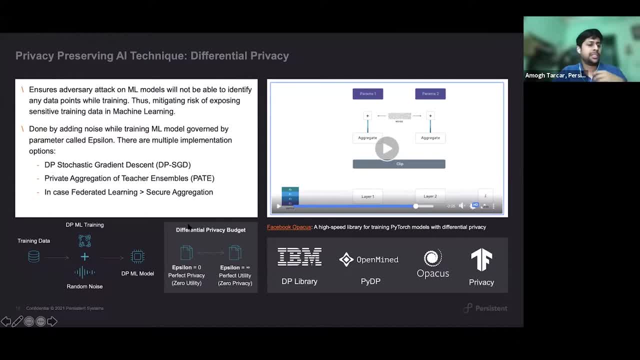 And I'm really glad that you know. Sneha Kumar Sahani from Persistent has been researching on differential privacy and he has some very novel ideas on how can we really arrive at this epsilon and get that trade off. So I'll let him explain that. 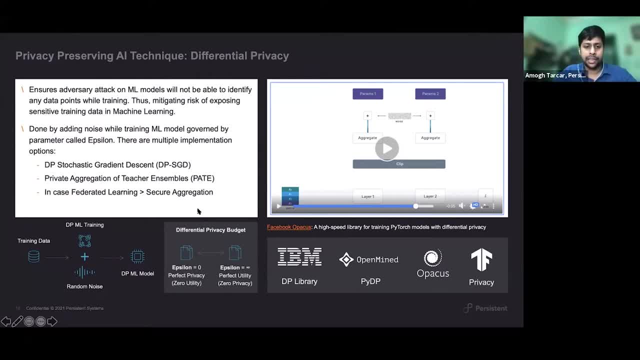 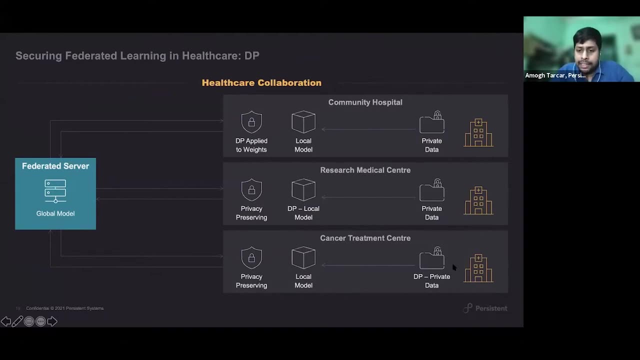 Okay, So I'll let him explain that in more detail in the next session and we can progress further towards how differential privacy can be actually applied in federated learning. So in federated learning as such like. so we saw that you know you can apply differential privacy at the private data level, which basically makes it very noisy. 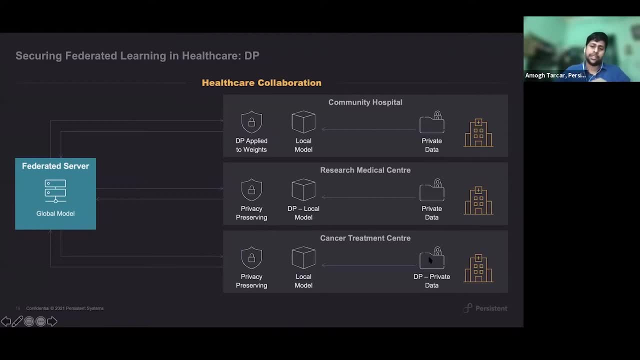 And when you're trying to learn, that's something you're kind of more skeptical in case the data is not even moving. So if you're trying to learn from that location and you're still applying differential privacy, you may not want to kind of, you know, apply differential privacy on the private data, but you can do it in case you have a large amount of data that way. 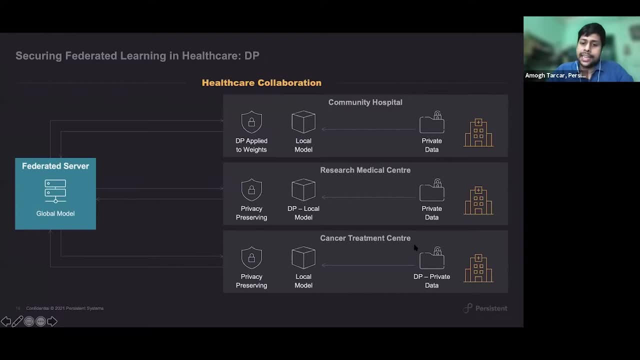 And you can kind of still do it. Second level is you try to train the machine learning model with differential privacy, And if you do that again you have to compromise on the accuracy a bit or you basically have to scale up your data to kind of, you know, compensate for that. 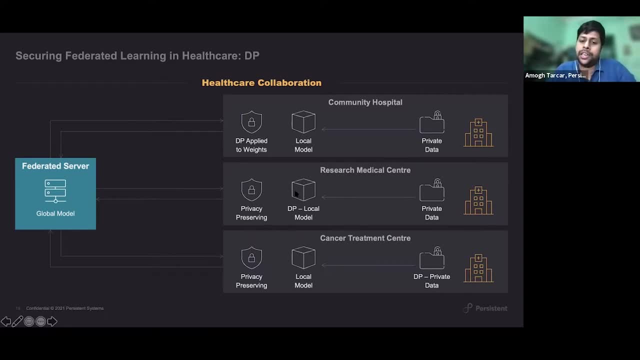 So that sort of accuracy shift which will happen because you're training in a privacy-preserving way And the third option, basically, is a little bit simpler but again challenging from a real-world implementation point of view. That is, for every time you are going to send your weights up to the federated training server, you basically apply this differential privacy on those weight matrices. 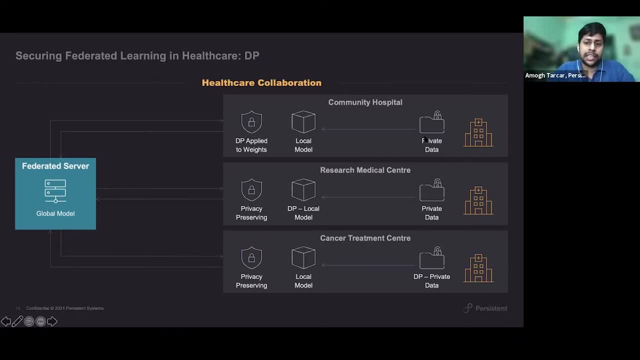 So you are not sending your weight matrices in the clear, but actually you're sending A differentially private version of that matrix and sending it up to the federated server, And the federated server will actually put together these noisy updates and get you NI updated parameters, which you will continue training further. 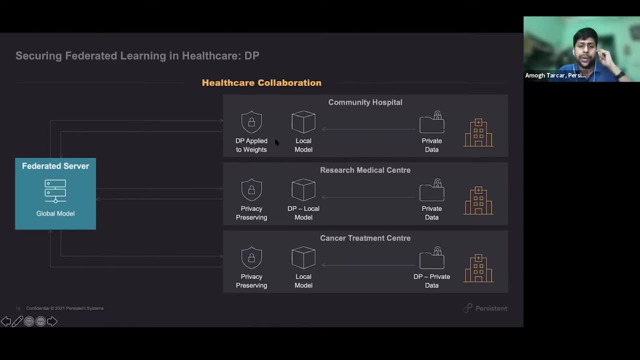 And so what is actually observed in the industry is that when you have a large number of such parties- like when you are, you know, aggregating over, say, 10,000 or 20,000 different phones and you're applying different- if you're applying federated learning across a cross-device kind of scenario- 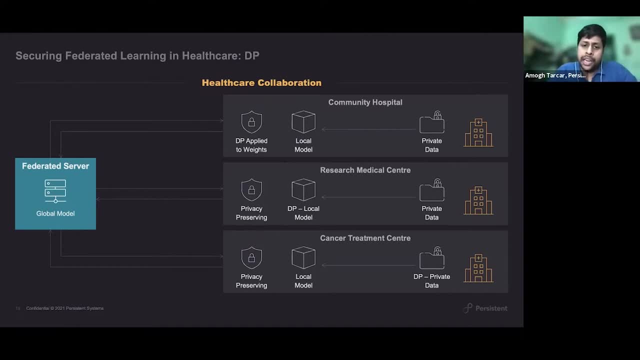 and you're applying different- if you're applying federated learning across a cross-device kind of scenario, and you're applying different- if you're applying federated learning across a cross-device kind of scenario, differential privacy really can help you there to protect data from users' phones, as well as those models. 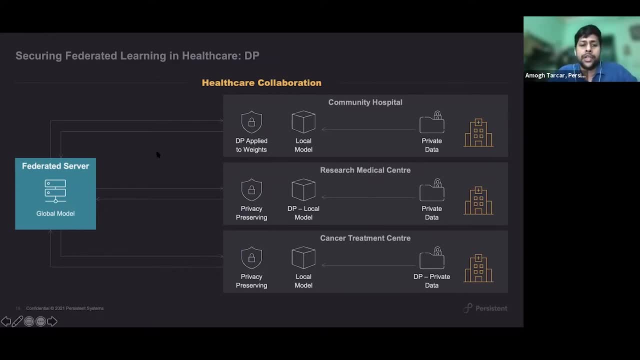 And also because you're operating at that sort of a scale, your noise can nicely be canceled out and you get good observations there. But in case of you know less number of parties joining in, like just four or five parties joining in, and the data size is also pretty big. 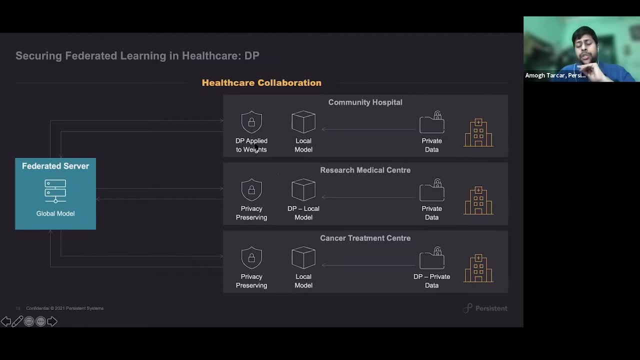 Differential privacy. basically, to achieve the same level of differential privacy and get those privacy values, you need to have a lot of data. So you need to have a lot of data. So you need to have a lot of data. So you need to have a lot of data. 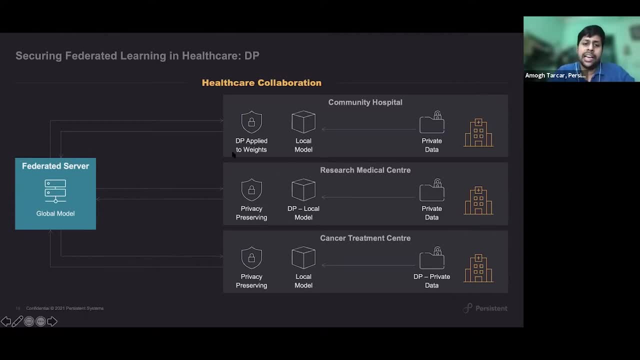 The noise which you need to apply actually is quite large And that basically makes it a little bit harder to apply differential privacy in this sort of a setting. So basically, in those settings, differential privacy is often combined with other techniques to achieve the same level of guarantees. 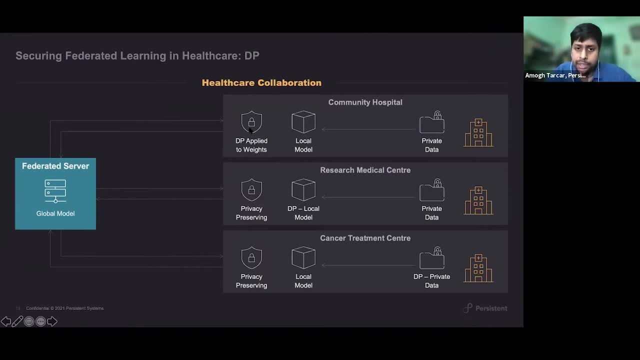 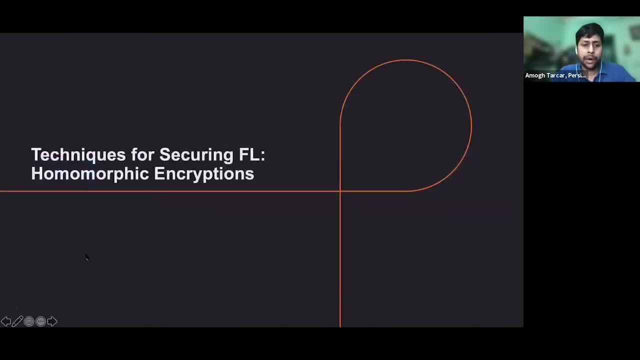 And we will take an example and take a deep dive on exactly how that is done after we learn our second important technology. So that's what I had about differential privacy. We have a session also coming up which will take deeper dives on differential privacy. 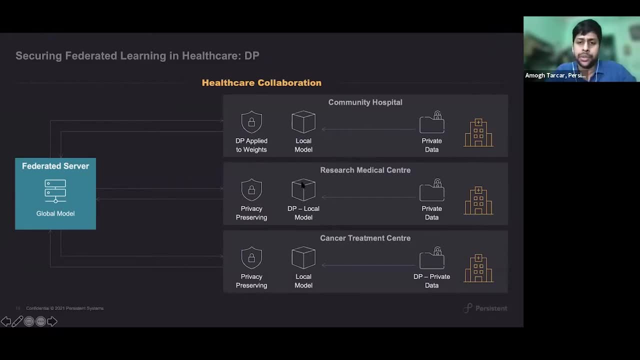 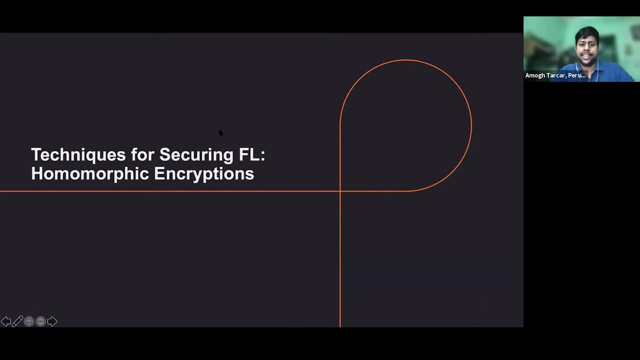 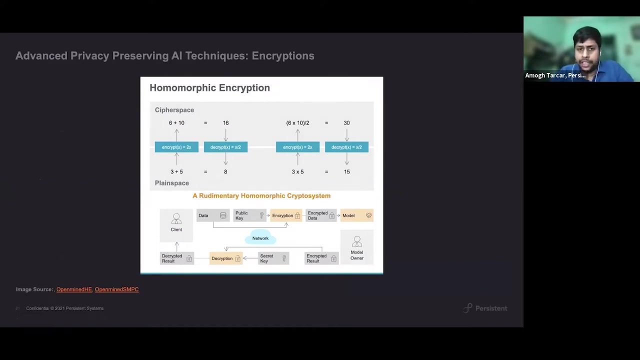 But with respect to how it is applied in predated learning. if there are any questions, we could take them here. So I think we can go ahead with learning our second technique, which is homomorphic encryption. So the concept of homomorphic encryption is kind of straightforward and it's something which is like very desirable. 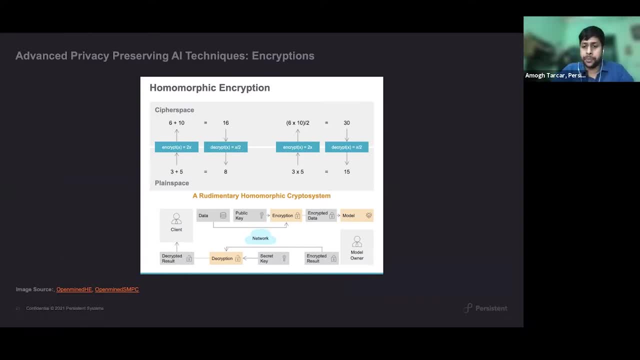 But at the same time cryptographically pretty difficult to do. So we think of plain space and cipher space whenever we are talking about homomorphic encryption and encryption in any general sense. So plain space is something where these numbers are directly available to anybody to see. 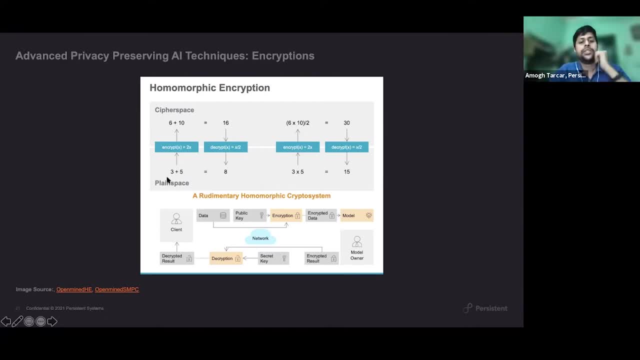 But just for example, let's try to understand that. Suppose we have some servers which are living in this plain space environment and they don't know how to exactly do addition. So we have a server which is living in this plain space environment and they don't know how to exactly do addition. 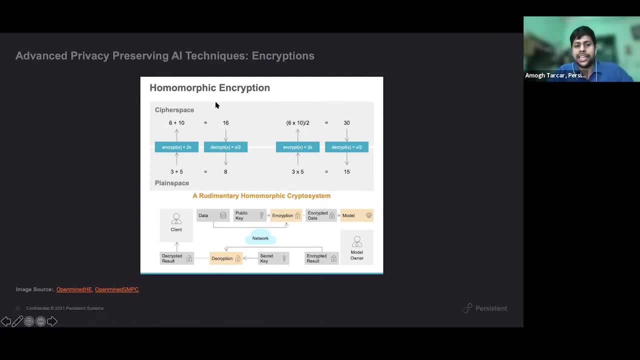 So they want another server which basically can operate in some other zone, which can do this addition for them, But they don't want to actually reveal this actual number 3 and 5 to this server, the third-party server, These particular two servers which are there, this 3 and 5, they want to do the addition operation but they don't know how to do the addition operation. 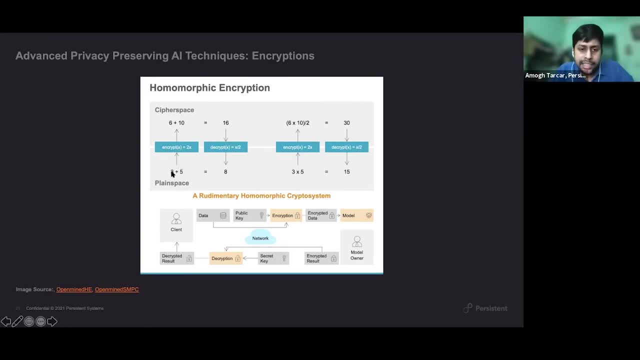 And basically they are also very apprehensive about sending this data in plain text And they don't want the cipher space to decrypt and find out what that real number is. So for the sake of explanation, in a rudimentary system you can say the encryption is 2 times x. 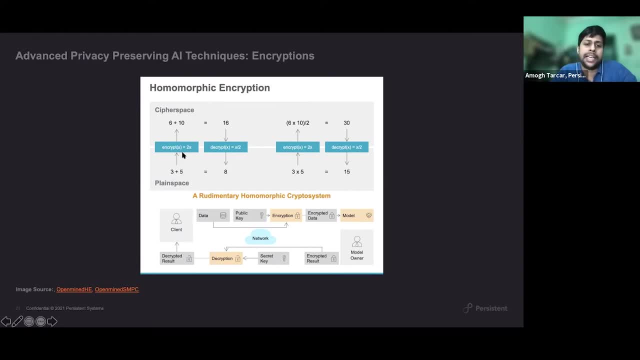 So every time you go from plain space to cipher space, you just multiply the number by 2.. And this encryption scheme is only known to you, So only you know that you need to multiply it by 2.. But the cipher space doesn't know that it needs to be multiplied by 2, or what exactly is the decryption? 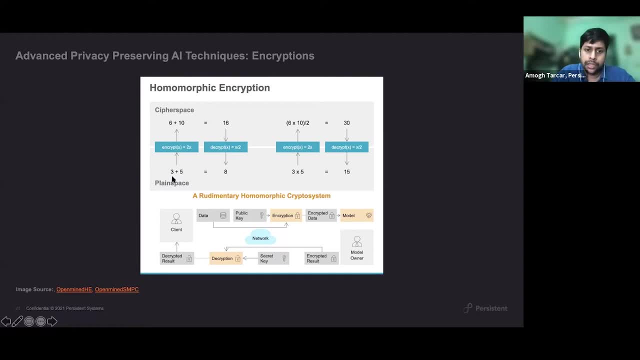 Which needs to happen in the cipher space. So what you do is that you encrypt this number and you send it to this other server. So you encrypt the number 3, it becomes 6, you send the 6 to the cipher space. 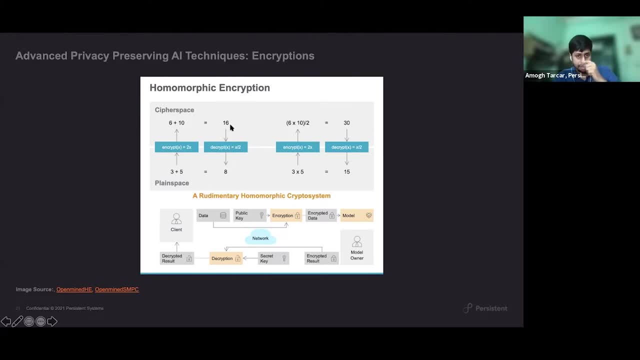 You take number 5, you encrypt it. it becomes 10, you send it to this cipher space. Now the breakthrough of why homomorphic encryption schemes are better than other encryption schemes is that Normally, when you try to apply any kind of encryption scheme, you don't have to worry about it. 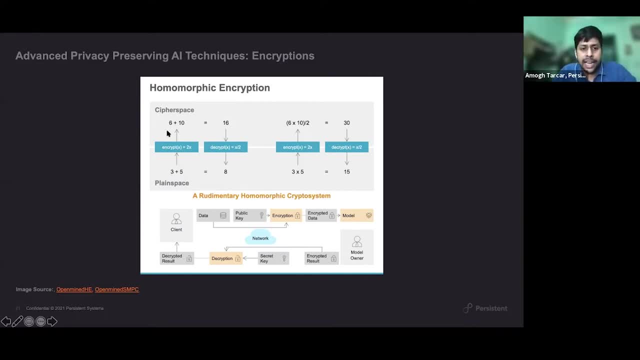 Normally, when you try to apply any kind of encryption scheme, you don't have to worry about it. For example, with cryptographic encryption, the end result is kind of a hash, which is most often times not really useable, Whereas when you do it using homomorphic encryption schemes, this end result is still useable. 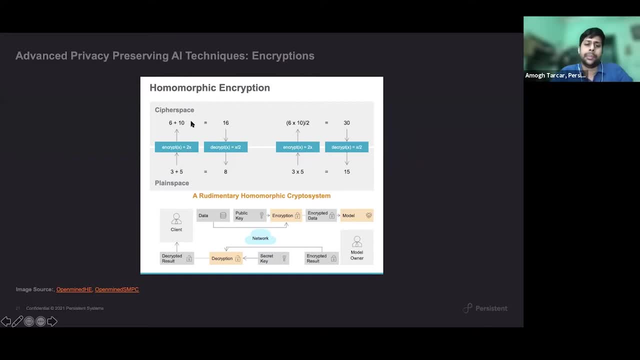 You can do certain mathematical functions with it, like addition, multiplication, etc. And that's what basically makes the homomorphic encryption really powerful. You go to the cipher space, but still some operations can happen in cipher space. And you can go to the cipher space, but still some operations can happen in cipher space. 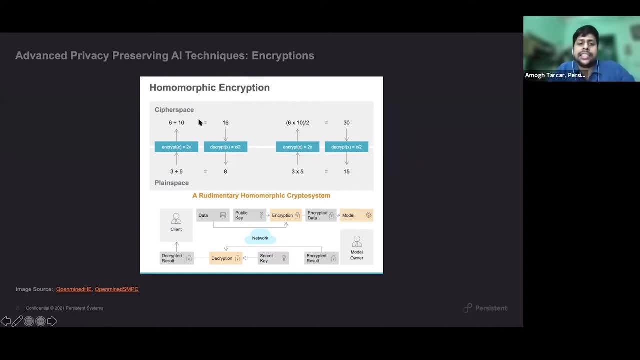 And you can go to the cipher space, but still some operations can happen in cipher space, happened in cypher space. So in this case, these two ciphers are being added by this server And the answer is 16.. Again, the server doesn't know what exactly 16 decrypts to. 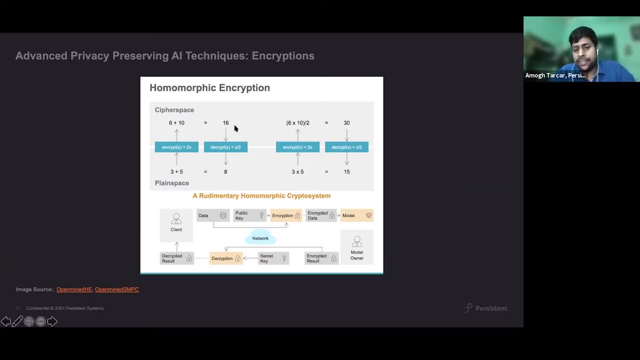 So this server is basically just doing the operation and giving you back that result, And when you get it back you kind of know the decryption. So you do it and you basically get your actual answer. So, in this sense, what you did was that you actually got the 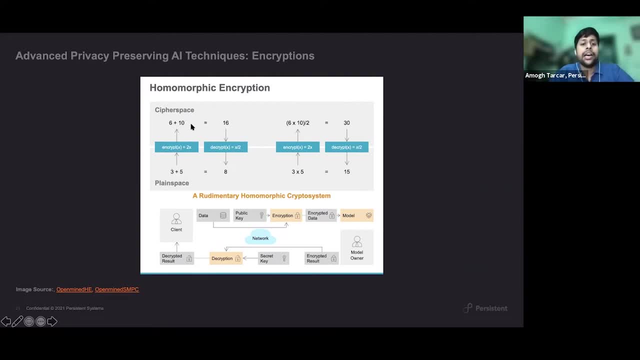 operation done, but you did not reveal the numbers three and five to the server, which is operating in cypher space. So this has lots and lots of advantages basically, And if you try to apply it to some sort of a machine learning system, then basically you know. 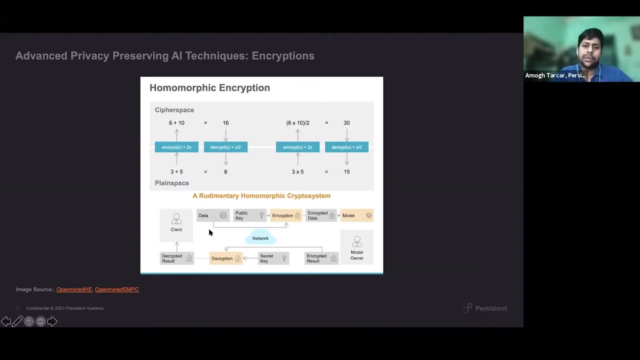 you can. essentially, this is something which actually has been happening as well, with some sort of structural data There are. there are startups which are doing this at scale, So what they say is that you can homomorphically encrypt your data and give it to us in this particular 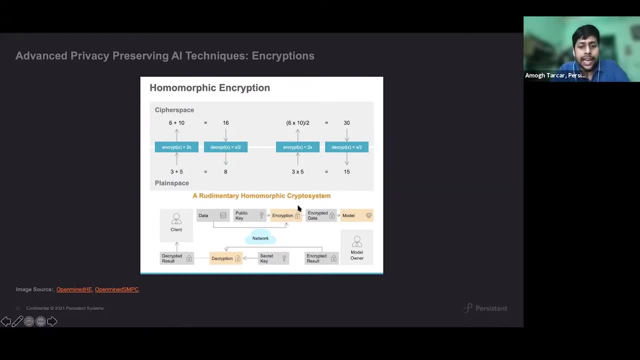 cypher space And in that cypher space we will use this encrypted data and we will train a machine learning model just by. you know, using this sort of homomorphic encryption, you know kind of operations we can actually make a model out of it And we will keep that. 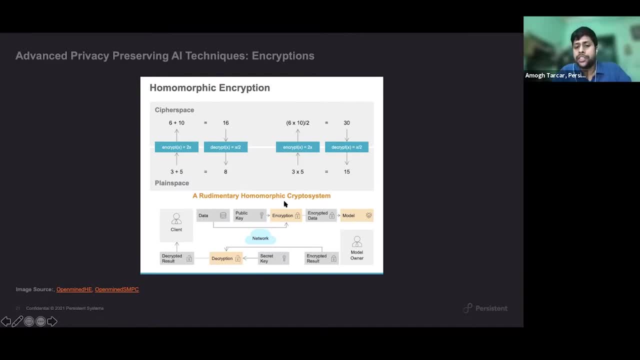 model. So basically, your data was sent to the server, but in encrypted format, and using that encrypted data, the cypher space server basically could actually train a model on this encrypted data And then later, whenever you want to use it, you can basically again just send your data. 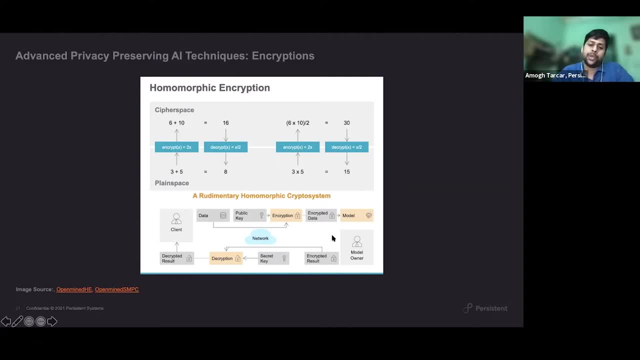 to the server. the server will do the prediction again, the output will be encrypted and that encrypted result will be sent back to you and only you know the decryption there. So you can decrypt it and then you can come to an answer. 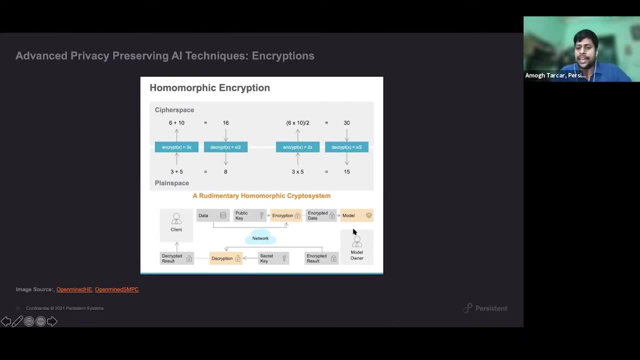 So essentially, you're using a server like, say, something like AWS or Azure to do your actual machine learning, but that server learns nothing about your data And that's kind of you know, a golden scenario when you. that's very desirable as such, But this basically. 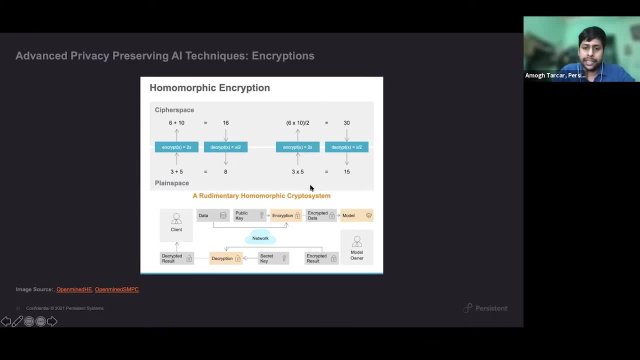 comes in with multiple challenges and so on, But this is a concept. This is a concept of homomorphic encryption. basically allows you to do operations. You can do operations in Cypher space And, based on what sort of operations can happen, there are multiple. 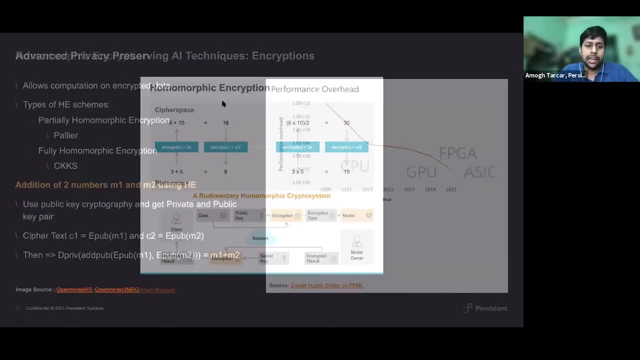 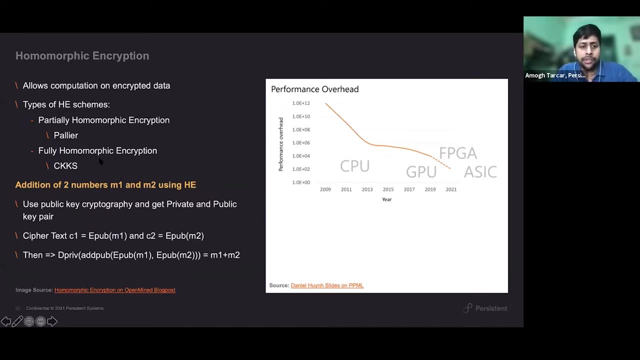 types of encryption schemes. There are some partial encryption schemes that are fully homomorphic encryption schemes. So what is the difference between partial and fully is basically the type of operations that actually supports. So a partial homomorphic encryption scheme is a Pehlier scheme, which was kind of introduced way back until around 1999.. And Pehlier scheme basically allows you to run a process of spitting information over no one's data. You can send it to someone or you can send out it to someone else. it's not just for your data, to see if you have access to it, So you can use it without any. 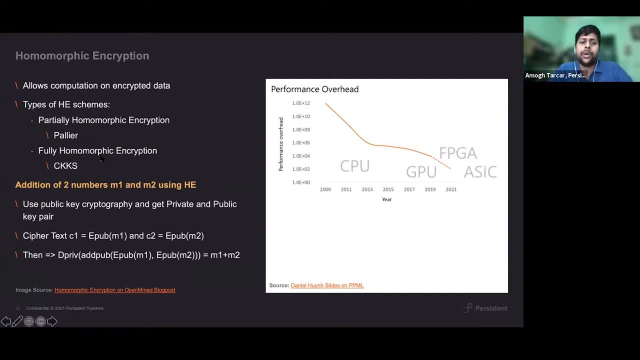 kind of problem. You can send it out to someone else and you can sort of find it with a password. you can send it to them, you can send it back to them, you can send it to the person you're to do, just addition, And fully homomorphic encryption is like the recent scheme, I think. 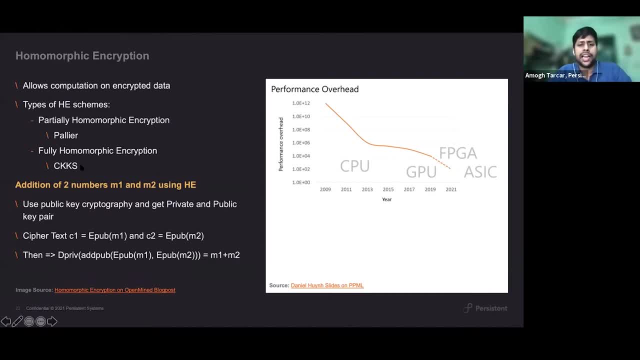 so Gantry, in around 2009, formally introduced various techniques of doing fully homomorphic encryption, And one of the very popular schemes for doing homomorphic encryption is CKKS, which actually allows you to do addition as well as multiplication and then so on. So, using 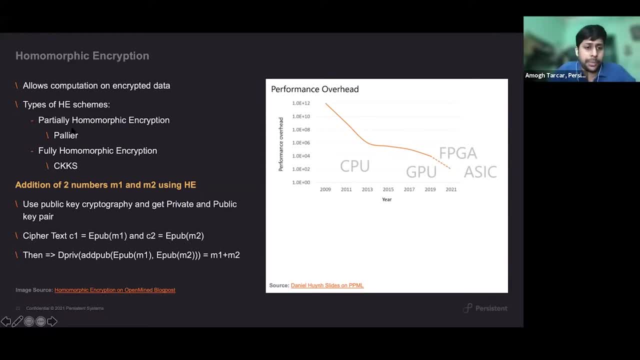 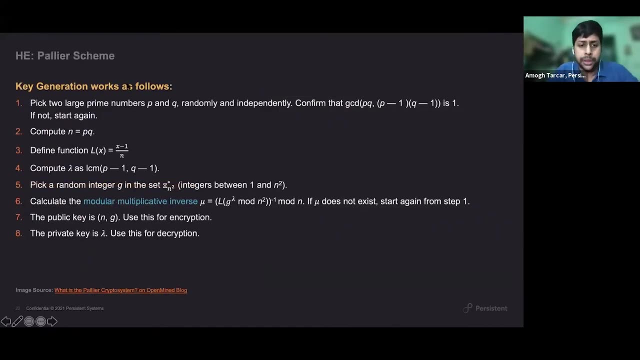 these kinds of techniques you can do operations in the cypher space and people have been trying it out in various ways. So we can actually try to take an example of how can failure scheme be used. So I'll kind of just- I'll not explain the full mathematics here, but 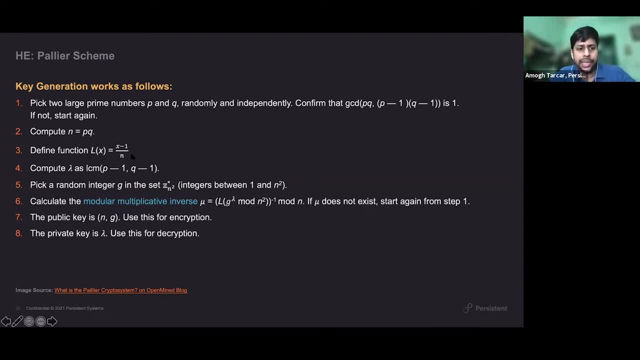 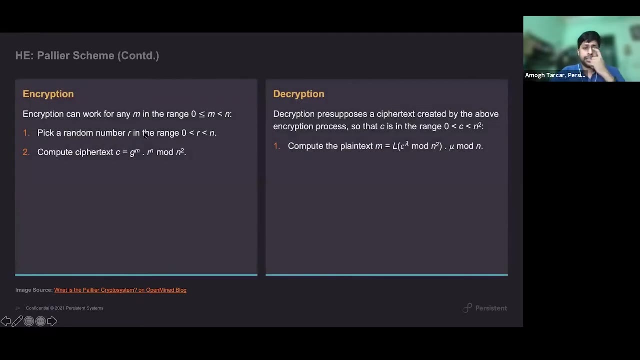 essentially, this is the scheme. this is the way you can actually get hold of your private and public keys. So you keep your private key with wherever it gets generated, and public key is something which can be used for encryption. So this is how encryption can work. You can pick some. 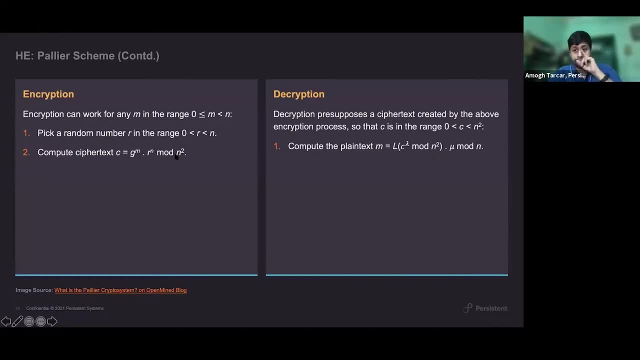 number which is, say, you know your message is M and you want to encrypt it, Then you can go to ciphertext using this formula in failure scheme. So with the ciphertext, basically you get your actual ciphertext, You can pass it on to the server which can do these operations on ciphertext, such as: 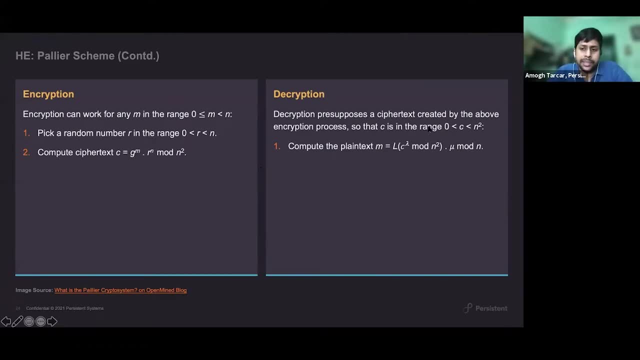 addition, And when you get the answer back, you need to run this set of mathematical operations on it to actually get your model M or your message M back. So using this and explain the math behind this is actually beyond the scope of this session, but I would encourage you to read about it in these blogs and try to understand. 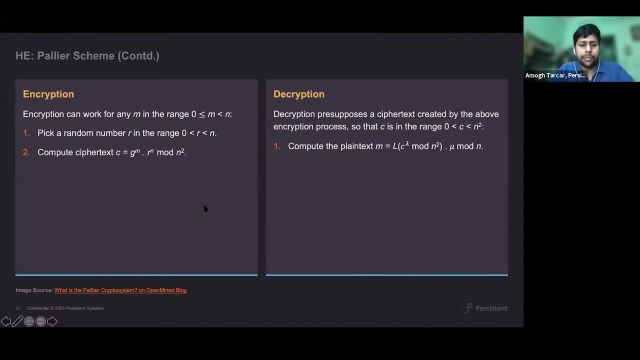 more of how exactly it works. So that's it for this session. If you have any questions, please feel free to ask them in the Q&A box, And I'll see you in the next session. Bye, Bye, Bye, Bye. 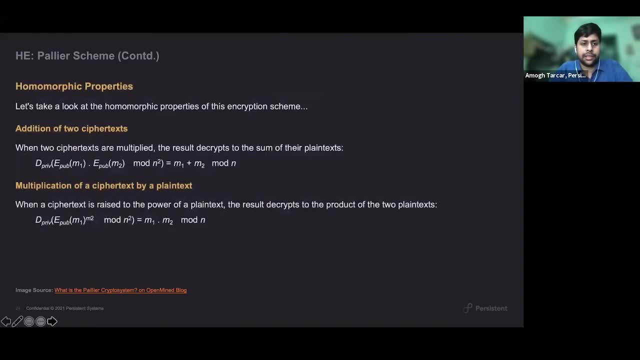 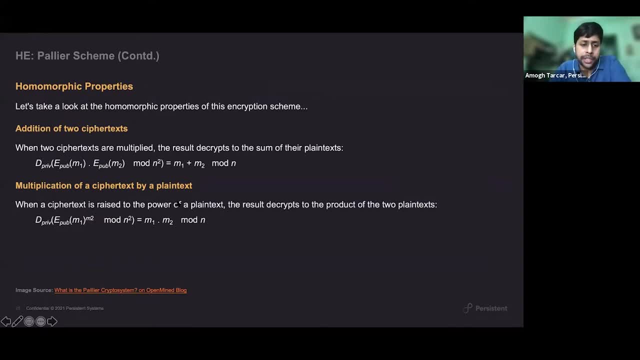 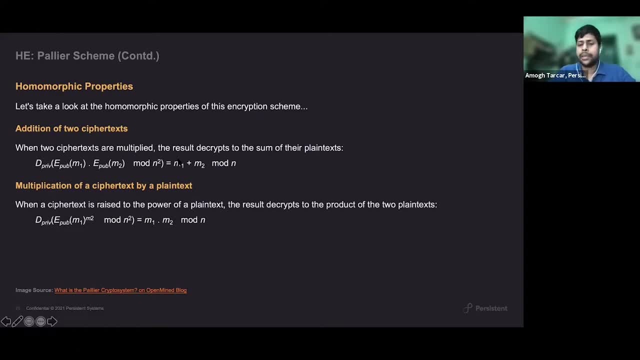 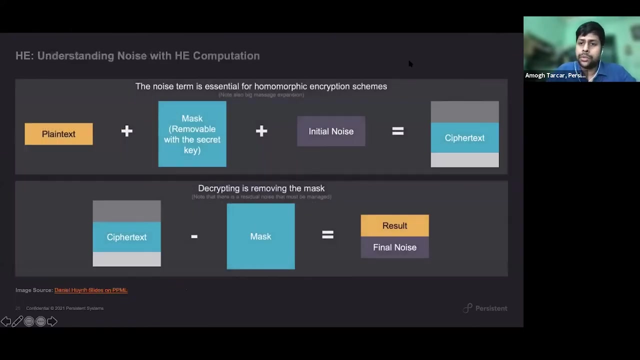 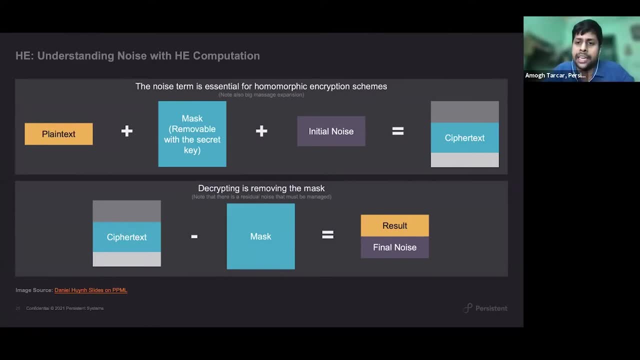 It's like so: in failure scheme we did not see the noise factor coming in much. But when we go to other schemes like BGV or CKKS and so on with homomorphic encryption, comes a little bit of noise every single time you try to do some computation. 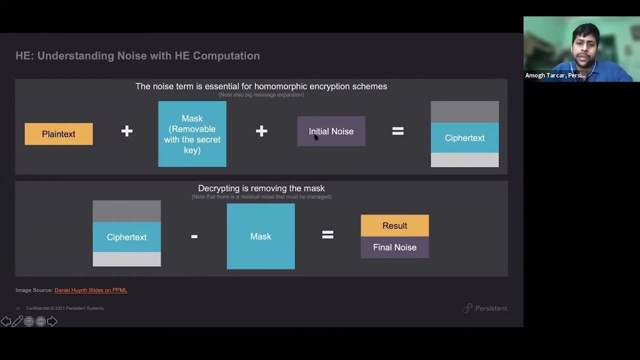 And the way to understand it in very simple terms is something like this: You have some plain text, you add this heavy mask on it and you add some initial noise to actually get your ciphertext. The ciphertext is something which you know. in cypher space, operations can be done and you're given the ciphertext back. 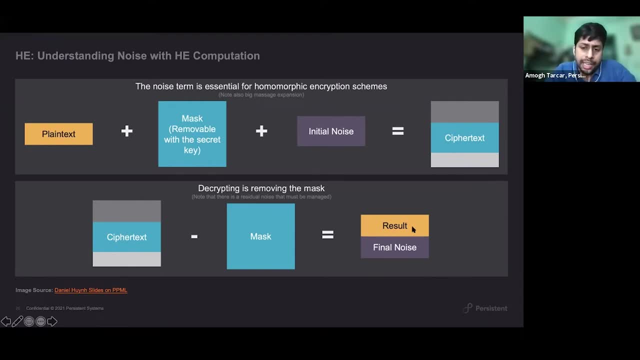 And when you remove this mask, the end result is the actual result as well as some final noise. So it's important to notice that there is some initial noise and there is a final noise, And that's something to basically remember when we're trying to do homomorphic encryption. 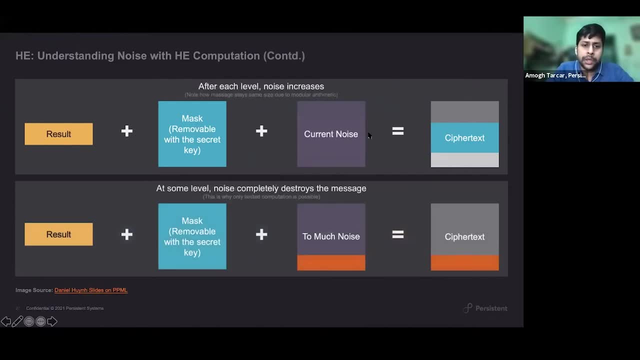 So In case wherein this particular noise, as you keep doing various operations in the cypher space, this noise keeps getting increasing, And if it actually increases even more than you know the mask which you're trying to apply, then what happens is that there's overflow and because of which you basically lose the end result. 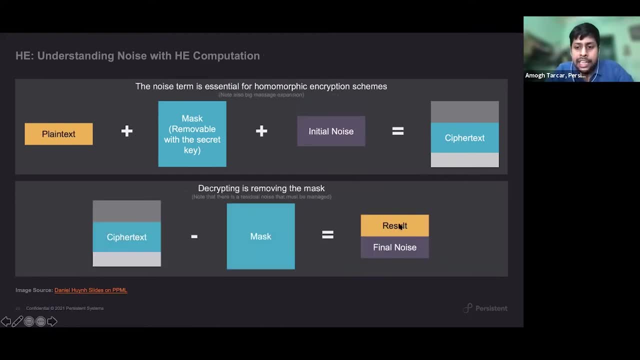 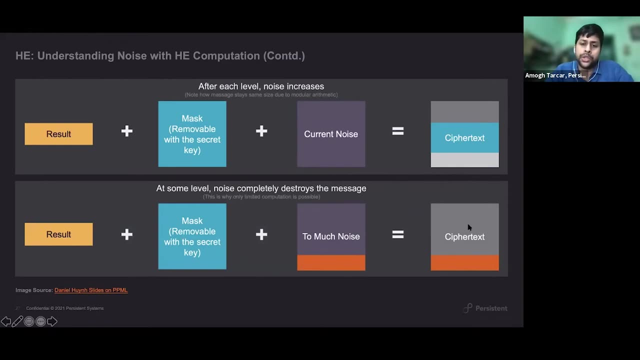 So ideally what you should have been getting is results plus final noise. But if this noise becomes extreme And it overflows, then essentially you lose your actual result and all you get is just ciphertext. So there are some sort of mathematical limitations of what sort of operations can happen. 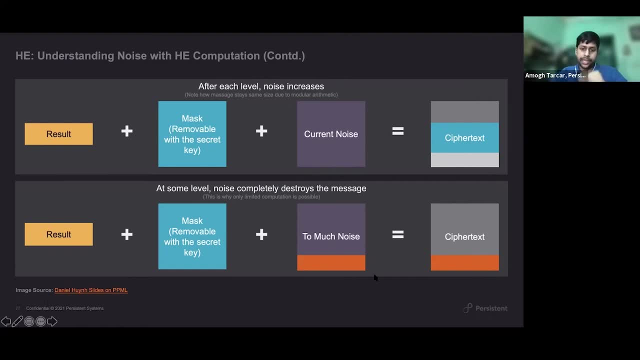 And you need to be more aware about this- noise parameters and so on- And, and you know, till the time you remain constrained in this environment, you're fine, You can actually do various operations, but there are scenarios when this sort of things happen and you have to be careful about it. 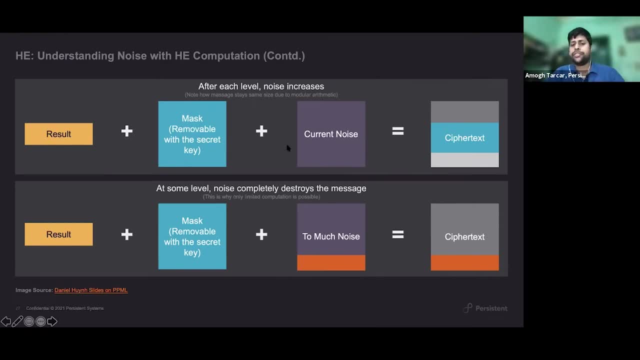 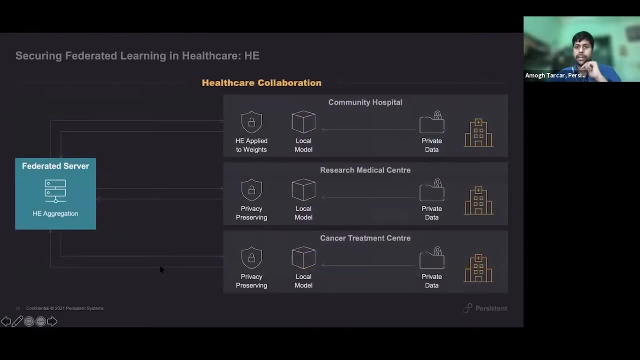 So and also this is something which is like this: This is sort of handled in these various schemes which is actually implementing all this homomorphic encryption, But we just need to be aware of such things, such kind of operations happening. In case you guys are interested, I have we can also try to see the actual homomorphic encryption code as such. 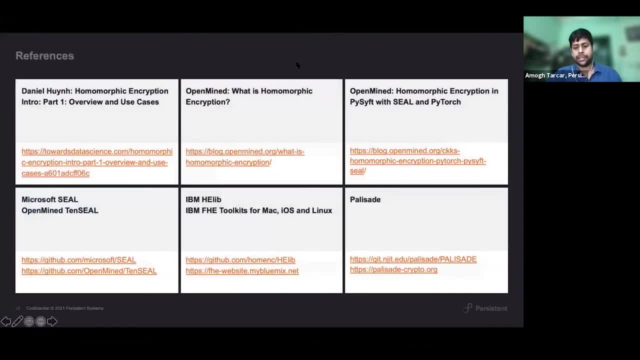 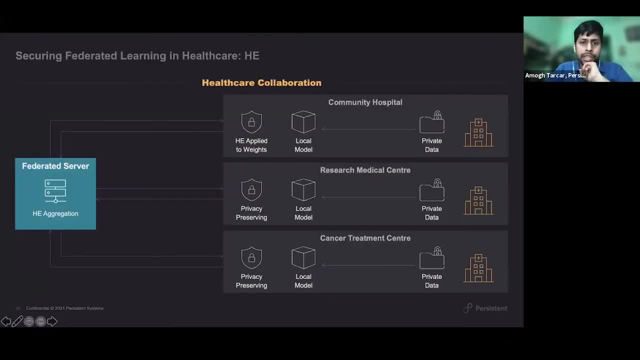 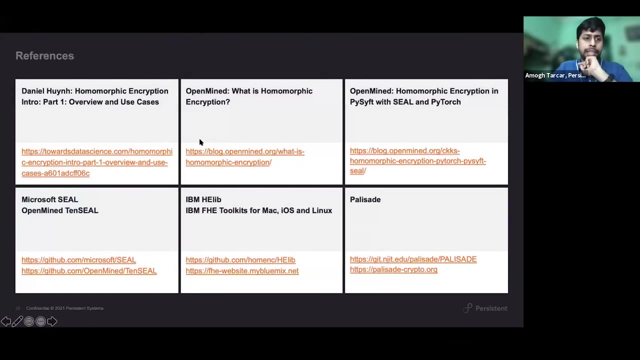 Or, in the interest of time, we can cover it up and maybe we can Get back to it later once we do the session. but so let me know about it in comments and I'll note it down, And then at the end of the session, if we have time, we can come back and see some code as well on that. 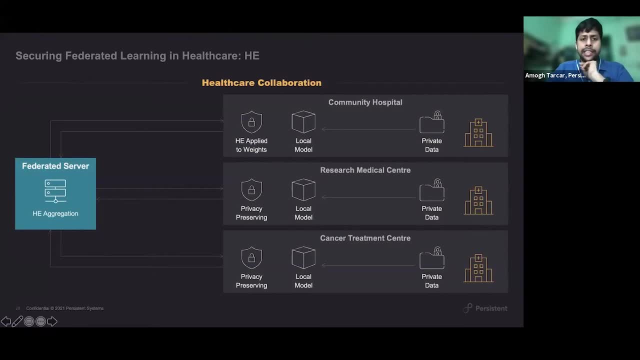 So yeah, how it applies to federated learning. So in federated learning you can basically so you there have been examples where you can actually Do homomorphic encryption on the data itself and you can ship it to the server and do training. 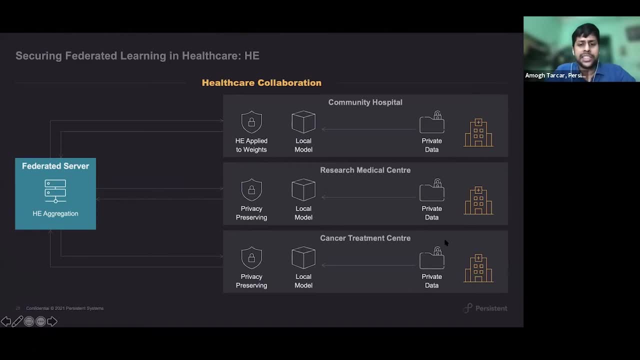 In normal machine learning. but that's something which can be avoided in federated learning, because you don't have to encrypt the data, because the data is not really leaving its source. So what you're more concerned about is the weight, is the local model, is training and actually you have to protect your weights. 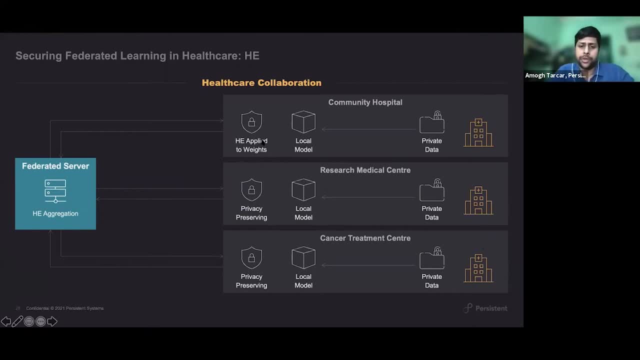 So homomorphic encryption can be actually applied on the weights, because if you, if you try to remember the, The fundamental concepts of federated learning is that that these weights are what is getting shipped to the federated server and in the federated server, basically they are just getting aggregated or some sort of operation is happening and 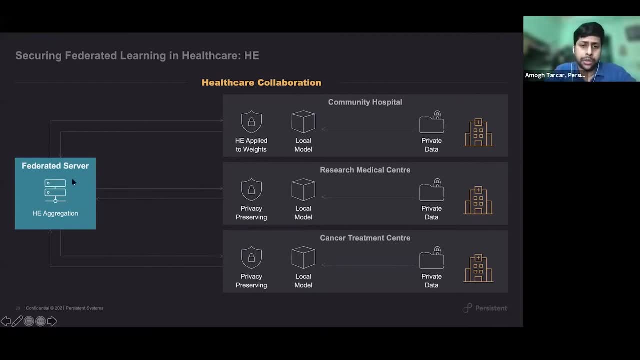 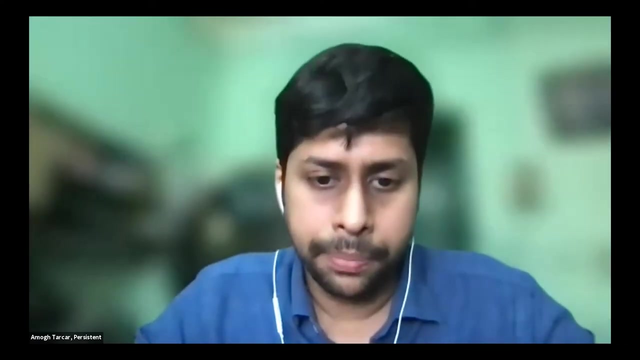 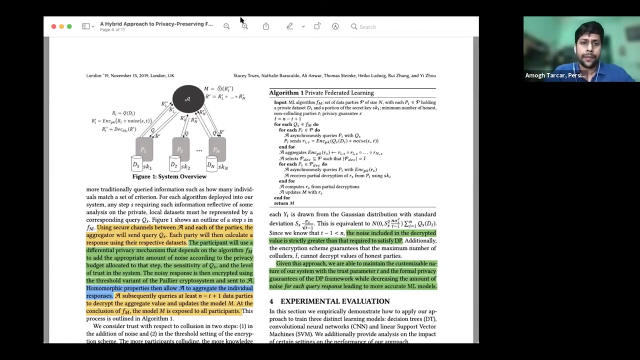 aggregation can be done using homomorphic encryption. So essentially, you can apply homomorphic encryption and you can do this federated learning in, or the fusion of these various weights in, ciphertext space. So that's where homomorphic encryption can apply here. Now to actually understand this more, I have a paper which is published by IBM. 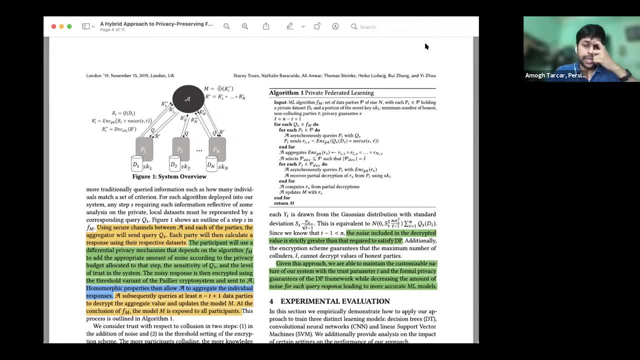 Okay, so I have noted down that we would like to see the code demo and we'll come back to it at the end of the session. Can you guys confirm You can see my code? You can see my screen which is showing a paper. 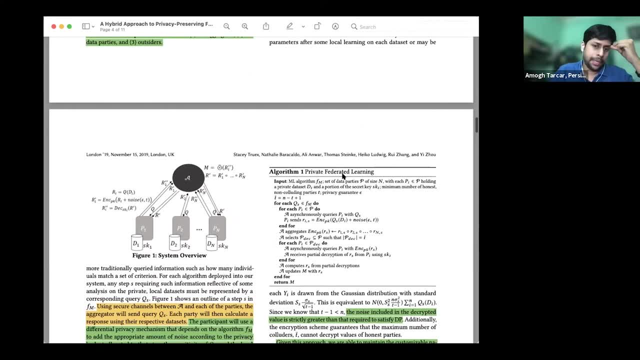 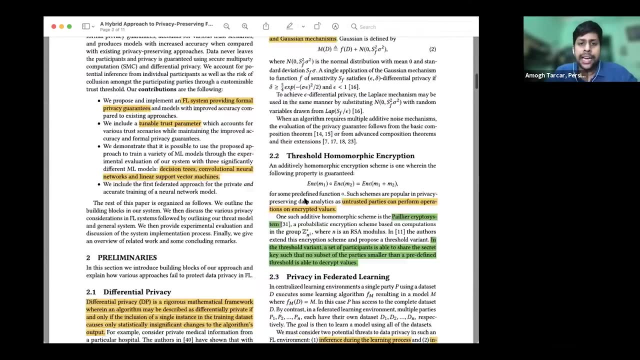 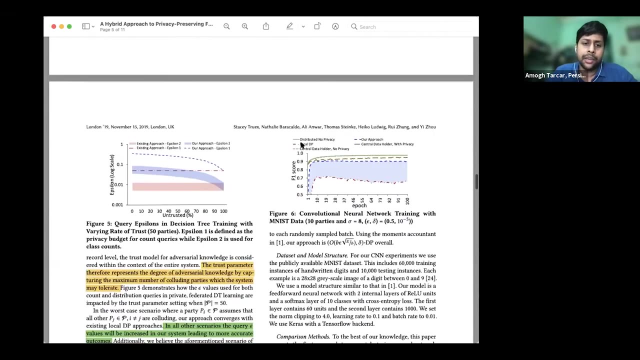 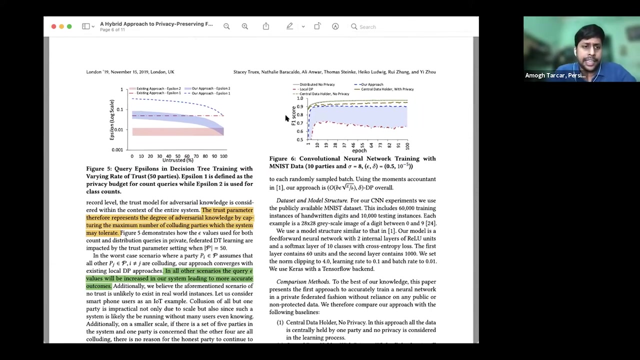 Okay, so this basically is an IBM paper wherein they have tried to. so basically, the problem which they found is that when we actually try to do machine learning or the federated learning in local DP mode, or basically trying to apply different methods, Right, They proved us that when people rely onlight access and they rely on theusethat they normally 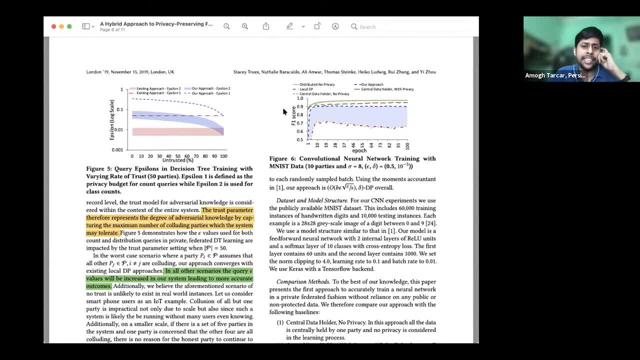 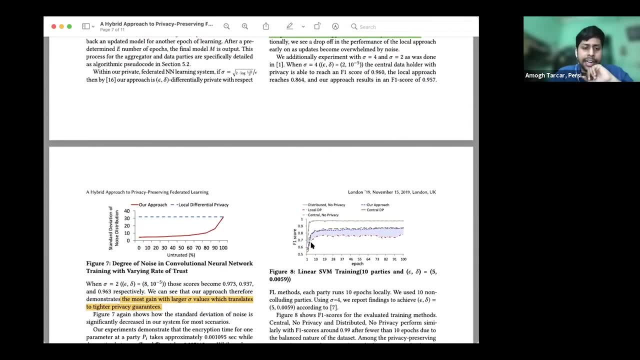 apply differential privacy to the weight directly. what they observed was that to achieve the same level of privacy guarantees, they have to supply a lot of noise, and when they apply a lot of noise, what they end up getting is that again end up getting a like: oh it's. 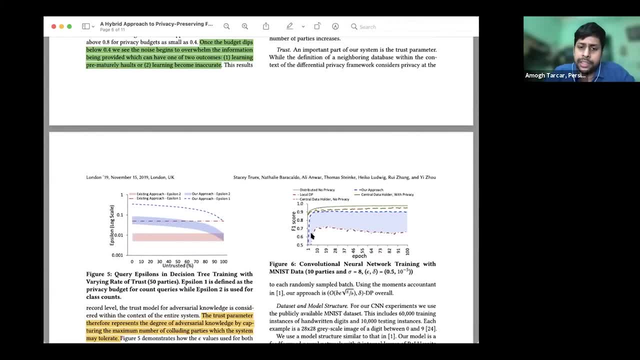 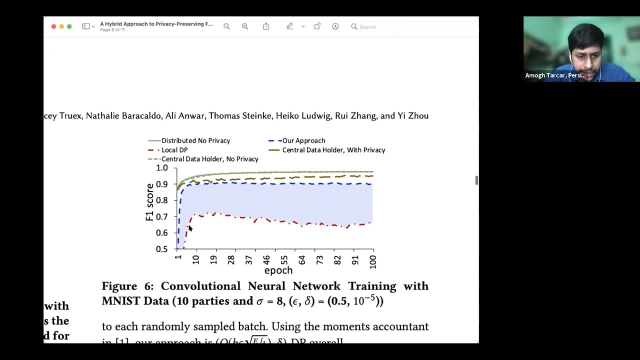 very difficult to train good models with that sort of a scenario. You can observe right here that you know, in the case wherein there was local differential, privacy is the red line and you can see the accuracy is kind of struggling a lot because you have added a lot of noise. so you are in around 0.7 kind of a range. and in case you had not done, 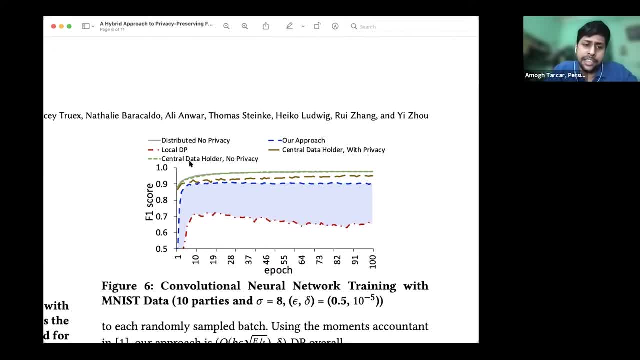 anything, uh like no privacy and a central data place. that is the green line over here which is kind of very strong, right so, uh, so that is the case wherein you have no privacy, and with differential privacy in a cross silo case, uh, you kind of see that there is a pretty big gap, which actually 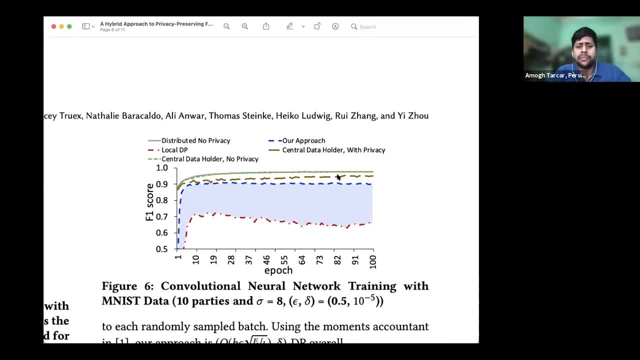 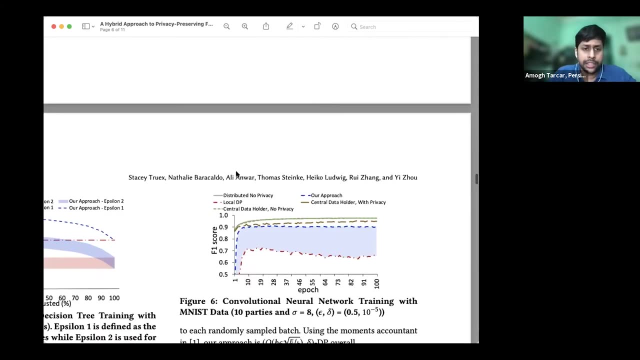 happens. so to basically overcome that ibm paper really applied, they combine these two things. so they do apply differential privacy to the weights, but what they do is that they try to do the aggregation in a homomorphic encryption space. right, so let's just try to understand what. 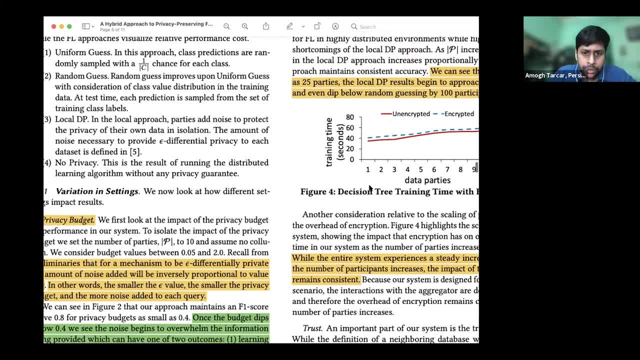 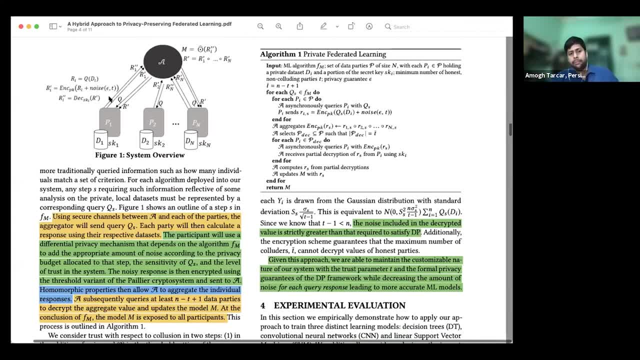 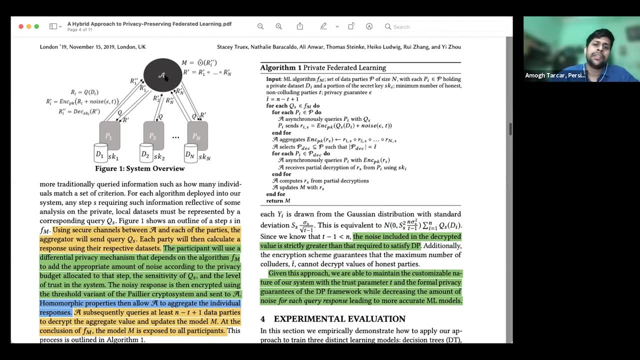 exactly they're trying to do. so this is basically their algorithm, which they follow. so what they do is that they compute this, so they compute these weights, which are the updated weights of the model, and when they are sending it to the aggregator, they basically uh do the public encryption or public key encryption of uh of this particular. 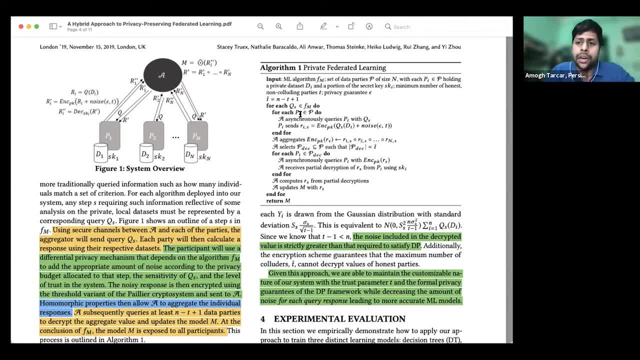 value of the matrix and send it to the aggregator. now, uh, one question you know you may ask is: uh, in this setting, because there are multiple parties, who exactly is holding this private key right? so, uh, the the common, the normal, like the first level homomorphic encryption of failure scheme cannot be applied directly over. 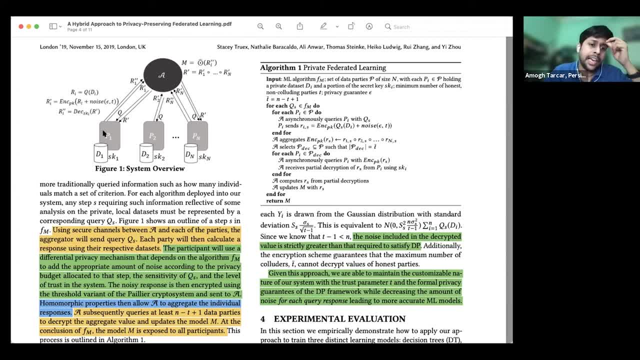 here, because if you want to apply directly you have to share the private key between the parties. and if you share the private key between parties then you know each party can actually interrogate and try to get something out of the end result. so it's it's kind of not. 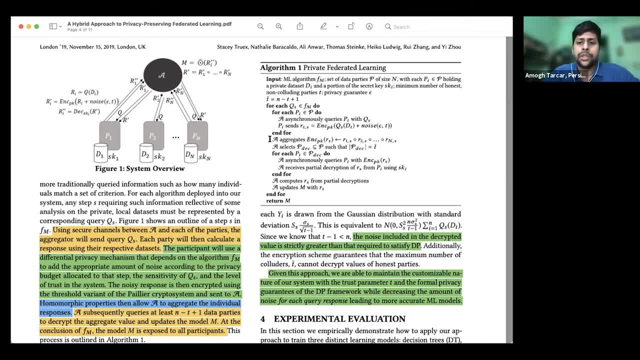 recommended to have the same key across multiple parties. so for that, uh, what they tried to do is they found a variant of this failure scheme- it's called a threshold variant- wherein, instead of a just having one key, what you get is that you get a set of keys, a set of secret keys. when you try to 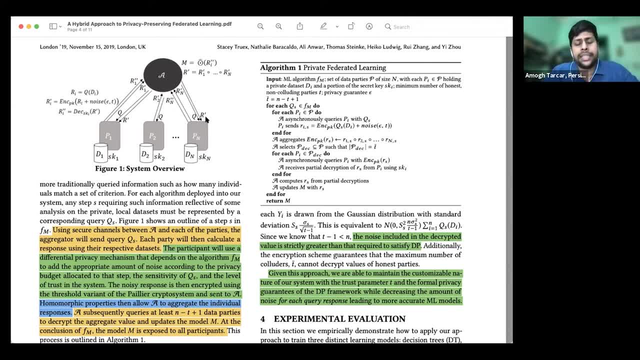 do homomorphic encryption, so you basically get one public key but say you get 10 private keys and these 10 private keys can be kept with various of these parties. so each of them gets their own private key. but what's important is that this is the threshold variant of the paler scheme. so this: 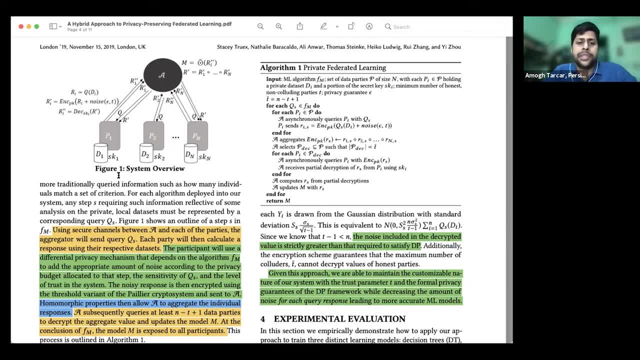 each key is, on its own, not able to decrypt the full encryption. so what you do is that you you have these 10 keys, but they are called partial keys, and then there is a threshold, which is a minimum number of keys which have to come together to basically do the decryption. so in this case, 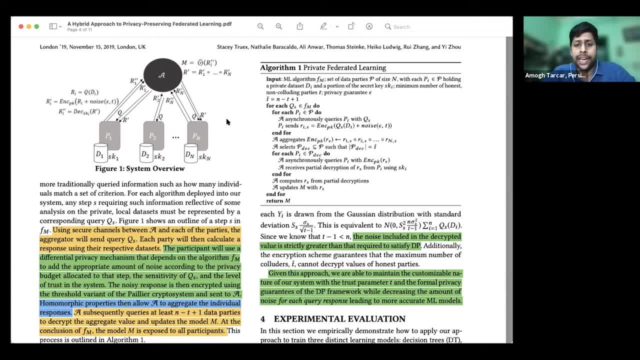 say, the number of keys which have to come together to do decryption is five. so you have 10 partial keys and at any any point of time, if you have decryptions from five, then you can put together and get the end message. So that's what happened in this example. where. so what they do is that they get their weights. 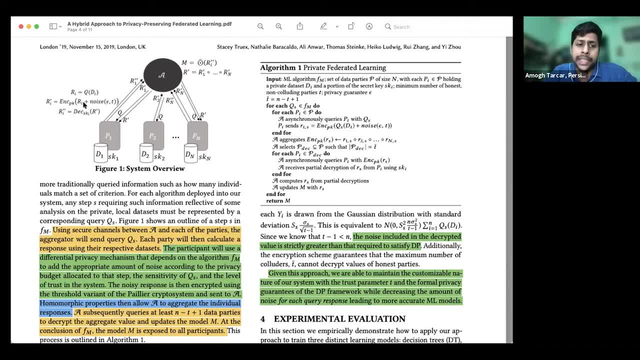 they apply encryption on it. they do apply differential privacy on these weights so that in any case, if that gets somehow leaked, then they want to protect it. so they do apply differential privacy and they send it across to this aggregator. now this aggregator basically computes the aggregation and it has this, so over here it has this something called as encryption. 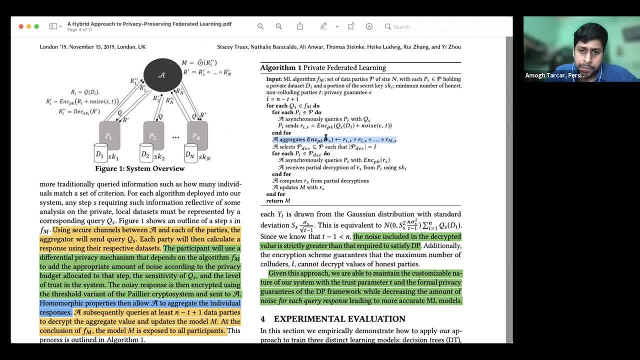 of the result rs. So this is the result of the encryption, and it has this something called as encryption of the result rs, And this is a public key encryption of the result. now, what it does is that it cannot decrypt it because it doesn't have the private key, so it sends it to this partial decryption. so, basically, 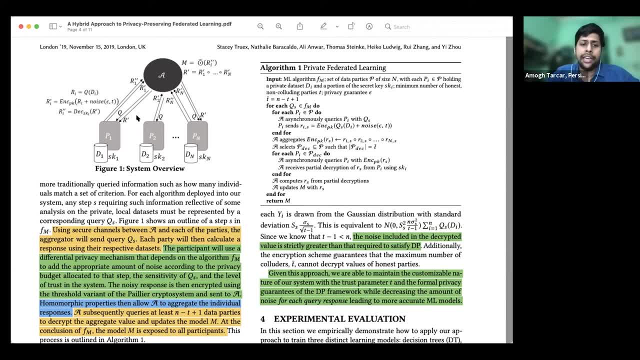 what happens is that this particular encrypted result is sent to five of these ones, who, each one of them, does some partial decryption and sends that partial decryption back to the central aggregator. so if you receive five partial decryptions, you can basically combine it together and you can. 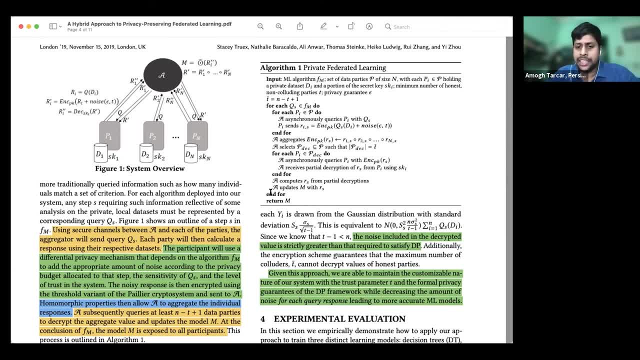 get your answer, which is the final aggregate. so basically, the actual weights in the aggregate are revealed to this aggregator and it puts together a new model which is again shared between all the parties and the federated. learning continues, but most important point to note over here is this aggregator learns nothing about individual parties weights. so those 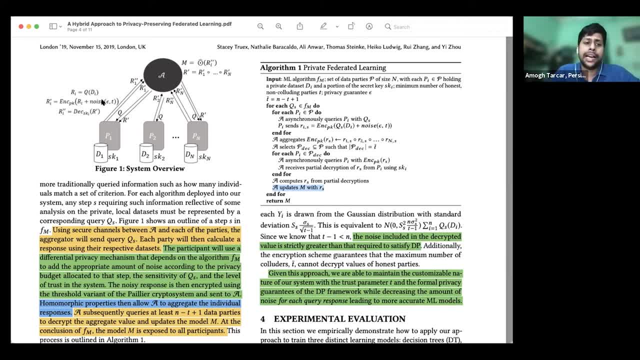 weights are completely protected, first level by differential privacy, in the second level by homomorphic encryption. so with this, both schemes together, we have pretty good, you know, grip on trying to protect the privacy of the end users here, and the aggregator just does aggregation and can reveal only the aggregated result, which is pretty good. so I would encourage. 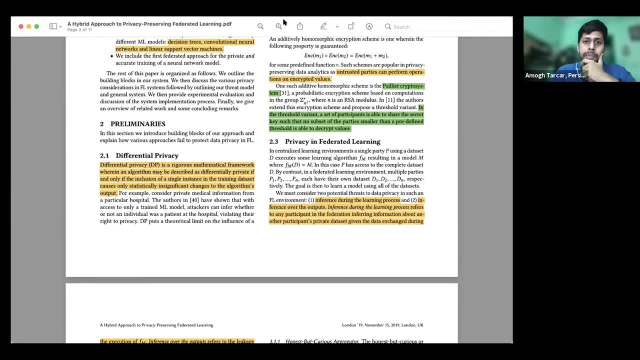 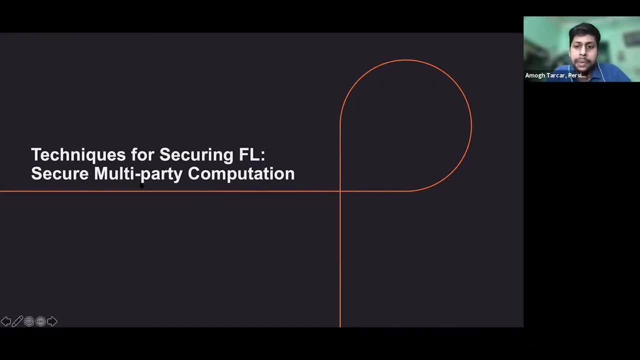 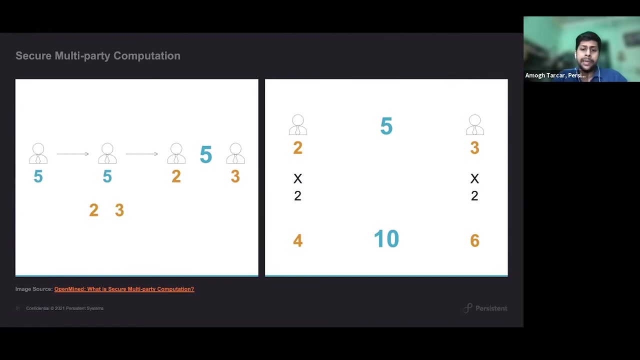 I have put the link of this paper as well. I encourage you to read through this paper. so the next session basically is a secure multi-party computation and this is kind of an alternative to homomorphic encryption, but with a slightly different twist. so this is basically how a multi-party computation can happen. 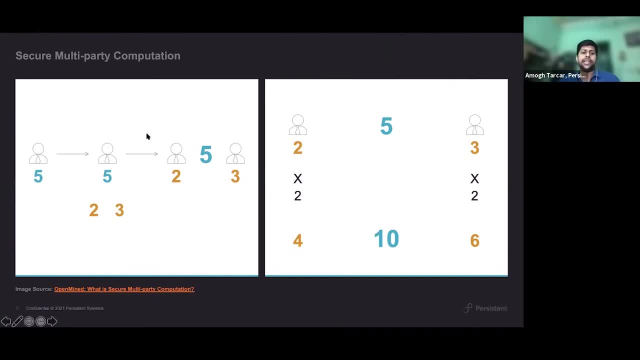 so in homomorphic encryption, what we had seen was that we basically wanted to kind of keep the as in do some operations on a number without actually revealing that number out to other parties. and in this case what we do is that we try to keep the same number encrypted between two parties. 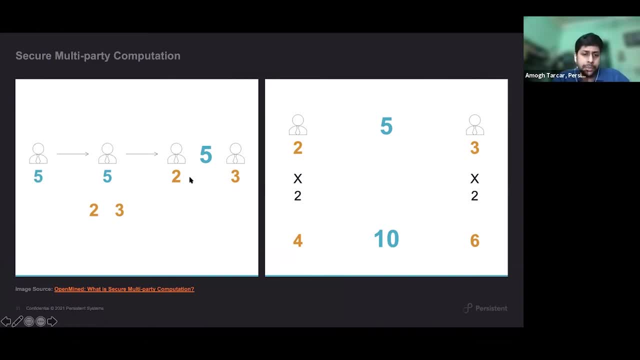 but what we try to do is that we basically divide that number into shares. we basically say we want the number five divided between two people. we can keep it as two and three and individually. we basically make sure that these two parties cannot talk to each other and if it is just this party alone, that party cannot come to know what the full number is. 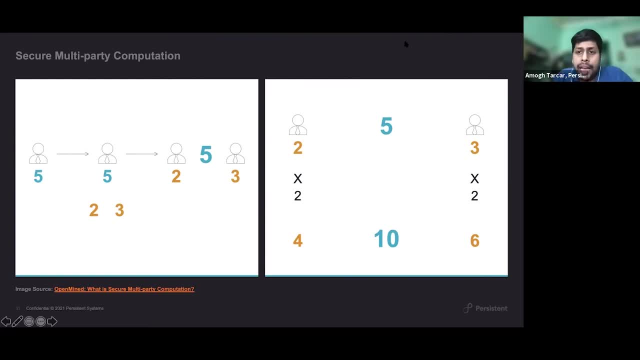 all that the party knows is that the number is just three. and in case you want to basically ask this, do some computation in this sort of encrypted way. what you do is that you tell both the parties to say you know you want to get this number multiplied so by two. then what you do is that you tell each of these parties saying individually: you: 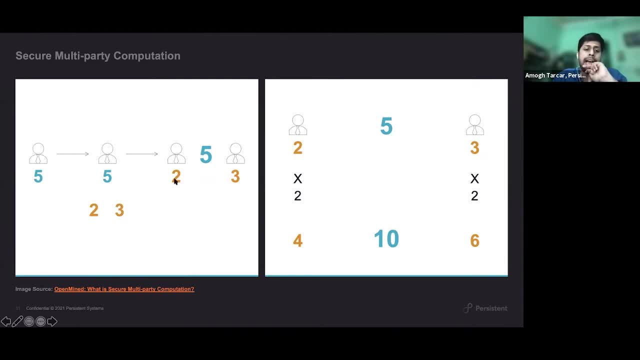 just go ahead and multiply the number number you have by two. so what they do is that they multiply their each number, which is like four and in this case, six, and what you get back is you just get that four and six, and this parties individually don't know. basically, all they did is: 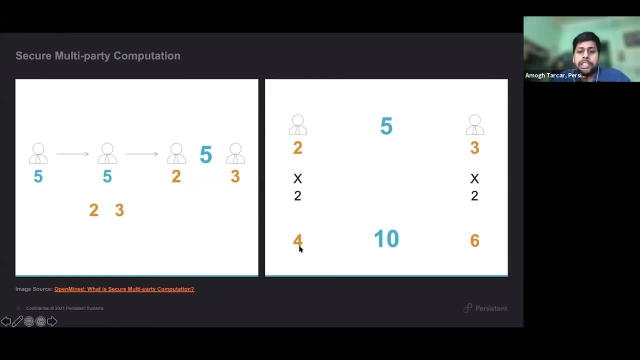 that one operation which they were told to do. but they don't know the bigger picture of what that number was, and only you know that the number was five before and now the number. when you add both these things, you know that the number is 10.. so you got your computation done, but individually. 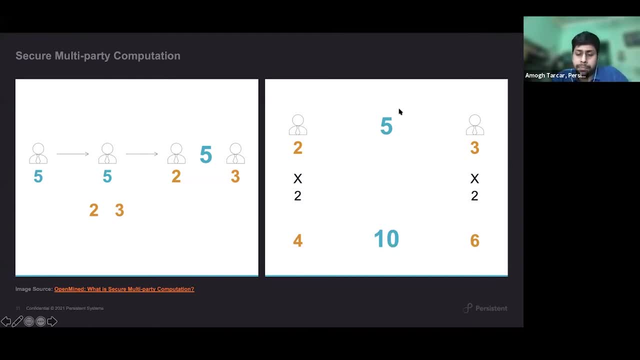 these parties learned nothing about the final number. that's basically the. that's the. that's the way you know multi-parties can do it, and that's basically the way you know multi-party computation can work. so, instead of using uh cryptography and try to go into cypher space, 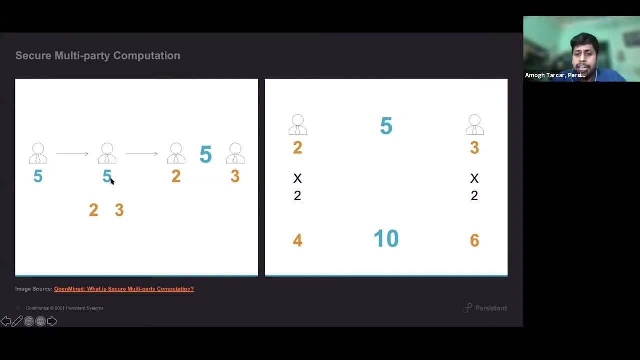 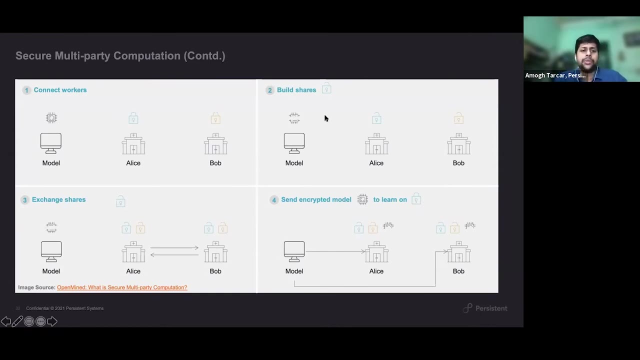 what you try to do is that you try to split the numbers which you have into shares and you want to send these shares to individual parties and then tell them to do certain operations on these shares. and uh, the same thing can you know, can be extrapolated to try to do machine learning in the 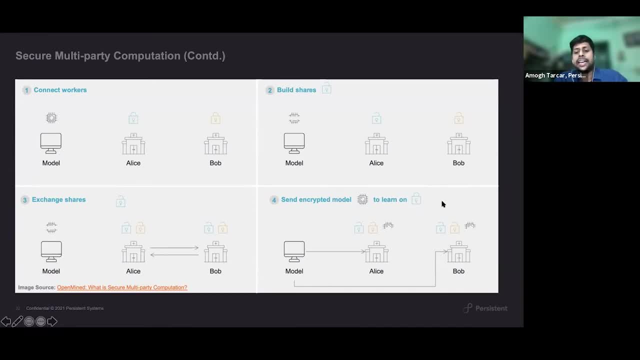 same way. so you know- and this pretty basically, this diagram combines a lot of concepts together. what you can imagine is that if you just have the data and you have these two parties, you can actually split the data between the two parties, and that's one way in which you can keep the data. 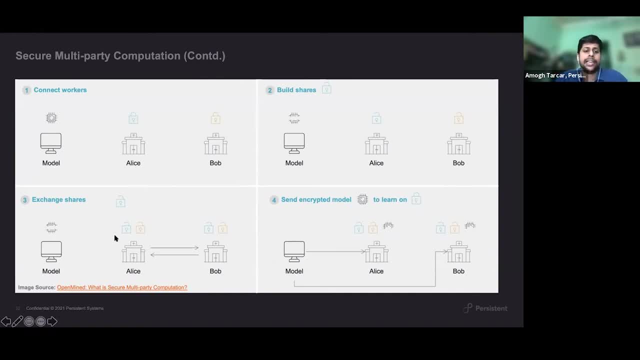 shared between two parties, but for individual party it becomes completely encrypted. now the model also which you have can be split and can be sent to these both parties. and then you have to, you have to devise a technique wherein you want to actually do machine learning or say stochastic gradient descent or, like you know, actually break the 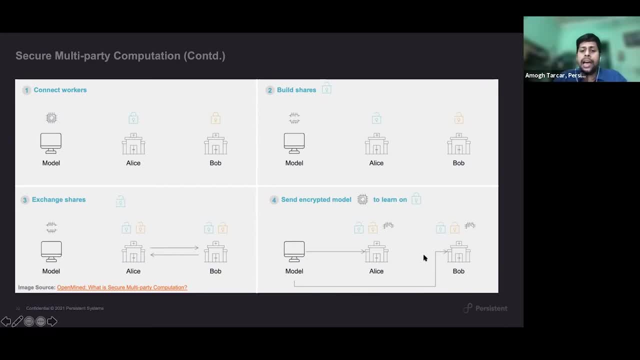 data into multiple parts and then you have to do some sort of a mathematical function, you have to do operations like relu and matrix multiplication when the data is actually in this sort of a format. so that requires a lot of protocol level changes and so on to basically achieve that. 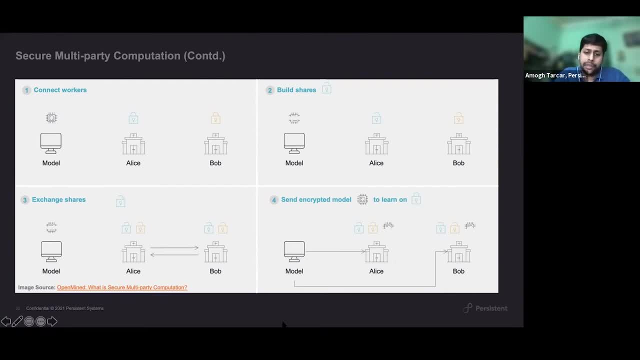 but this is a clever way out and one of the main reasons why this is, you know, gaining popularity is because, uh, it increases the number of, you know, network calls which need to go between multiple parties doing the same computation. but it is not that very cryptographically heavy as such that in homework encryption the amount of 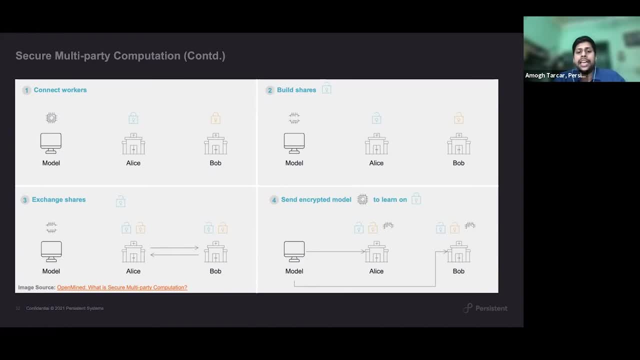 you know cryptography you need to apply. it is to become a very heavy computational load, whereas in this case, uh, what we do is that we split it between parties, so the network calls increase, but still it's. it's a scheme which people like because it's comparatively simple. 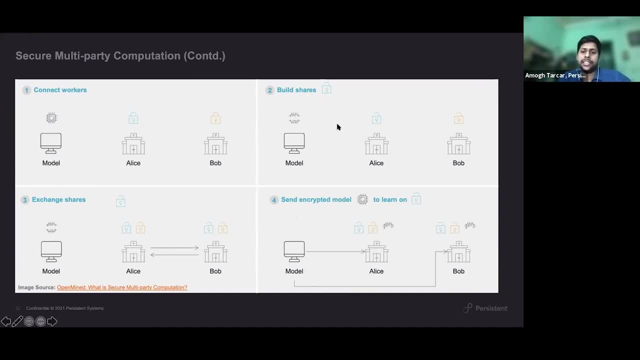 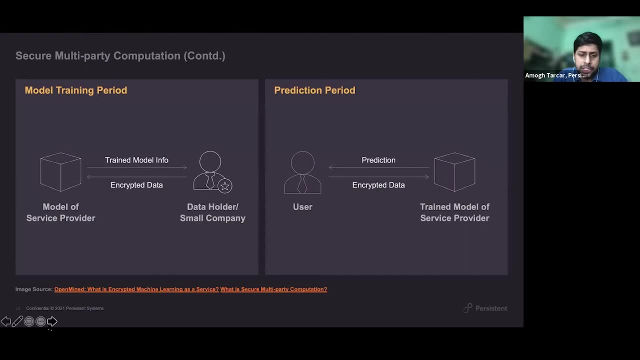 to divide data into shares and actually execute machine learning in that sort of a way, and early implementations of this has been actually put out, even by azure, and so microsoft is very big on multi-party computation, and so the first thing which they have come up with is: 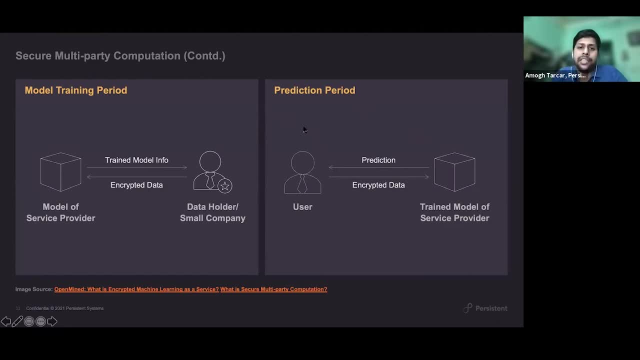 basically, uh, they have come up with a compiler level you know solution which you can just simply send your model to them, and they basically distribute it between a couple of servers, and what happens there is that they basically offer you, uh, encrypted model as a service. so what happens is that your model basically gets split and it's 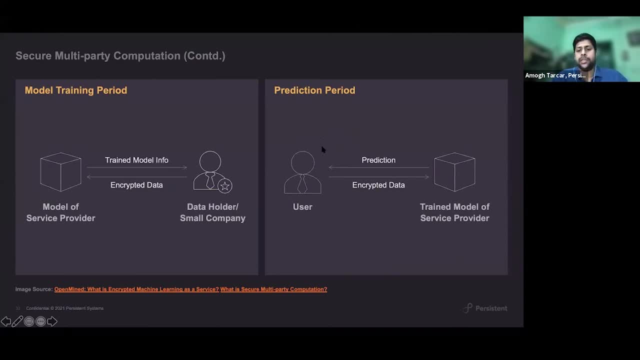 actually put out on different machines and, uh, you know, they have a specific way in which your data also has to be split and sent to all those various machines and you can actually get the partial prediction from each of those servers. you give all those partial predictions back and when you 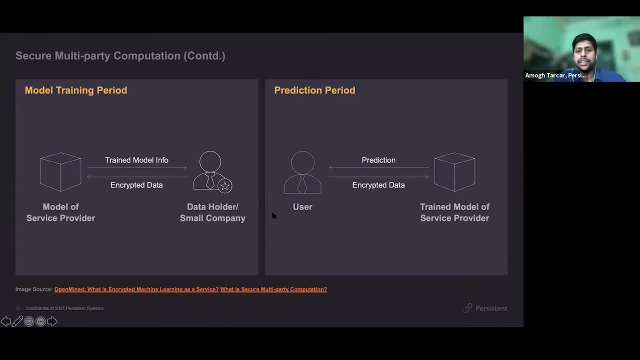 put it together, you get your encrypted result. so, uh, that's a very clever way in which secure multi-party computation actually can be used for proper machine learning, inference or training. uh, i think it's uh, secure inference. that's what the service was called in in azure terms. 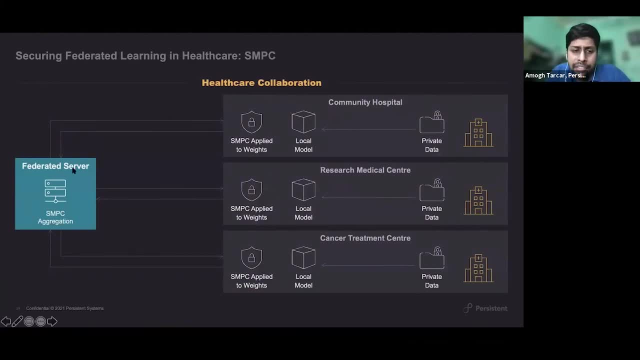 so, uh, we are not taking a deeper dive at how exactly smpc goes on, but you're free to read more about it and open mind as well, as on microsoft, azpc, and so they have some open source libraries as well. they have invented a crypt, tf. 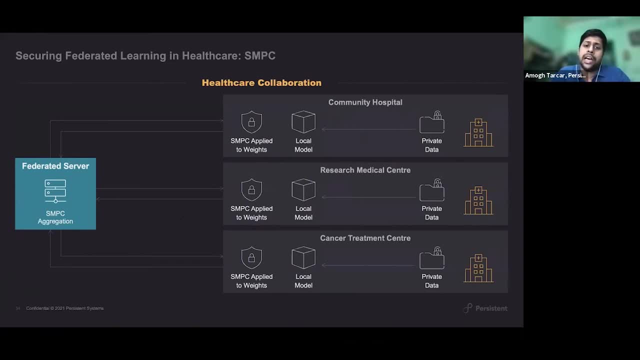 flow, so crypt, flow, secure, and then various protocols which actually allow you to do machine learning. in that case, but specifically to federated learning, what's important is that you can again keep your local models and all that exactly as it is, and you can basically get to this weight matrices and those weight matrices instead of, like earlier, you were applying homework. 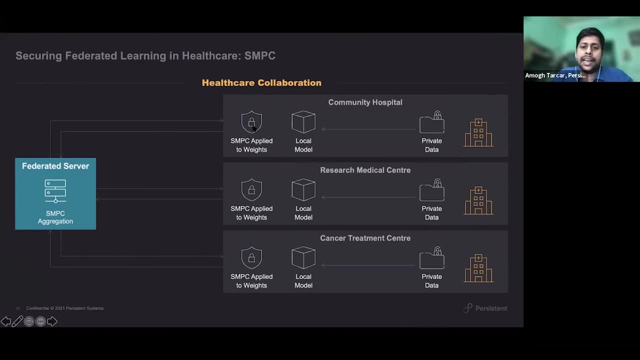 applying differential privacy. instead, you basically can form a collaboration between these various parties and split this matrices across different parties, and then there could be, you know, a central protocol controller which actually can get this operation done without each party and knowing you know what the other party's weights were. so in that case, you know. 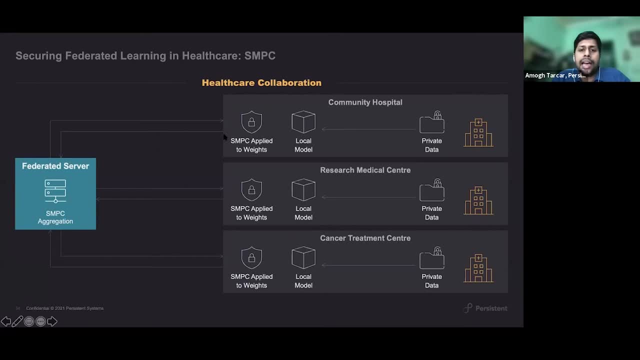 you can actually do aggregation in a very secure way and, uh, that's some. that's one way in which a edited learning can use secure multi-party computation. but again, this is something which is researched. it's not something very common, but it can happen and open mind and with the 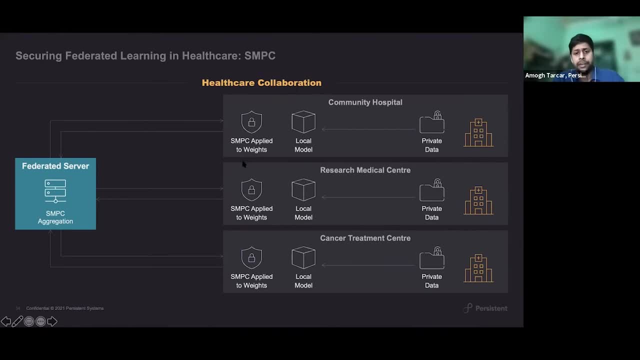 pytorch implementations are really trying to get this and it's very interesting to kind of go through and read how exactly they kind of build this. so they had to go reinvent very specific things like activation functions which work in a multi-party settings. but that's applied for 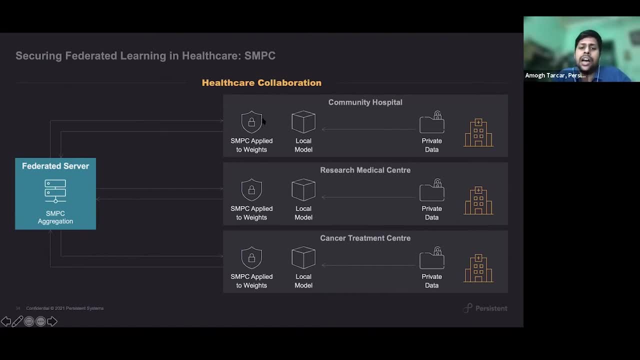 machine learning and such, but just for matrix multiplication as we are seeing here, all they kind of need to do is that they need to get these weight matrices to fix precision so that they can split it very nicely between multiple parties and try to do the computation together with all. 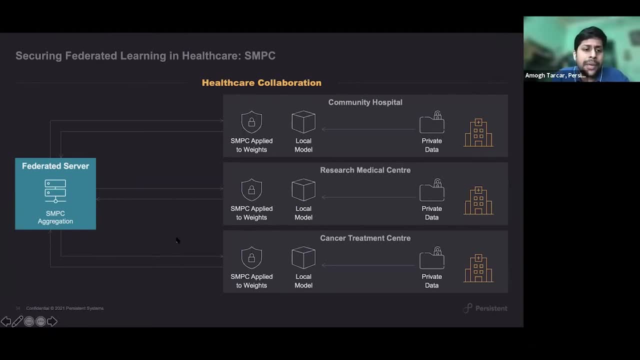 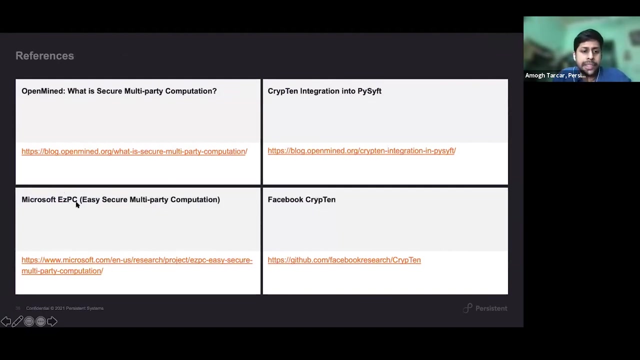 these three parties. so it's it's kind of interesting to do it that way and, as compared to homomorphic encryption, this is a sort of alternative which can serve the same purpose, and i encourage you to read more about: uh, microsoft, ez, pc, uh, this particular github. 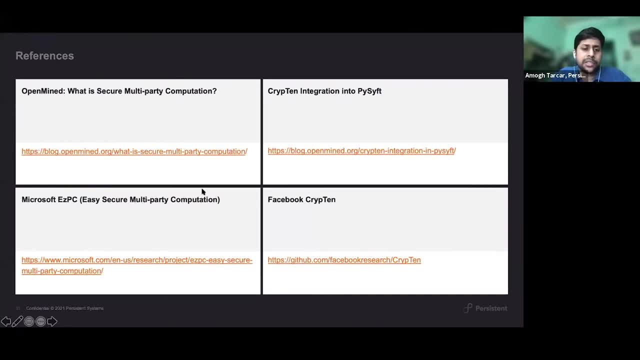 repo- it's open sourced- wherein they are working with compiler level work as well as they are working on various other protocols to actually do machine learning using multi-party computation. krypton is another library which facebook has come up to do multi-party computations and openmind also has a nice blog post on that. in interest of time, let's just 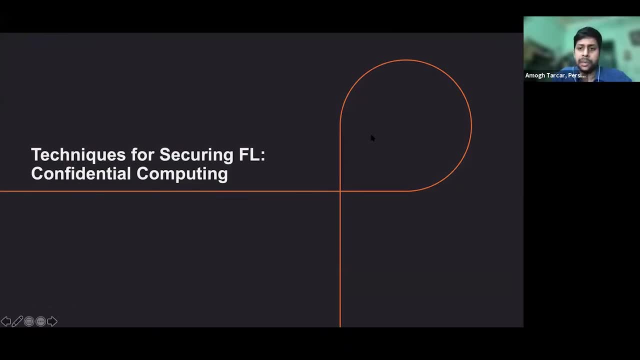 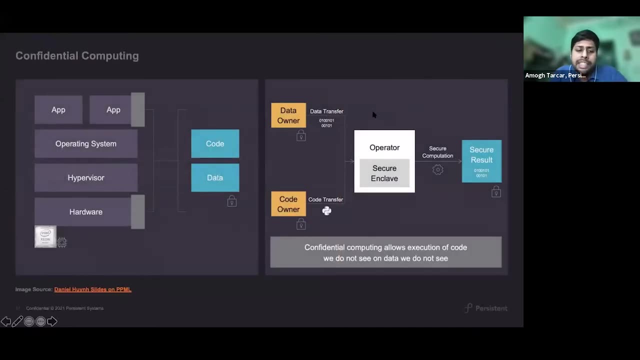 go to this final technique, which is confidential computing, and once that is done, we can, you know, maybe take questions. so, uh, so so far, what we have seen is that we were trying to use cryptography, we were trying to use- uh, we were trying to basically use all these encryption techniques to kind of. 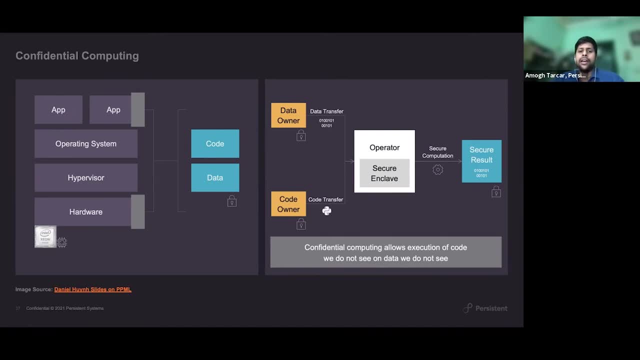 make sure that you know the data is kept private. there's another scenario wherein the trust factor comes in, and the trust factor basically is talking about integrity of the code or actually doing a lot of execution in the desired way and making sure that it the whatever code you wrote exactly. 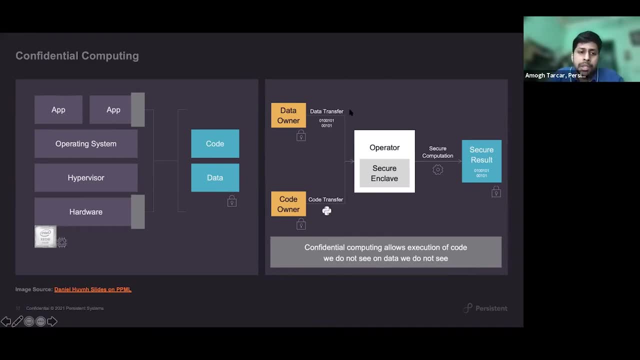 the same way it was implemented and that gives you lots of trust guarantees, as we saw. so, uh, you know, just to build context, what usually happens, uh in in normal machine learning as well, is that if suppose you're using a remote server to do any sort of computation, uh, in that server your 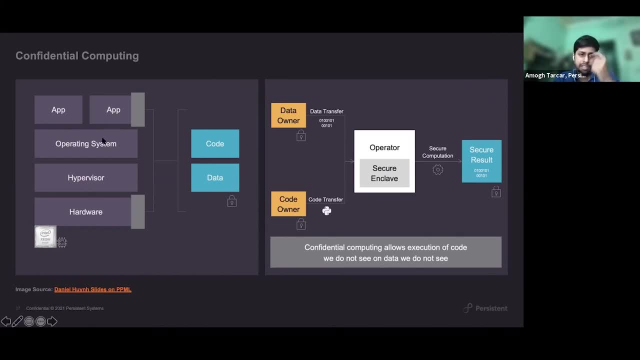 application is running. but whatever your data is, it's visible to the operating system and the hypervisor and actual hardware. this particular you know operations are going on. so if suppose there are system level you know attacks which happen on this kind of you know systems, you are at risk to kind of the data which 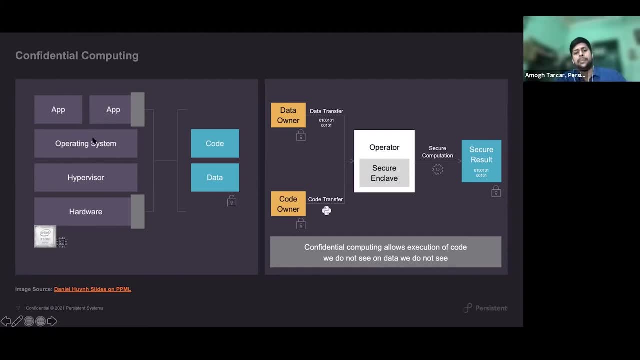 is there which is actually getting operated upon is, even if it is encrypted and sent to this particular operation, when actually doing this operation it is kind of decrypted. it's in that form present at this kind of, you know, hardware levels. so what intel actually worked with is that they. 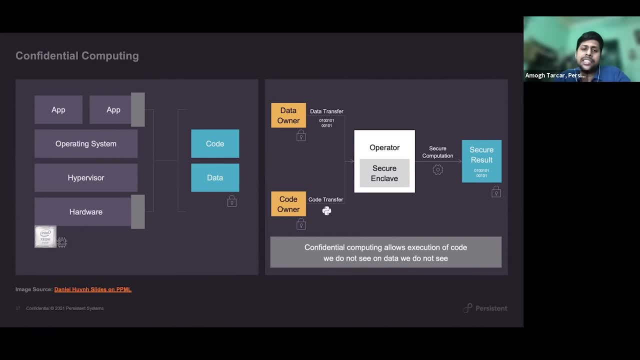 developed something called a secure enclaves, which are actually regions in their chip which are completely isolated and they basically allow you to. they basically do this direct connection between your app and they allow you to direct. you know, they give you a secure memory space inside the 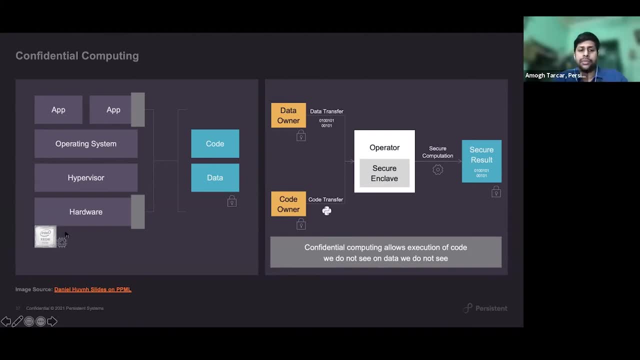 processor itself to do your computation. and uh, with that, with that secure enclave, your, your compute basically, is kind of uh safe and it's not really visible easily to this uh other actors on the same machine and with that what happens is that you and the other thing 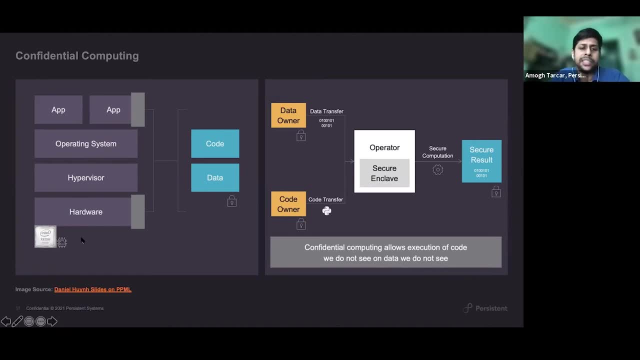 which- which, uh, intel does- is that they have a test station service which, basically, every time you run a particular code in that enclave, they generate an attestation, kind of an execution certificate, which can guarantee that the execution worked exactly like the way you code it. so with, with, 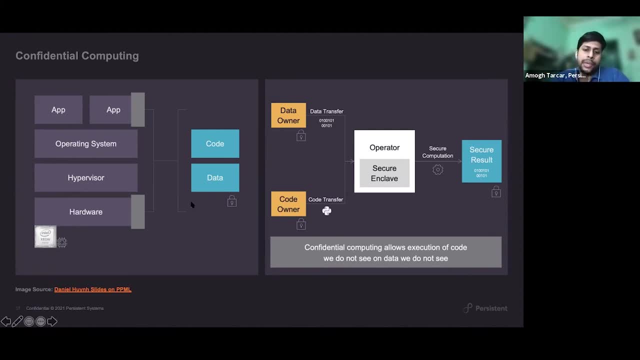 that basically you you get a very powerful tool for doing very secure kind of operations inside this secure enclaves and, uh, to actually expand it further, what they have also done is that they have introduced protocols which say that this is a hardware area in the micropos, in in the processor. 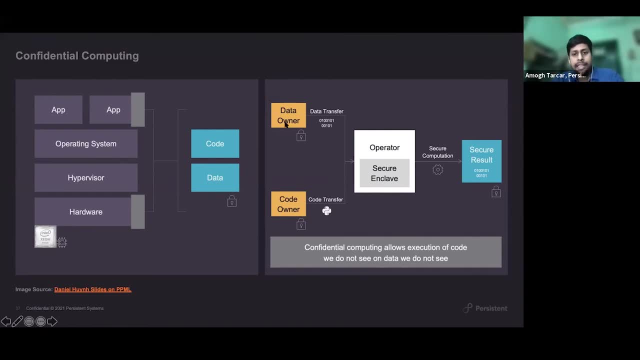 itself right, and what they have actually devised is that they have some encryption schemes. uh, these are usually, you know, symmetric or asymmetric encryption schemes wherein the data owner can just send that data inside the enclave in an encrypted format. so your data as such is sent encrypted. so none of these you know network or the operating. 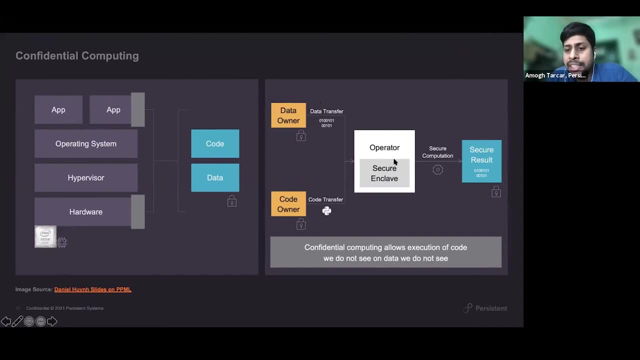 system. nobody sees that data but it straight away appears inside the secular and play where you can keep that private key and decrypt it. on the other side your code basically can also be in the same way completely encrypted, can come inside or say if you have a machine learning model. 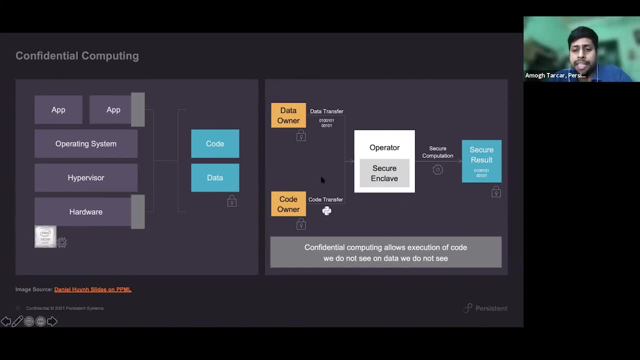 then the machine learning model can stay encrypted when it is outside this enclave, but when it goes into the enclave it can be decrypted and inside the enclave then you can actually do the operation between this code and this data. so, uh, common operations are actually of inference, which is: 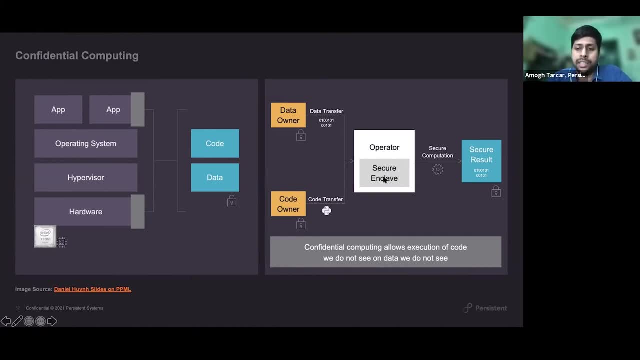 like this model is loaded here. this data is brought in, you do the, you do the prediction. the predicted result is again uh can be sent back in encrypted format to data owner. so there are multiple advantages of using confidential computing or actual hardware backed secular enclaves to do this execution and that gives you very 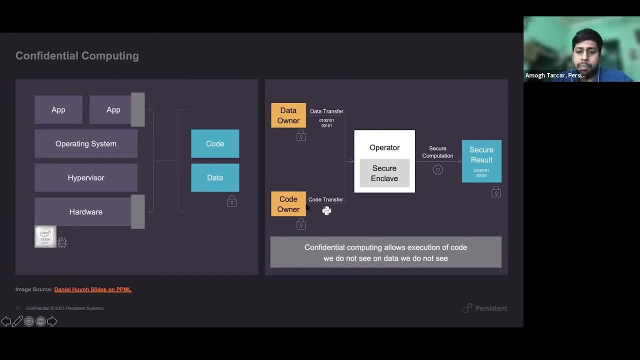 good guarantees that your data is kept private and at the same time, you know you can actually do operations in this security, but it's hardware backed. you need to find that specific. you know types of intel processors which have, uh, which have that sort of secure enclave. and then you 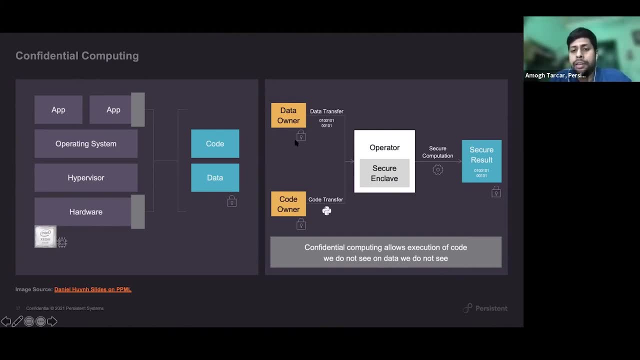 have to also code this whole platform on basically saying, uh, you know, your data has to arrive in that encrypted format and it has to be decrypted only inside secure enclaves, and so on. and so intel has actually worked on like c plus plus libraries for exposing, uh, the you know, the. 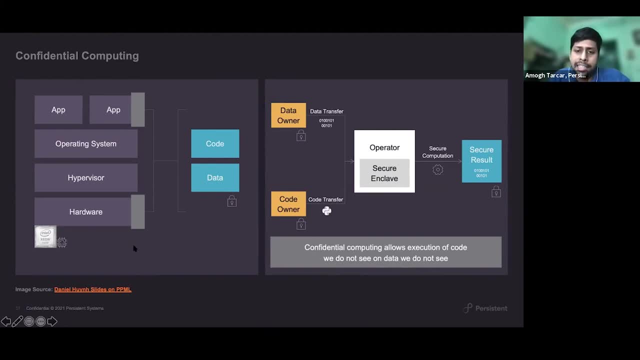 programming interfaces for doing it. they call it intel sgx and over sgx. then there are, like it's, c plus plus, but then, uh, because c plus plus is kind of a little bit more tricky for people to widely adopt, uh, there are other players as well who are trying to help with that. uh, there is a project. 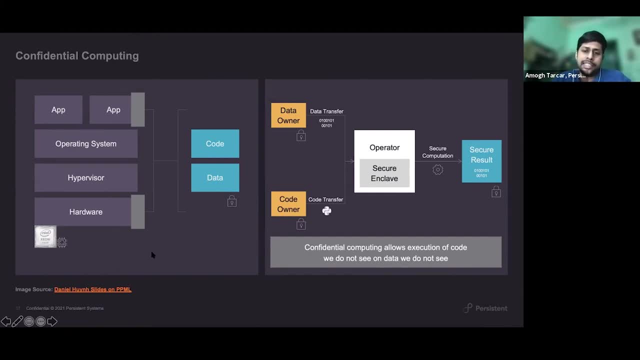 called graphene, which actually allows you to run a docker container inside this enclave, or, you know, they basically manage how exactly the docker container runs inside, but again, the docker container is not running the full version of everything. it has to be kind of thought about. uh, as we see, you know it, this, it's a hardware area, so you need to so that particular you know. 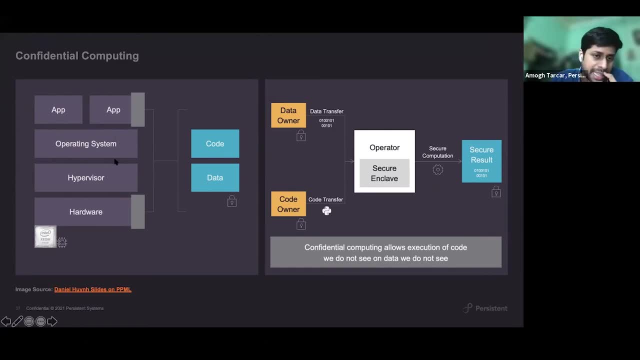 you have to think about various operating system components which you'll use and all that. so graphene is a very interesting project which is trying to do that on a parallel line. r3, which is a blockchain technology leader, is also working on that, and the docker container is a very interesting project which is 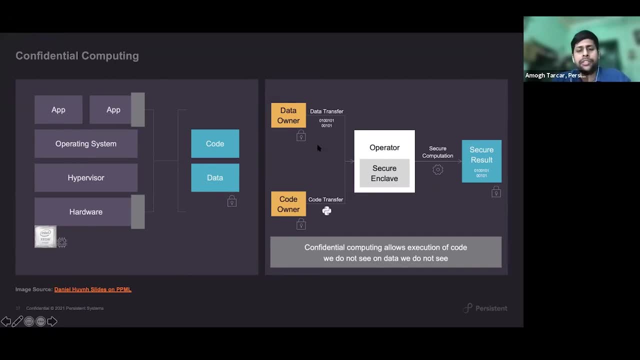 uh, running on a parallel line and they have invested into this and they have made their own docker implementation of doing that and what they have put inside the docker is a java runtime kind of operations and this java runtimes allows you to suppose you can do this setup in java. then 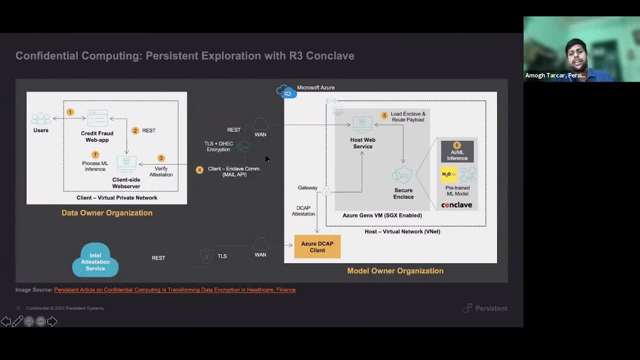 you can actually do modern inferencing in java, and so persistent has been exploring this and working on this, and we recently had written an article about how to do confidential computing in in a real world setting. so we have basically built it over this conclave, which is uh made by r3 and 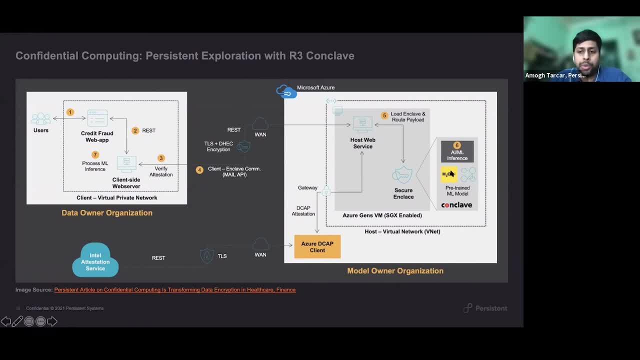 what we put inside that concrete was an h2o model, so that model basically is inside that conclave. so that is what we are really trying to protect and the data basically from. say, in this particular example it was about credit card fraud detection, so it's like this particular end user wants to. 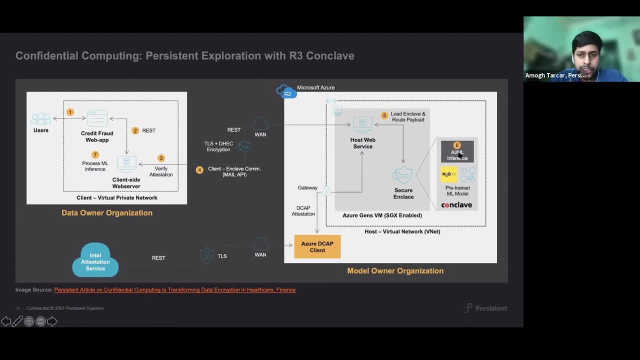 get the prediction from this model. but this model is also made to be protected. so if you run a normal machine learning service and you just send this data and print text to this service, probably the service can make a copy of that data or, you know, do something like that and the other. 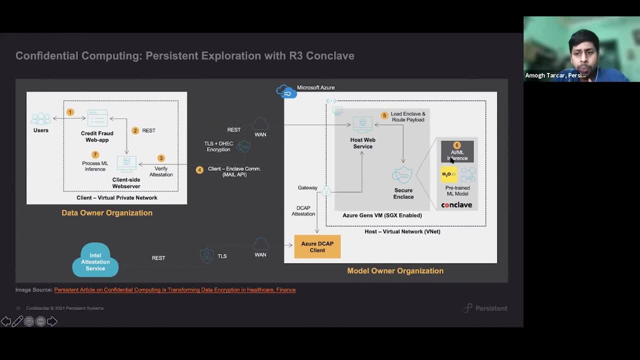 side, in case we have, uh, this model, if it is directly shipped to this users, then again there is a risk. it's a model which we want to protect. so this setup basically helps in in getting there. so you have this model which is nicely sitting inside the conclave. 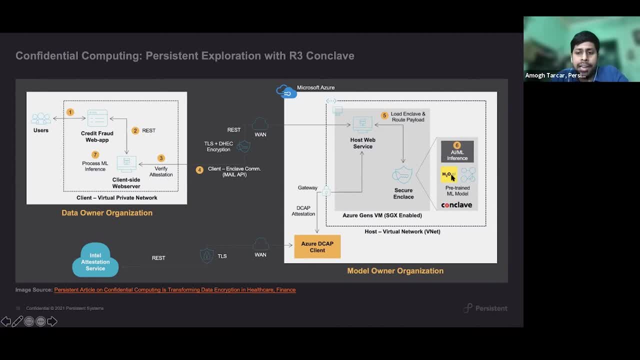 your data comes encrypted all the way inside the enclave where it actually can do the operation of doing the prediction, and then that result is then sent back to the client. so in that case the the service did not learn anything about that particular data point, but it still ran the. 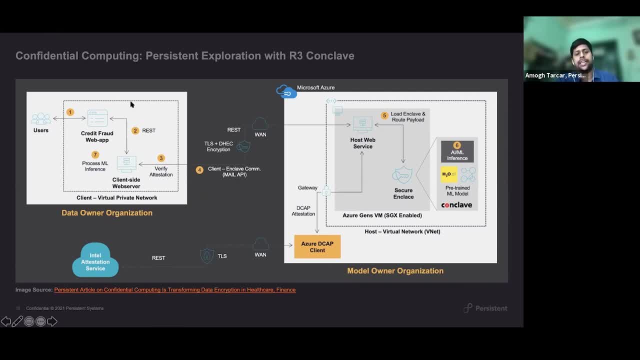 prediction and the. the data owners are also happy because the data was protected. they got the result as well, and uh. so one thing which was kind of interesting over here is that you want to still trust that this operation was successfully. like you know, it did not do anything. 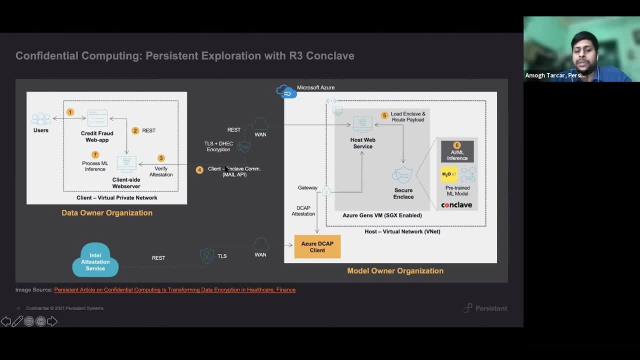 different from, uh, what was told- or which was basically what was discussed earlier- that what they will do is that they'll take this data inside your secure space. they will just run the model and give you back the prediction. so nothing else supposed to happen inside secure enclave. 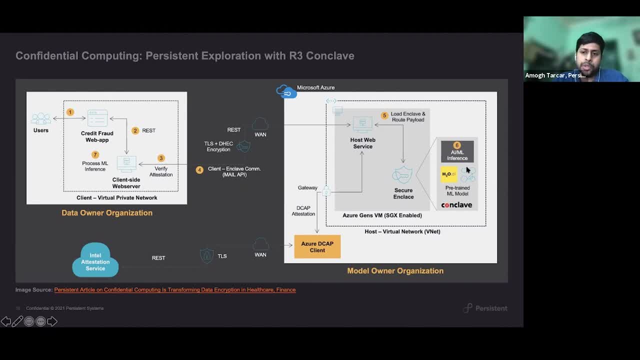 you're not supposed to make copies of that data, you're not supposed to do any sort of other operations on that data. so that sort of guarantees is what is provided by the software, this attestation service, and this attestation service says that we have checked this particular. 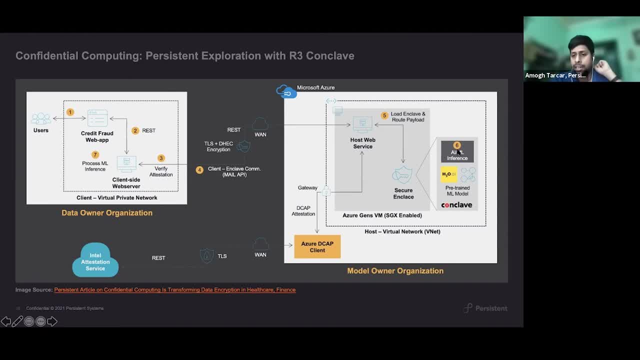 code. it does exactly what it is, and here is a certificate which says it actually operated the same way. so with that sort of guarantees, you know, there's a peace of mind for this data owner to actually, you know, get the prediction without being scared of sharing their data to this particular. 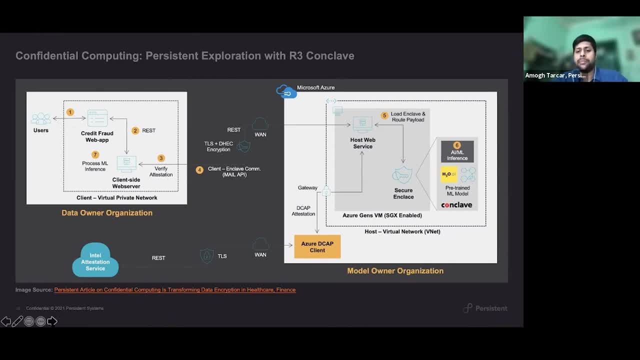 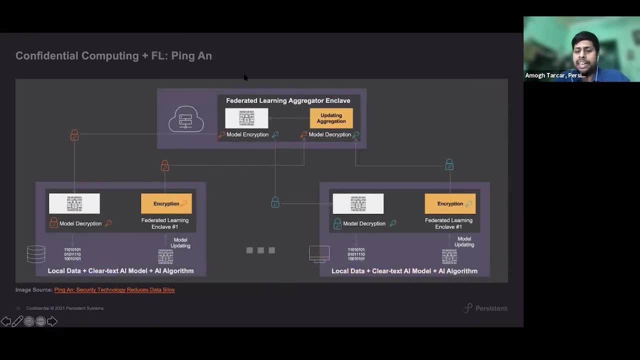 service. so that's how you know, confidential computing can be applied to machine learning in general, to federated learning. this is something of a of a very interesting research scenario, because the actual memory inside this enclave is kind of controlled by these chips, and so it's hardware. 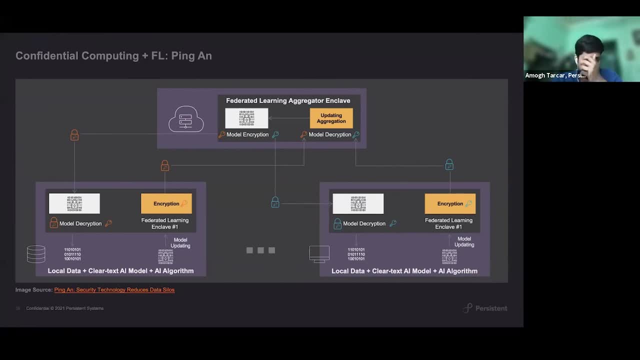 backed. so you need to be very aware of this. how much space is actually present inside that particular enclave and which? so, to give you an example, simple things like if you just want to load pandas in a secure enclave, it's very difficult. so, unless you basically you know, figure out. 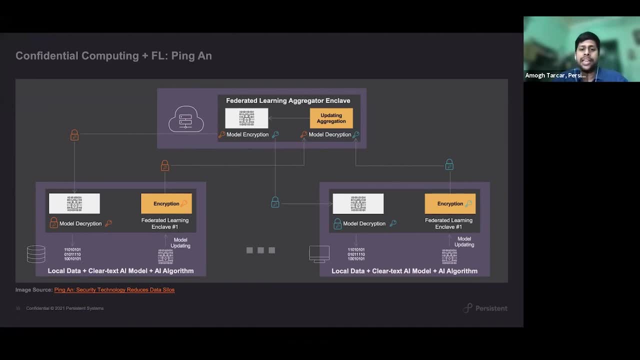 a way of actually loading python properly in the python runtime properly. just loading pandas could fill up the whole memory which could be there in this enclave. so there are some challenges, but there are. there are various companies who are actively, like ping and is one company who are actually trying to figure out if you can try to do, you like to actually do machine learning. 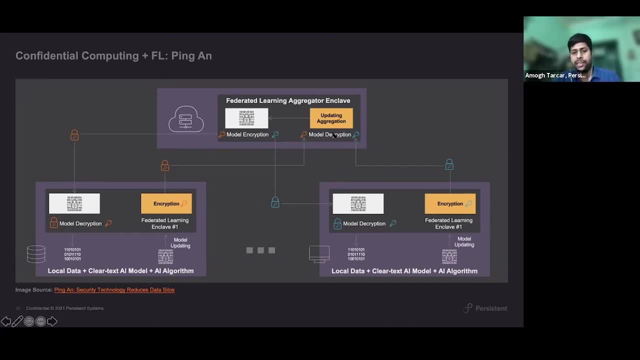 in an encrypted space and they have written about it and they have a service as well which tries to do something like this, and it's very interesting that there are some companies who are actively to see federated learning in this sort of a way, but tying it together to our case. so, basically, 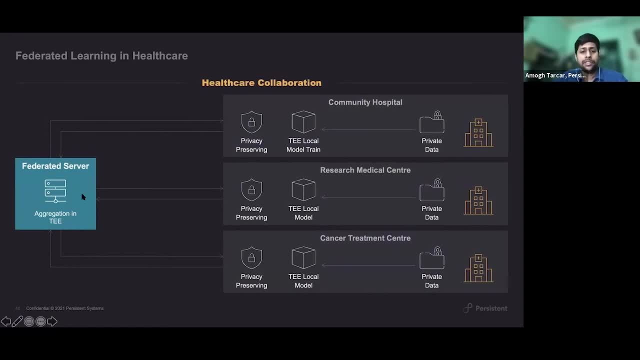 this. this can be, uh, raise concerns about. suppose we did not trust this aggregator. then whatever operations the aggregator is supposed to do, we can try to do it in a trusted setting. so the weights can be like the way the fraud detection company encrypted and sent it to the enclave straight away. 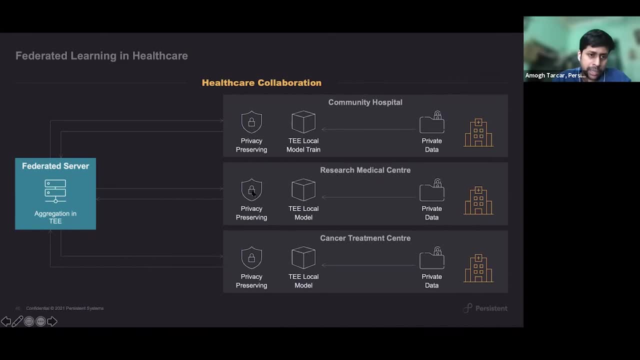 the same way, we can probably just take the model updates and send it directly inside that in a trusted execution environment and do the aggregation there, and that could solve one of the trust issues. if the aggregator is supposed to do anything else about, you know that weights, that's. 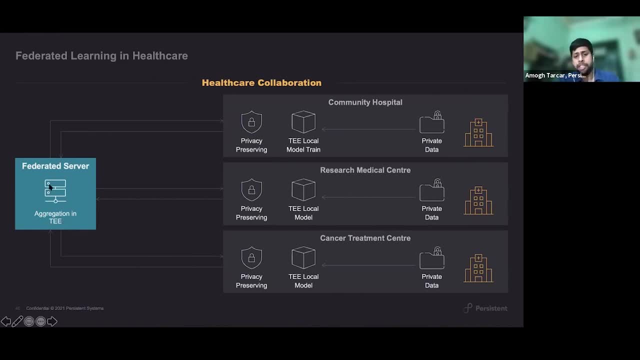 something which can be prevented by using trusted execution on the aggregation. uh, if you want to actually try to push trusted execution on the local training that i just now, as i explained, it's a little bit tricky but you can find workarounds of you know, trying to get there. 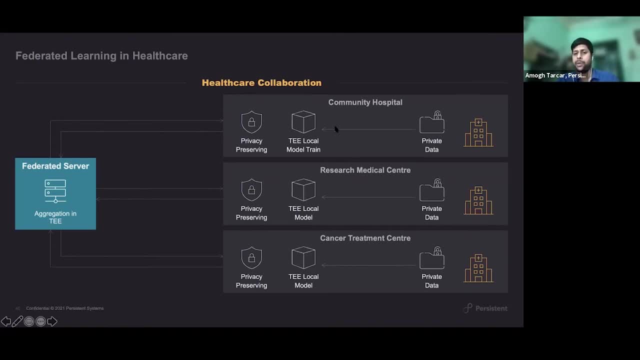 using technologies, how ping n is really exploring, or with graphene and other kind of you know approaches. but uh, it's a very interesting paradigm of trying to use hardware to kind of uh back the, to get the trust in in actually execution, so you can guarantee integrity of uh executions by using this trusted execution environments. 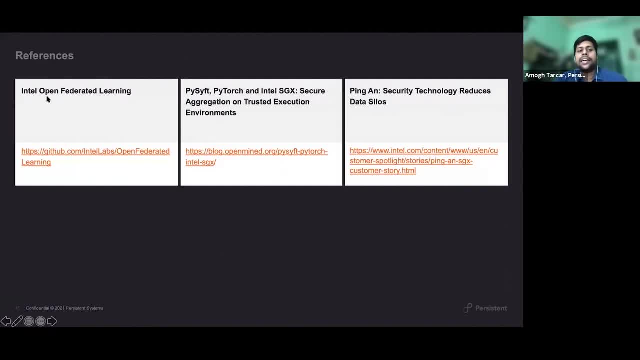 so and you know, intel has been also working with federated learning, uh across multiple universities as a part of the federated tumor segmentation initiative and they have open sourced a library called intel open federated learning which has some components which do refer to this. sgx ping n is another company which is like very heavy and federated learning using 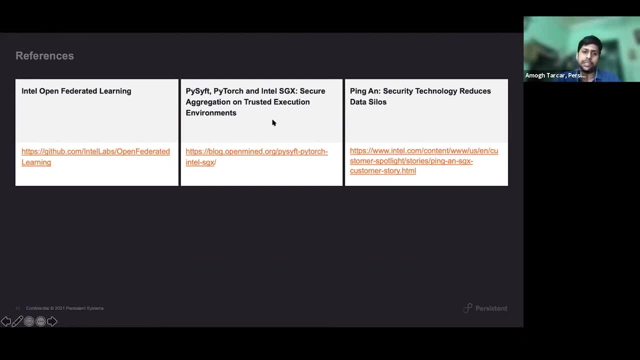 sgx for financial kind of use cases, and pytorch and pisif. they are kind of just expanding the envelope with respect to what's possible, and there are examples using graphene on on these. so yeah, that's about it and i think we have just five minutes left. so 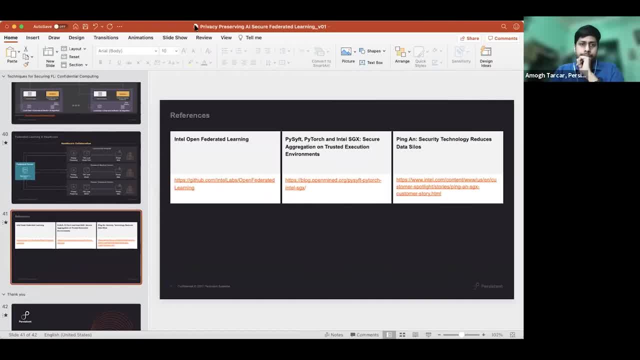 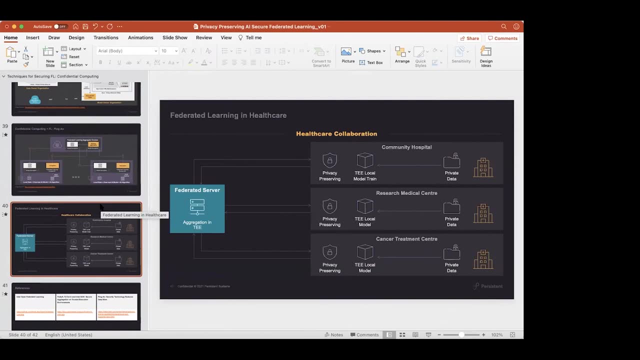 i can take some questions about this. uh, hi, hi, i'm, it's renal here. yeah, so the last, uh, last topic which we have discussed in terms, uh, in it's related to the pong that we we are actually doing is federated learning server, or is it being the operational shape or like? 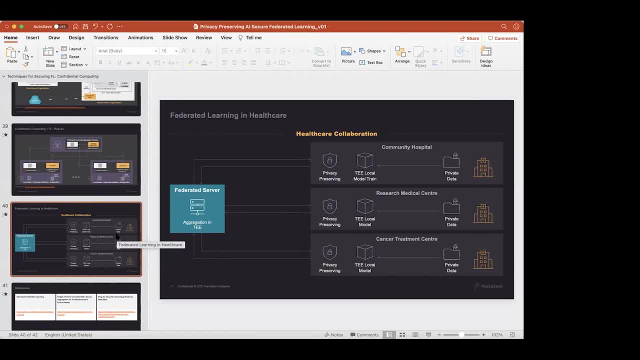 a federated learning in that actually it's like a bigger challenge in itself, or it is, it's the research area it's going on or it's done. actually, that's what my question is. so, yeah, it's a very good question. so partially some problems have been solved. like if we try to see federated learning. 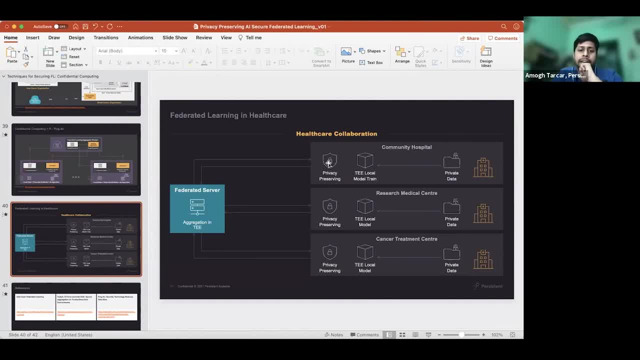 server. what it's trying to do is that it is trying to just aggregate some matrices and uh case. you know you do, you can do it in a and java backed. but there are some enclaves like colda actually have java blacked, uh, java backed kind of services which allow you to do this matrix. 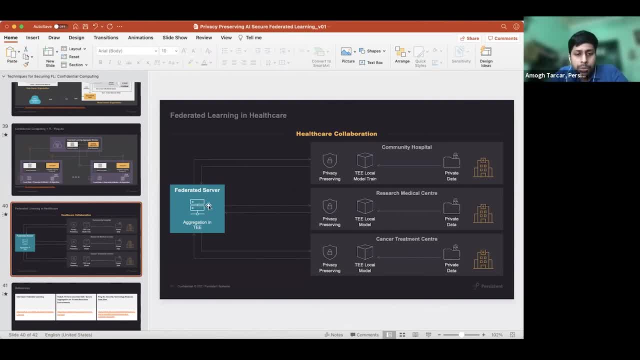 operations. uh, so that's something which can be used for doing it, and some you know partially it has been already done as well, but the the bigger picture of you know, as you know you might recollect, like i had, i put a slide which says you know there is a state of the technology. 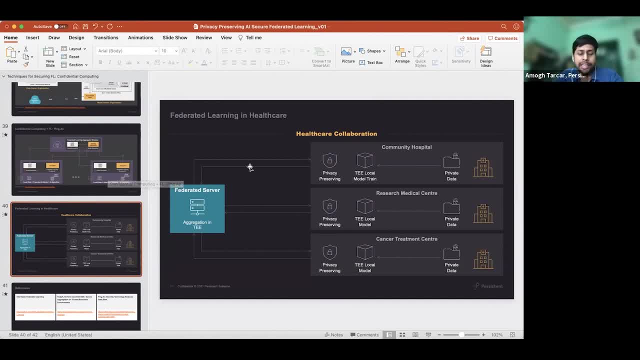 where it has been used and how it applies to federated learning. so, with respect to machine learning, it's something which is still uh in active research, like there are multiple implementations. uh, there's some. some people have been actually able to do it, uh, in some specific you know constraints and so on, and uh, in some cases it actually has been, you know. 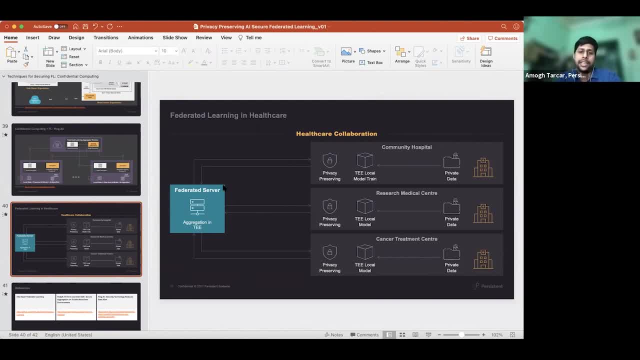 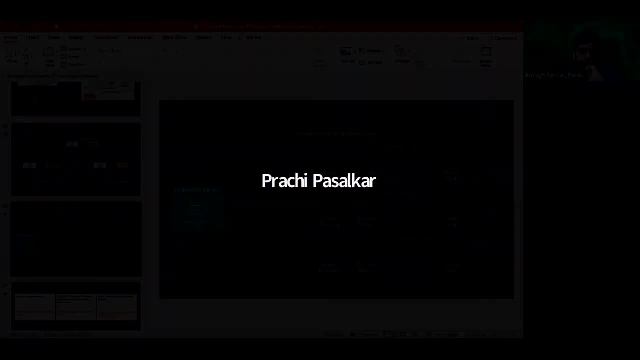 possible, like, like the way we could load a model for inferencing. uh, in that case, in the same kind of, you know, using the same kind of options, we can also do a federated learning or that uh, aggregation inside this particular trusted environments. okay, actually, i'll just take one question, which is: 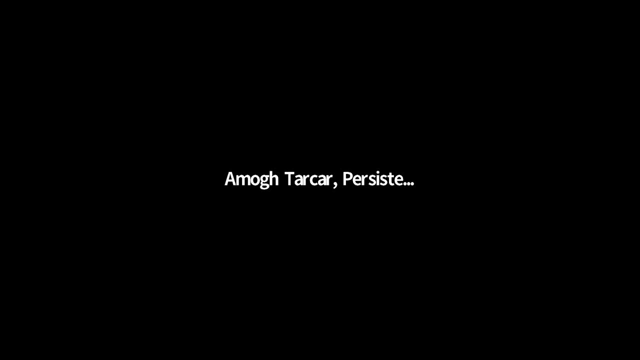 from dr sham about uh azure confidential compute. so, uh, dr sham, the way we have tried to do it is actually using uh colda's conclave and uh, what we have, uh, you know what we have in our experience. what we have done is that we have worked with h2o. 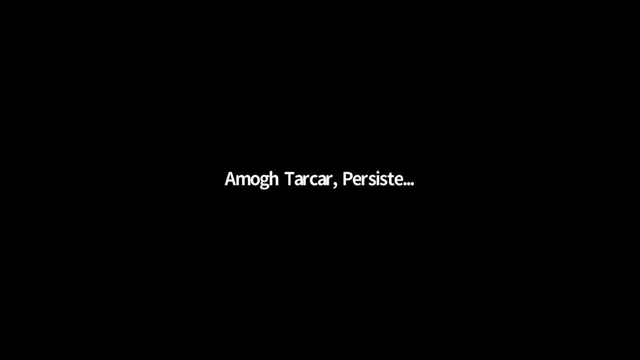 libraries and, using the java backed implementations, we could load the model for model inferencing and, uh, we could, we could do that. so we have to be more aware of what sort of ram and all those like not exactly ram, but memory areas which are actually allocated on this. 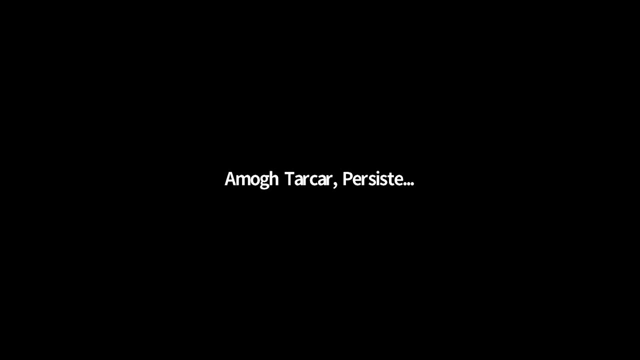 but trusted executions is actually much more larger topic and i would encourage you to read more about it. uh, it's for, like anything, big data, uh, it's kind of still it's sort of in research. uh, mainly because of the, the limitations of, you know, memory inside trusted executions. but 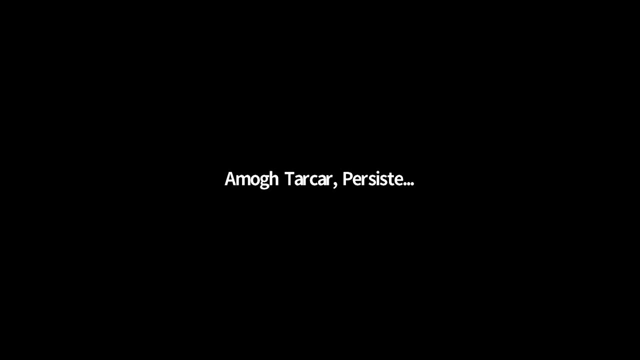 actively. there are multiple solutions uh being applied to overcome that. thanks everyone.